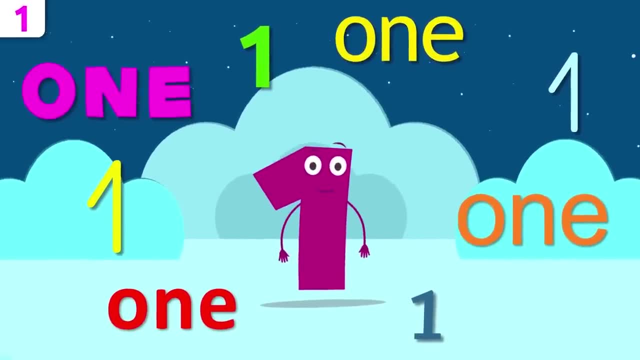 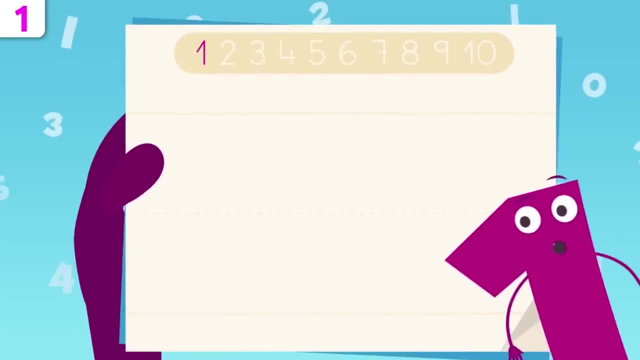 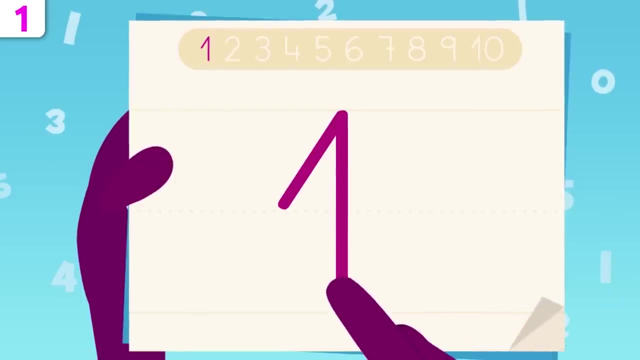 One. That's it. Did you know that number one is super easy to write? Pay attention, We start right there and we go all the way up here. Now we trace down to this point. That's it. You've just traced number one. 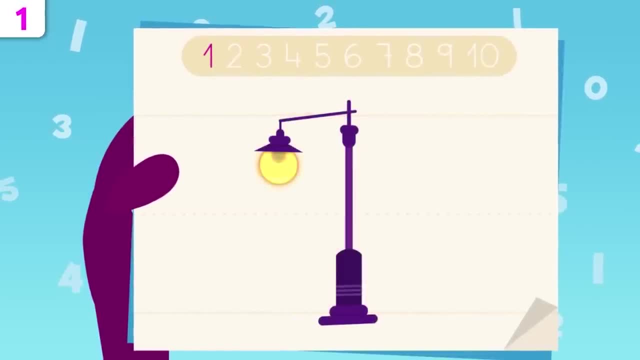 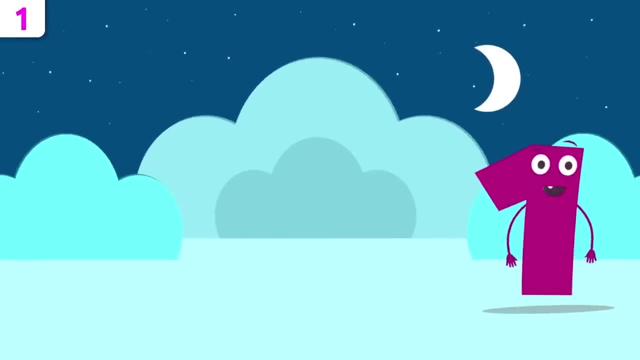 That was easy, wasn't it? Look, I look like a street lamp. Try it at home using some paper and a pencil. Now I'm going to give you some examples. Let's see How many candles are on this cake. 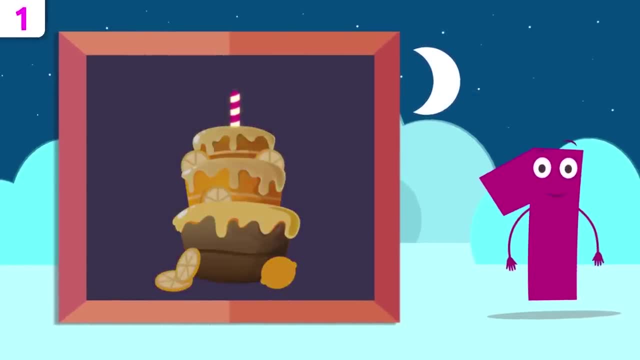 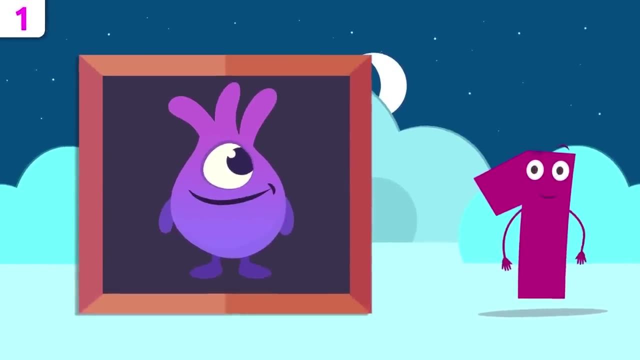 Easy peasy. There's just one Happy birthday. Happy birthday. Look how cute that alien is. How many eyes has he got? He's got one eye. See you later, alien, and we could sing a bit. What do you say? 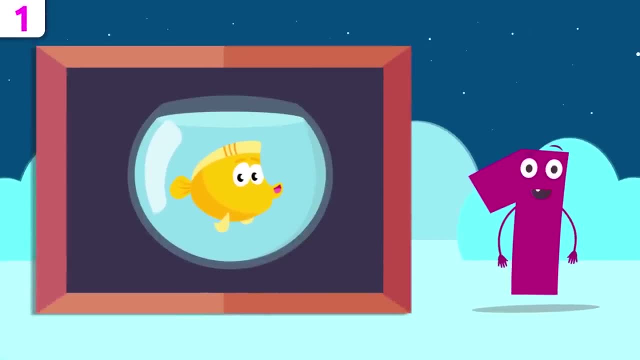 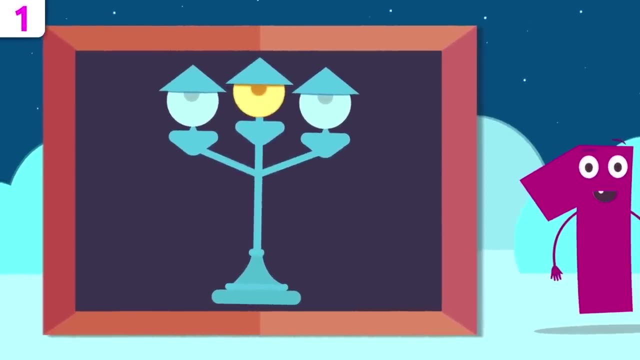 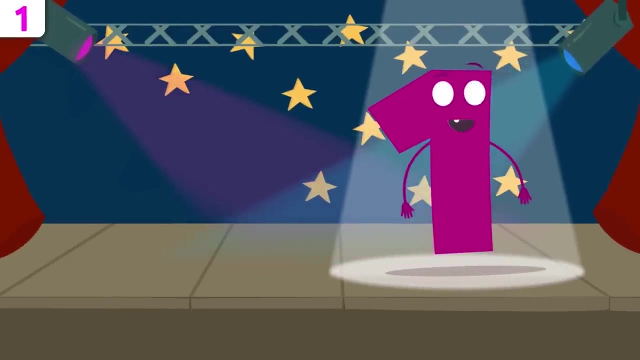 How many fish are there? Let's see There's one fish. Will you figure out this one? How many light bulbs are on? Let's see There's one Way to go. Hey, What if we liven things up a little with a song? 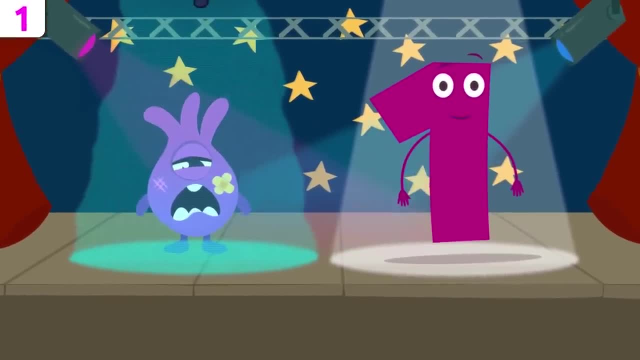 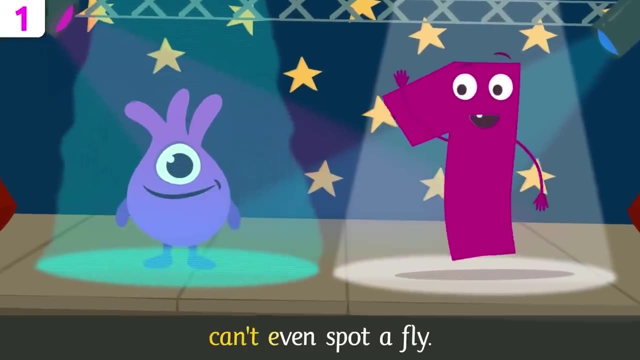 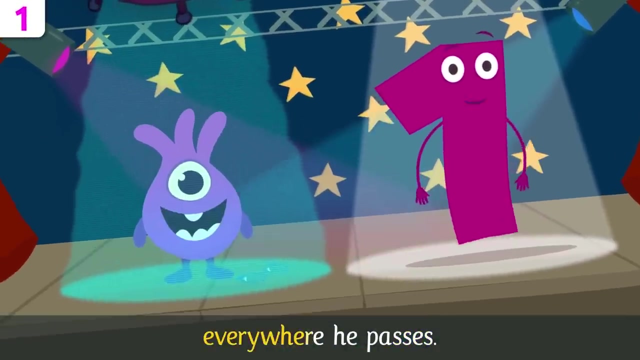 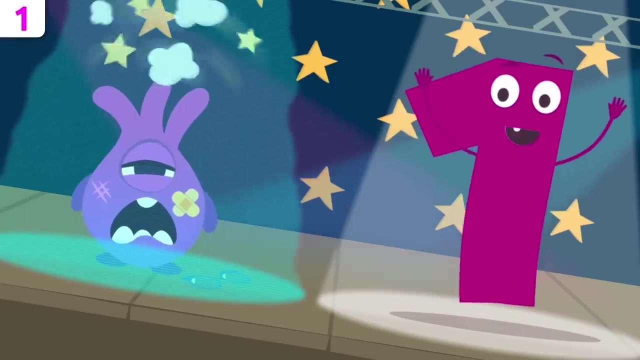 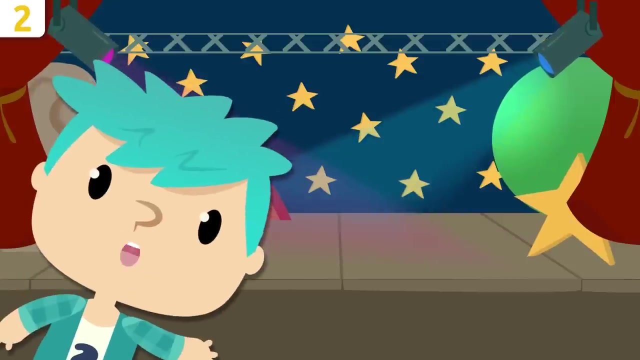 Will you sing along alien M話, filled with so many other fish. A little alien with one eye Can't even spot a fly. He's looking for glasses everywhere He passes by. How are you friends? Would you like to keep on learning the numbers? 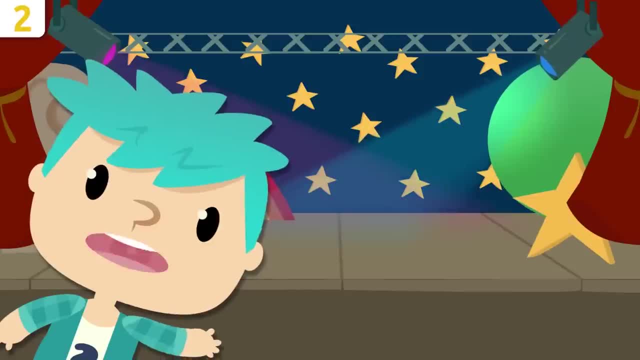 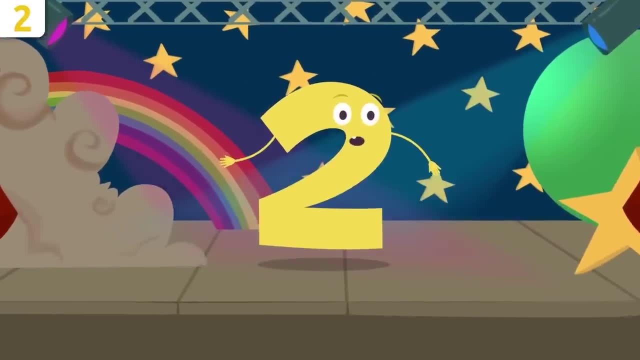 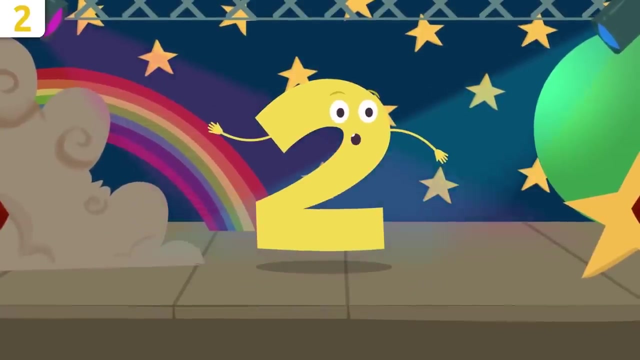 Today I'm going to introduce to you my friend number two. Hello, How are you doing, my little friends? Do you know which number I am? I'm a really cool number, Number two. I'm going to tell you a few things about myself. 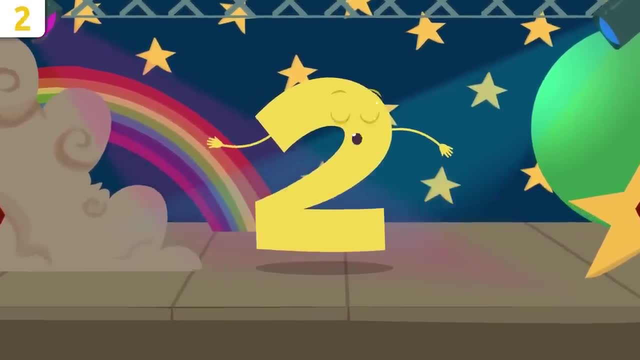 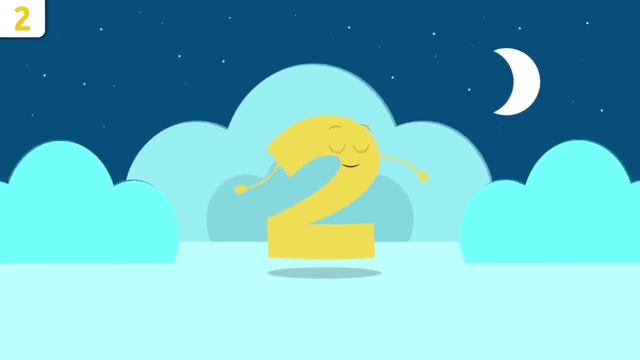 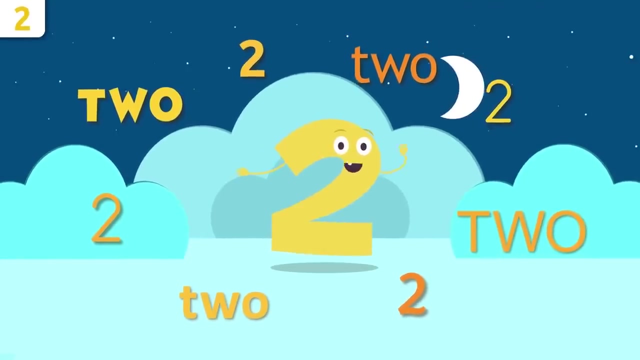 Would you like to learn about them together? Remember, we'll be singing a song in the end. You can't miss it. Do you remember my name? Come on, repeat after me. Two, Two, Can't hear you Louder. 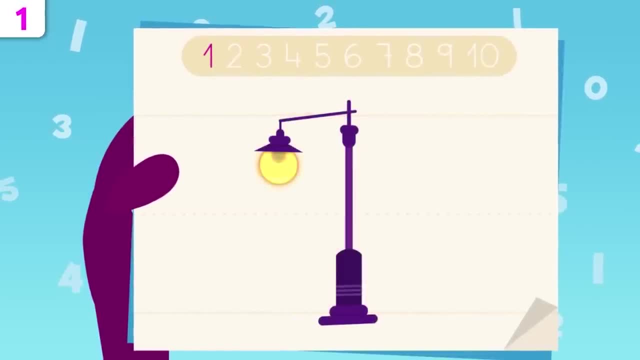 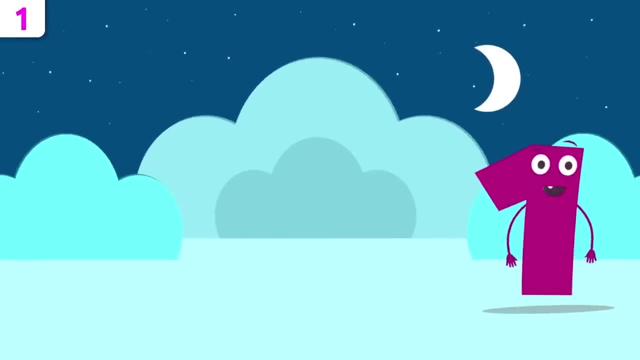 That was easy, wasn't it? Look, I look like a street lamp. Try it at home using some paper and a pencil. Now I'm going to give you some examples. Let's see How many candles are on this cake. 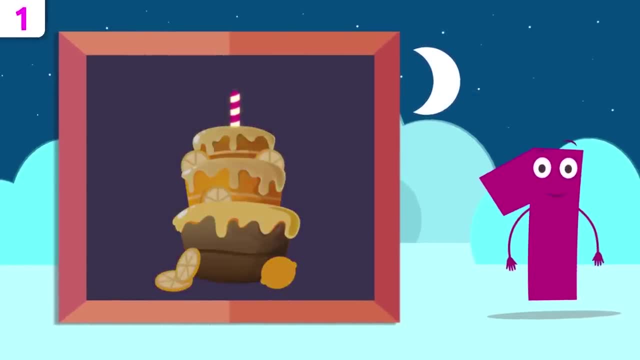 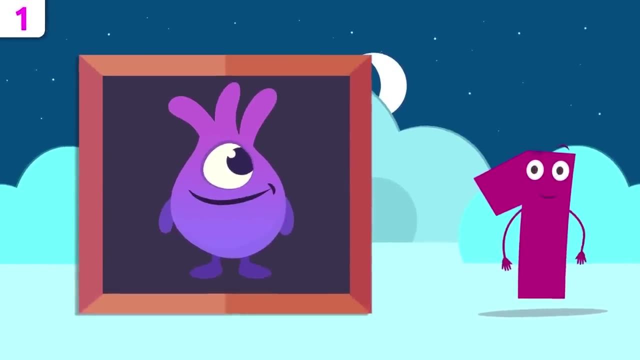 Easy peasy. There's just one Happy birthday. Happy birthday. Look how cute that alien is. How many eyes has he got? He's got one eye. See you later, alien, and we could sing a bit. What do you say? 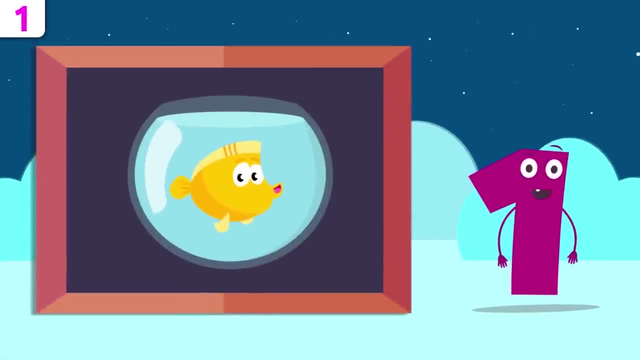 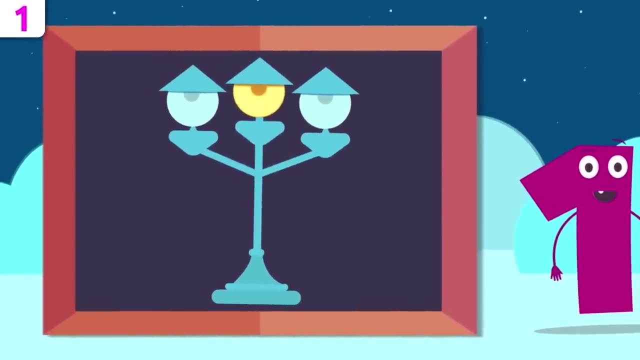 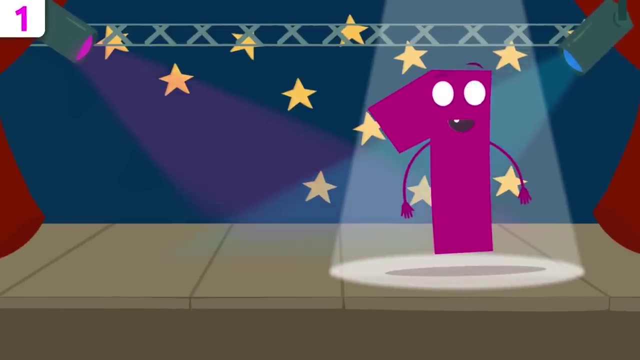 How many fish are there? Let's see There's one fish. Will you figure out this one? How many light bulbs are on? Let's see There's one Way to go. Hey, what if we liven things up a little with a song? 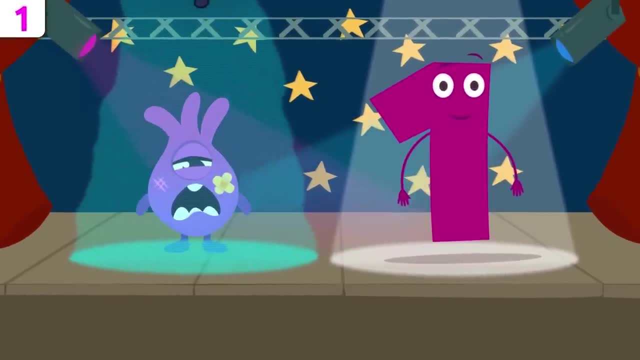 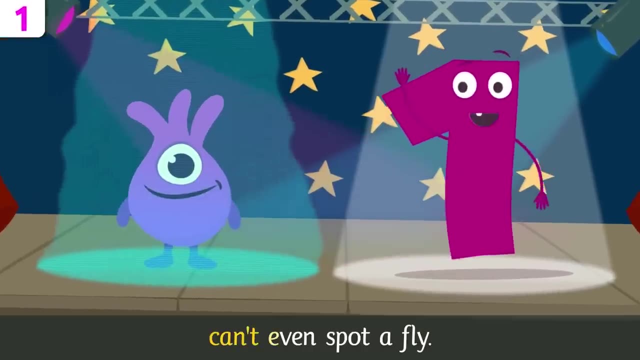 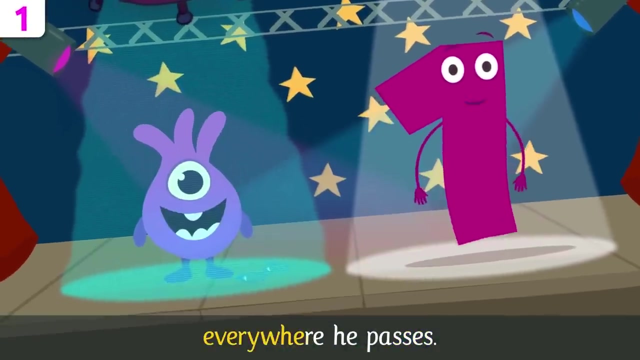 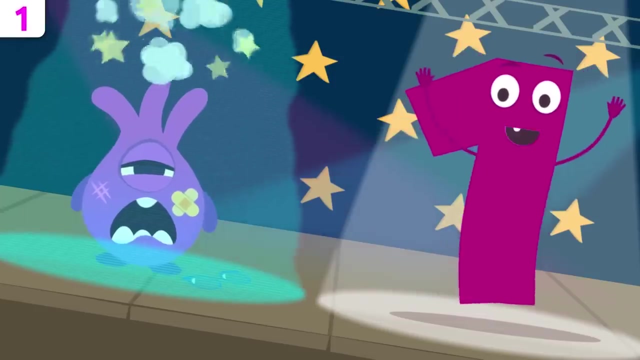 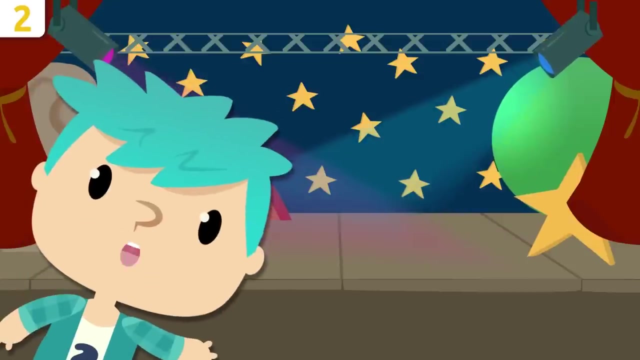 Will you sing along? alien, Yes, Little alien with one eye Can't even spot a fly. He's looking for glasses Everywhere he passes. Oh, How are you friends? Would you like to see us? you like to keep on learning the numbers? today, I'm going to introduce to you my 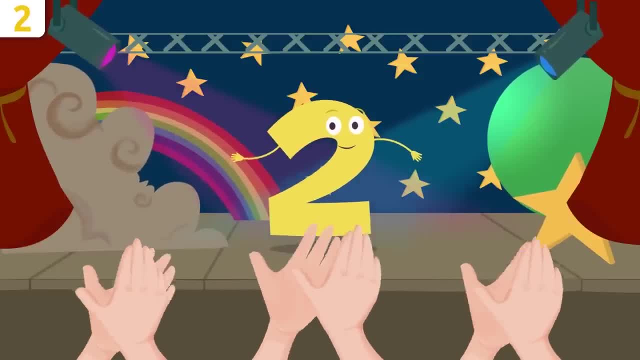 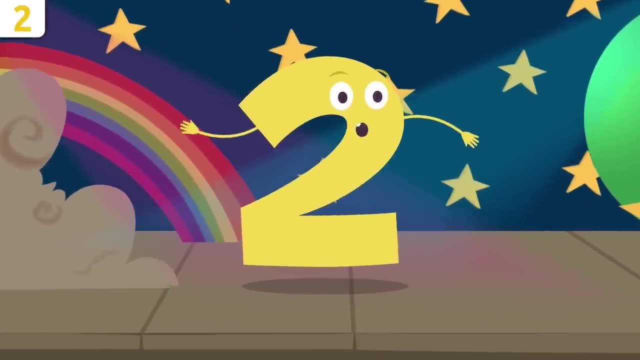 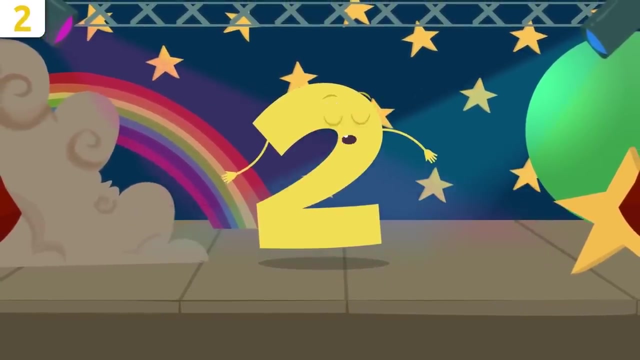 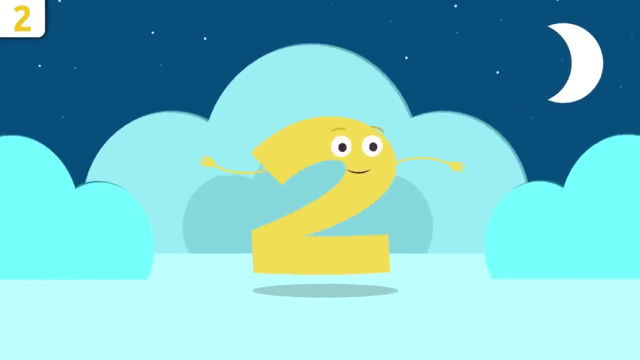 friend number two: hello, how are you doing, my little friends? do you know which number I am? I'm a really cool number. number two. I'm going to tell you a few things about myself. would you like to learn about them together? remember we'll be singing a song in the end. you can't miss it. do you remember my name? 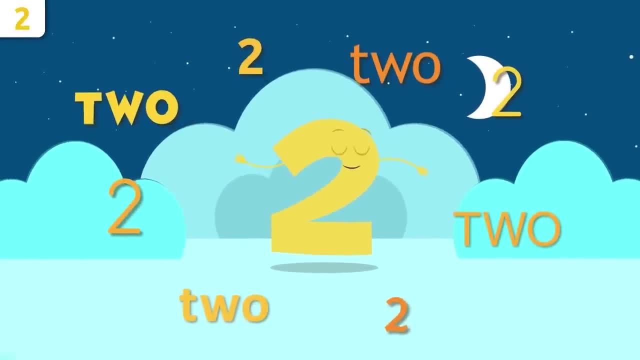 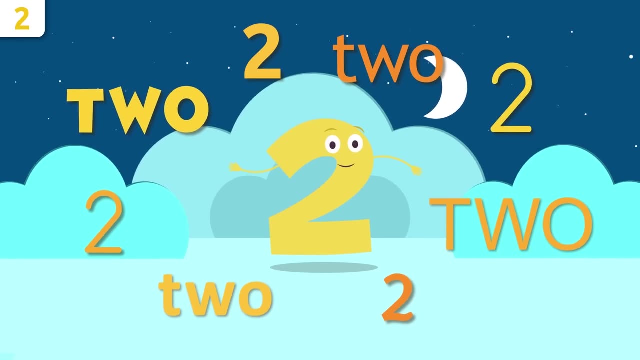 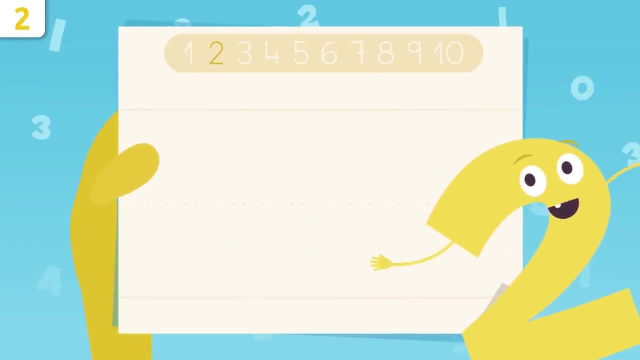 come on repeat after me to to- can't hear you louder- to wait to go. what would you say if I taught you how to write number two? we start right here and we make a curve, we trace it down and then draw a sleeping line. that's it. 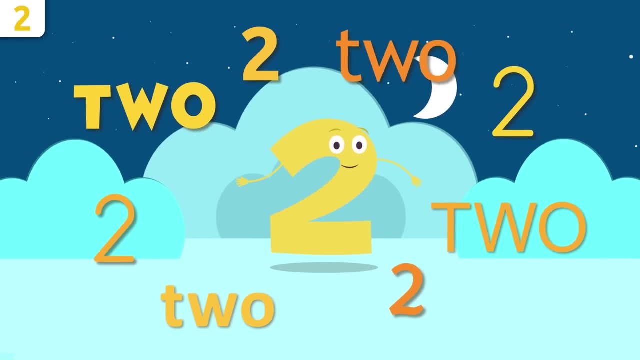 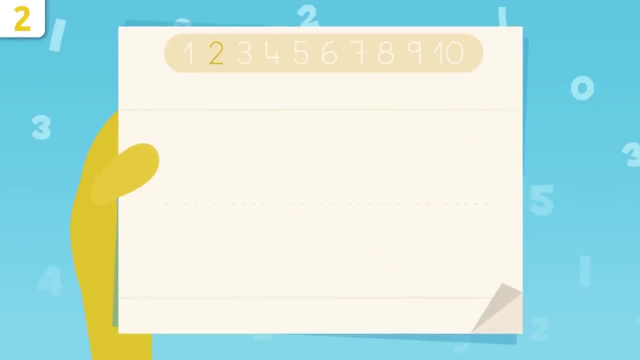 Two Way to go. What would you say if I taught you how to write number two? We start right here and we make a curve, We trace it down and then draw a sleeping line. That's it Easy, right? See, I look like a swan. 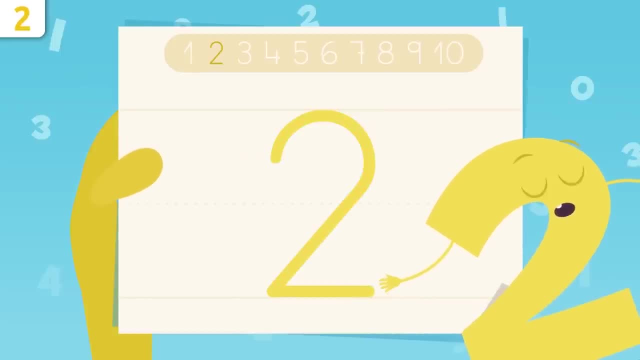 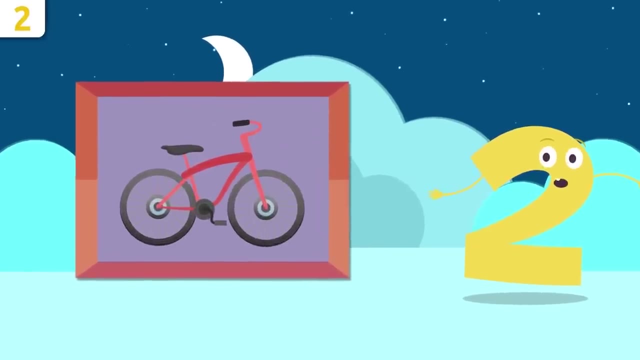 Try it at home using some paper and a pencil. It's super easy. Now I'll give you some examples. I love this bike. Do you know how many wheels there are on the bike? Let's count them: One, two. 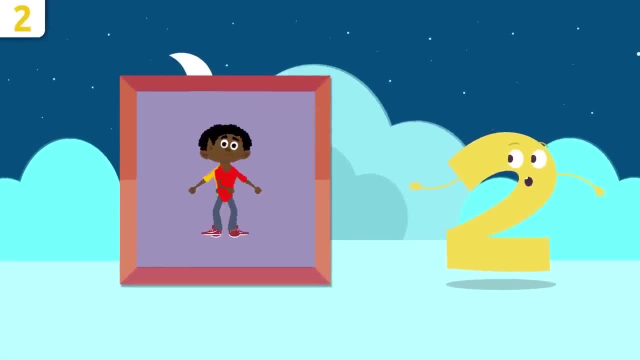 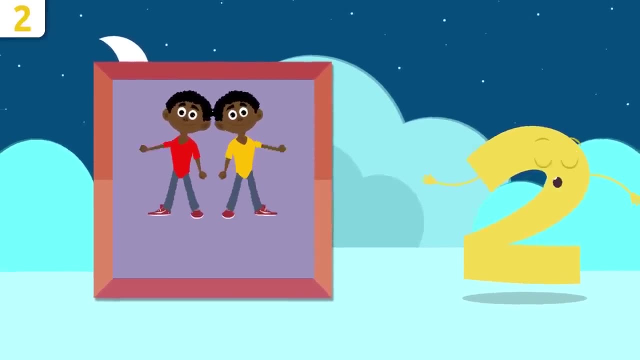 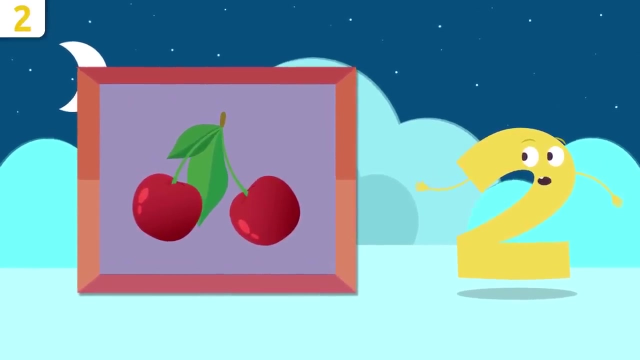 There are two wheels on the bike. Look at those twins. They're identical. How many children are there? One And two? There are two. Let's do some singing. What do you say? These cherries look so yummy. How many are there? 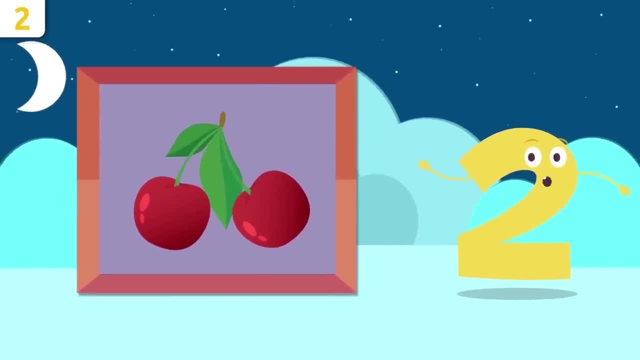 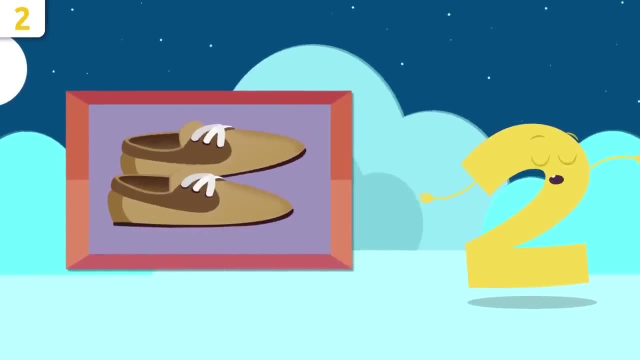 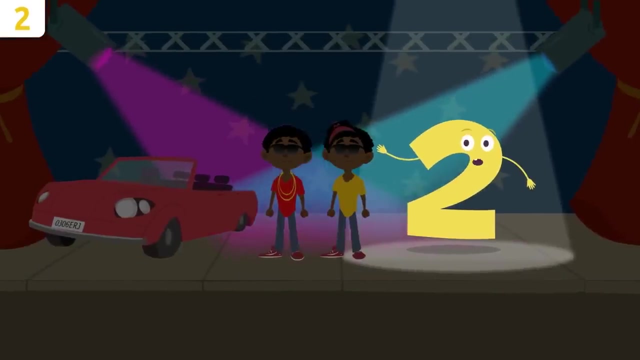 Let's see One and two. There are two cherries. What about these shoes? How many do you see? Count with me. One and two. There are two shoes. Awesome, I feel like singing. What about you, little twins? 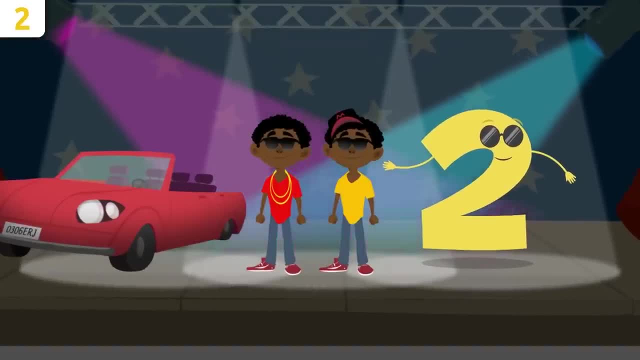 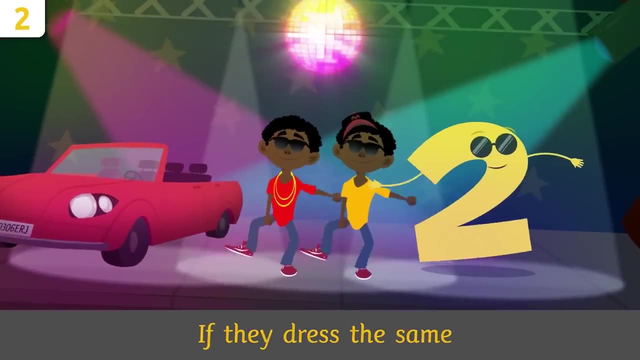 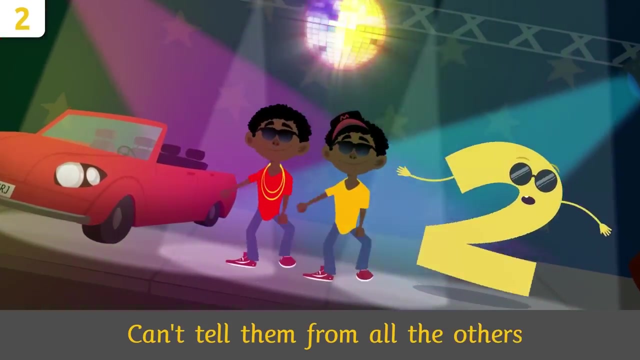 Will you sing with me? One and two. Two twin brothers- Can't tell from all the others. If they dress the same, You won't even know their name. Two twin brothers Can't tell from all the others. If they dressed the same, You won't even know their name. 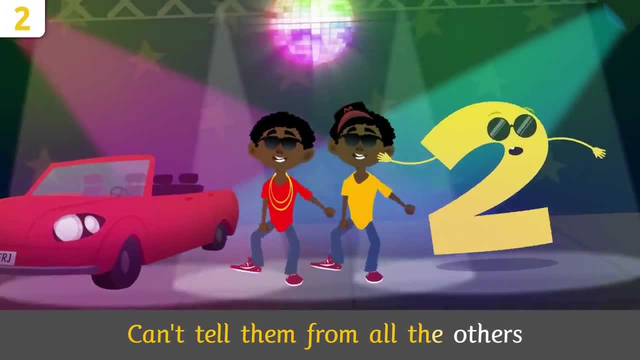 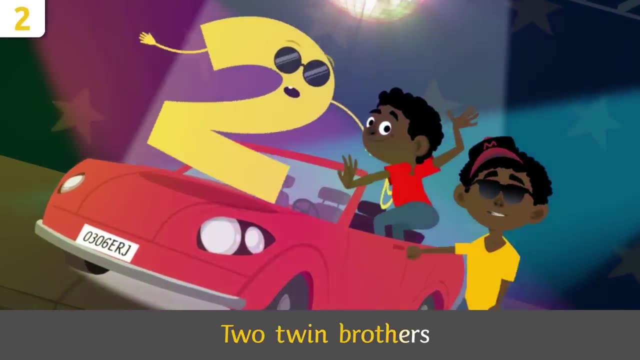 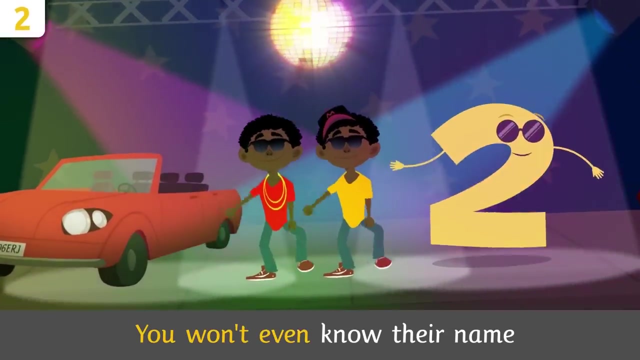 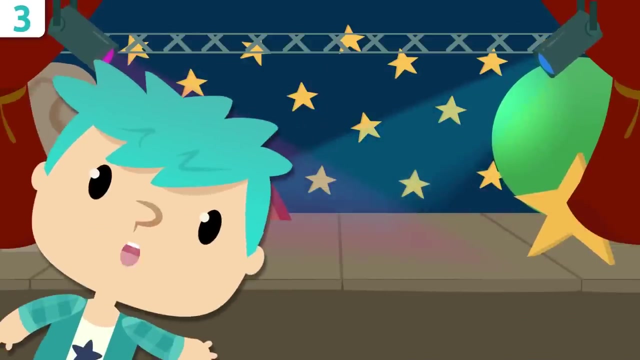 Two twin brothers Can't tell from all the others. If they dress the same, you won't even know their name. Two twin brothers can't tell them from all the others. If they dress the same, you won't even know their name. Hello there, How are you friends? 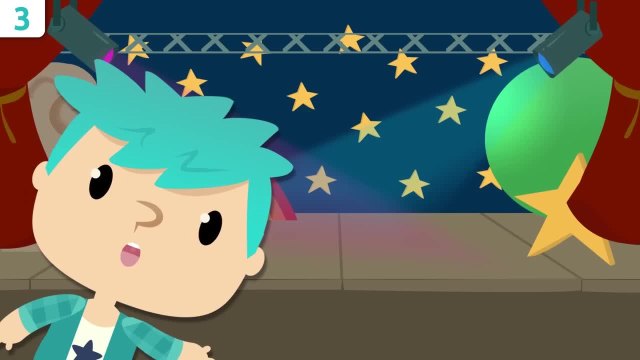 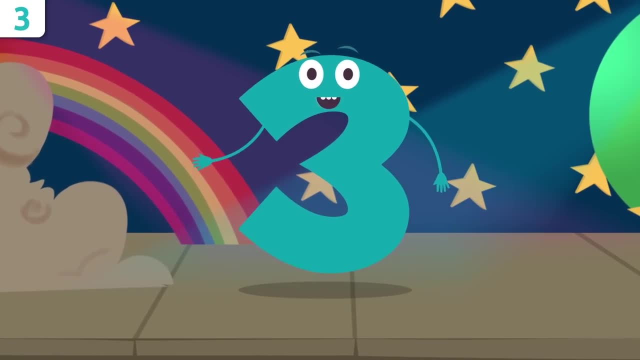 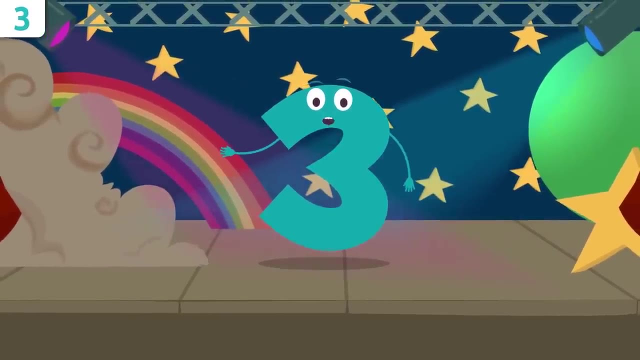 Ready to learn a new number? Today, I'll be introducing you to number three. That's right, that's me, Number three, the most beautiful number of all. Why is that? Because I say so. I'm here to tell you all about me. What do you say? We're gonna have a great time. 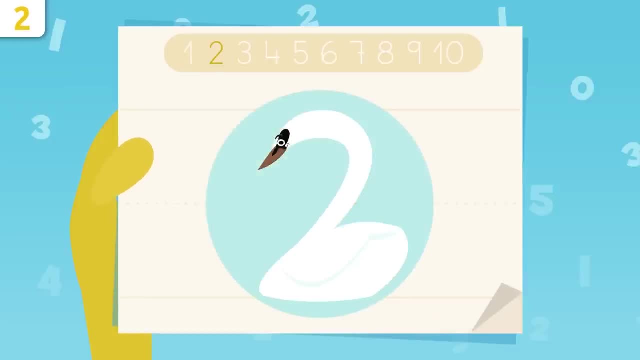 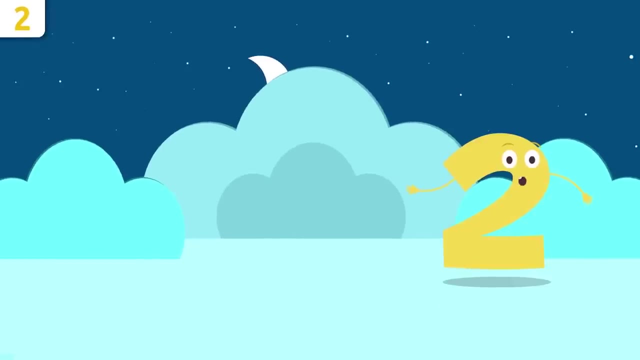 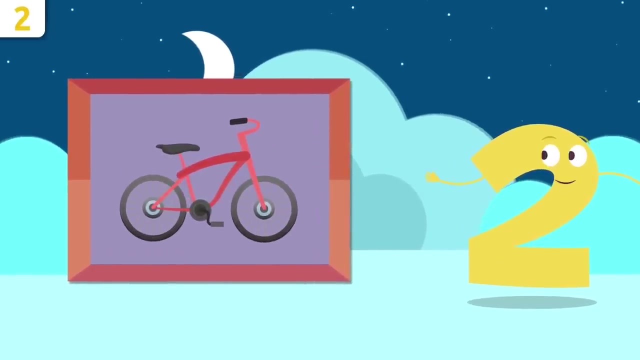 easy right? see, I look like a Swan. tried at home using some paper and a pencil. it's super easy. now I'll give you some examples. i love this bike. do you know how many wheels are on the bike? let's count them one, two. there are two wheels on the bike. 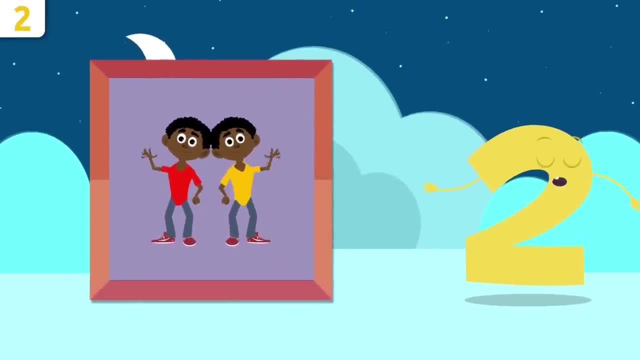 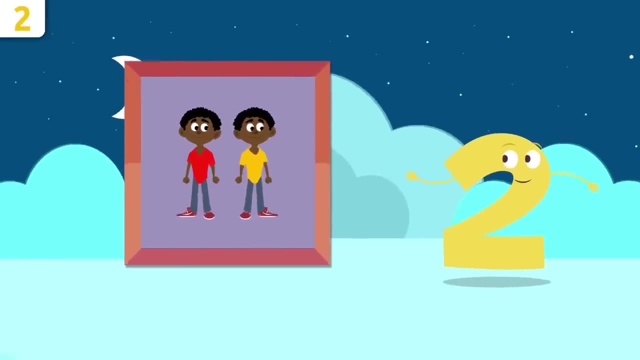 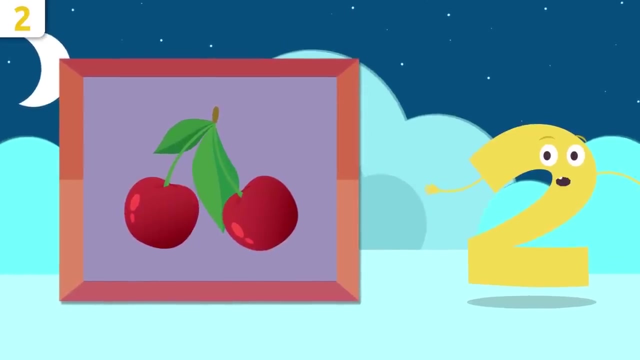 look at those twins: They're identical. How many children are there? One and two. There are two. Let's do some singing. What do you say? These cherries look so yummy. How many are there? Let's see One and two. 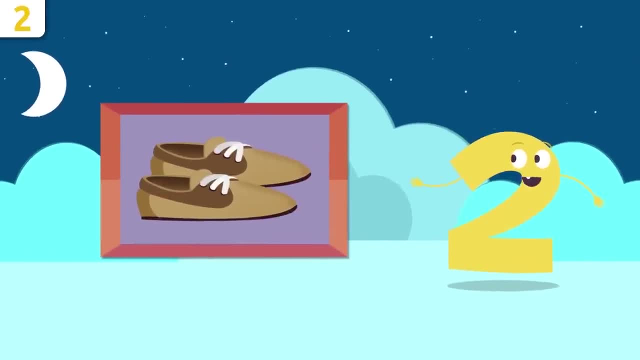 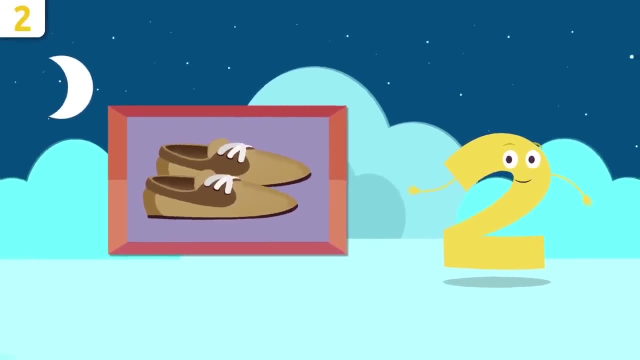 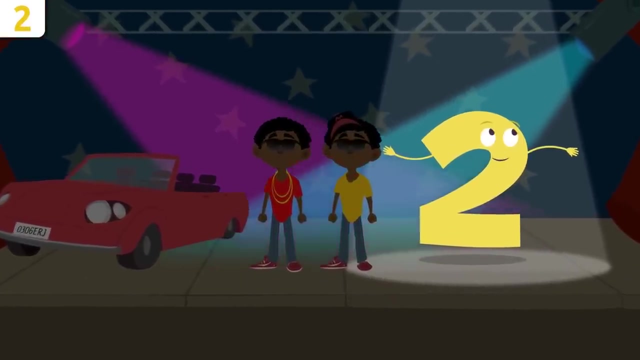 There are two cherries. What about these shoes? How many do you see? Count with me? One and two. There are two shoes. Awesome, I feel like singing. What about you, little twins? Will you sing with me? Two twin brothers. 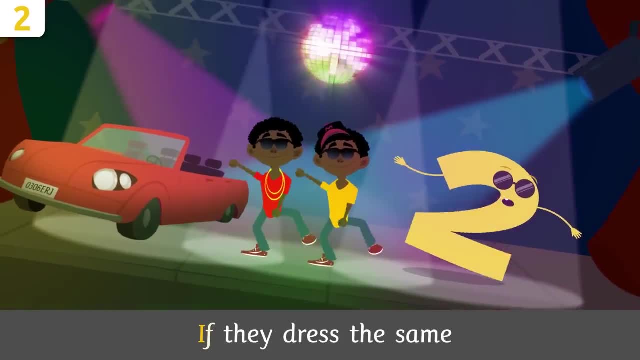 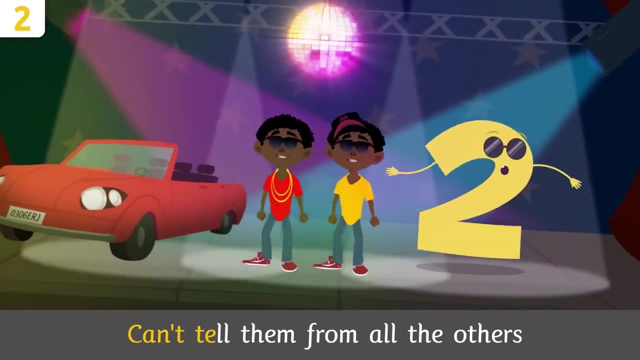 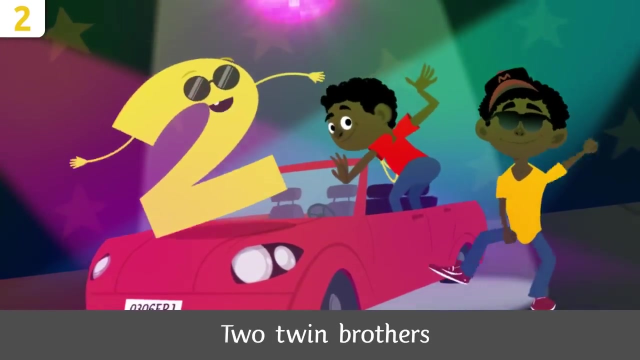 Can't tell them from all the others. If they dress the same, You won't even know their name. Two twin brothers Can't tell them from all the others. If they dress the same, You won't even know their name. Two twin brothers Can't tell them from all the others. 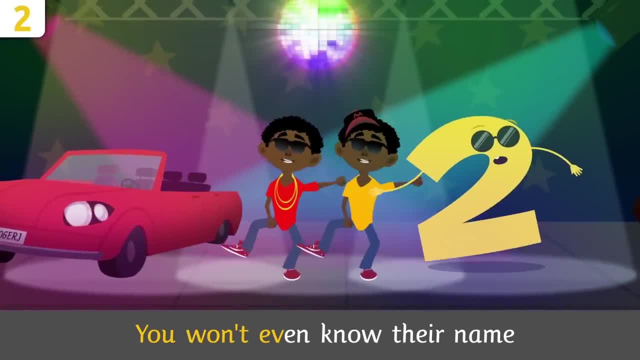 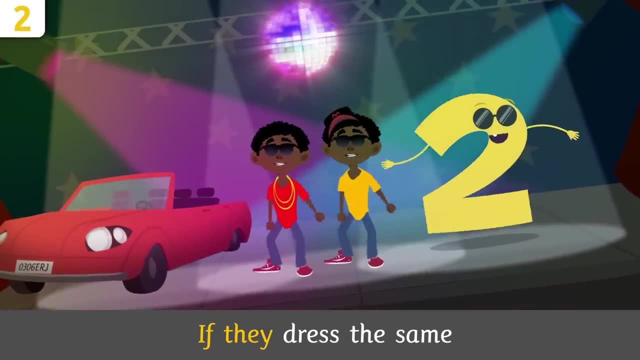 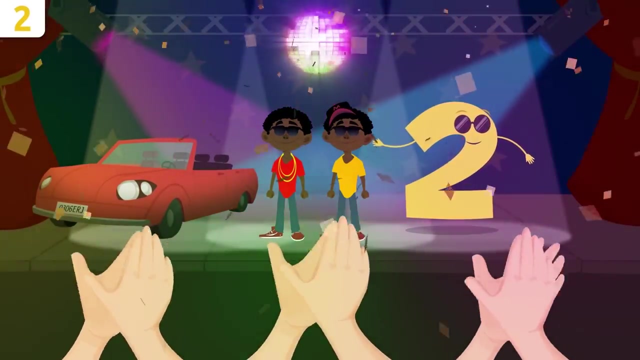 If they dress the same, You won't even know their name. Two twin brothers Can't tell them from all the others. If they dress the same, You won't even know their name. Hello there, How are you, friends, Ready to learn a new number? 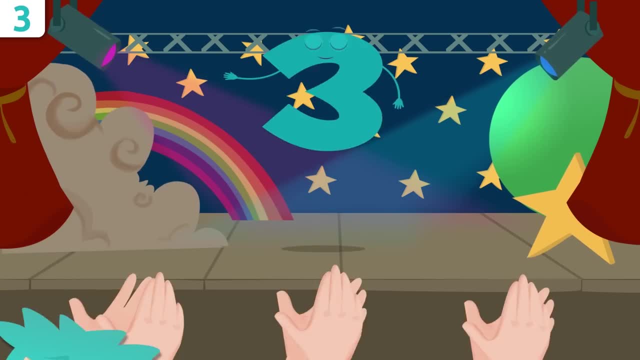 Today I'll be introducing you to number three. That's right, that's me, Number three, The most beautiful number of all. Why is that? Because I say so. I'm here to tell you all about me. What do you say? 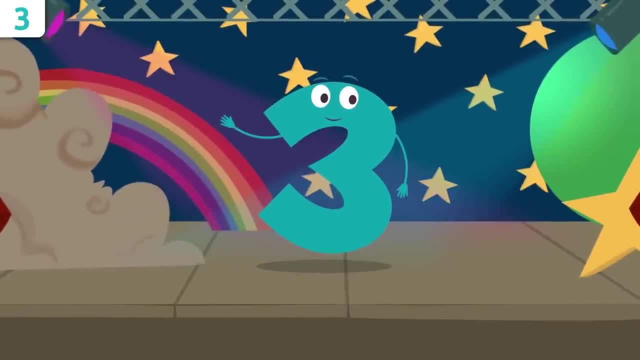 We're going to have a great time. Oh, and don't forget, we'll be singing a song at the end. Let's start by saying my name loud and clear. Repeat after me: Three, Two, One, Two, One. 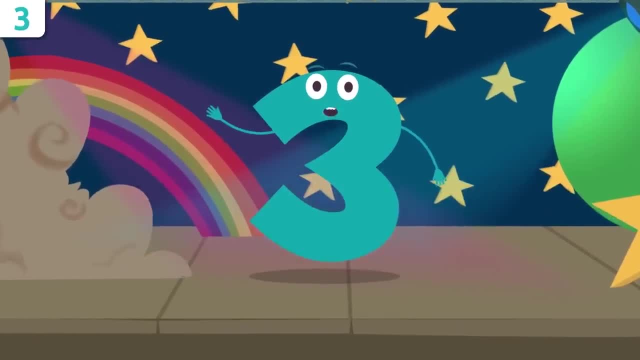 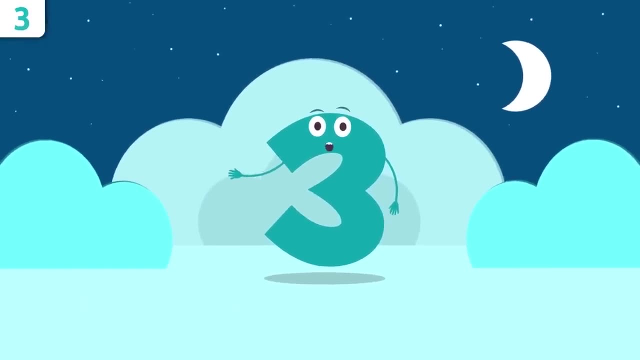 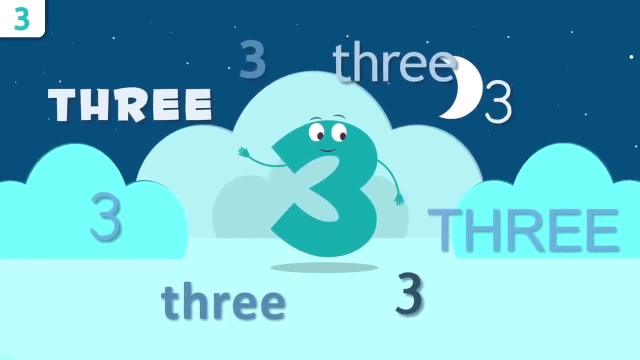 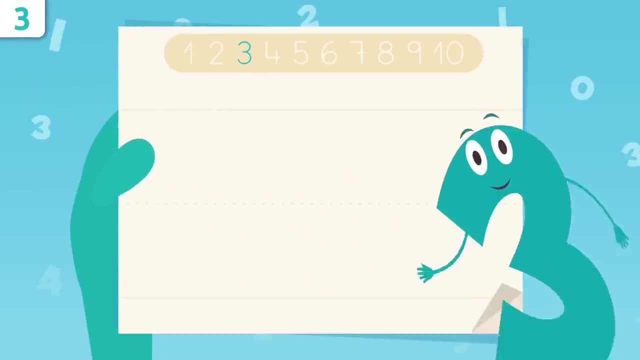 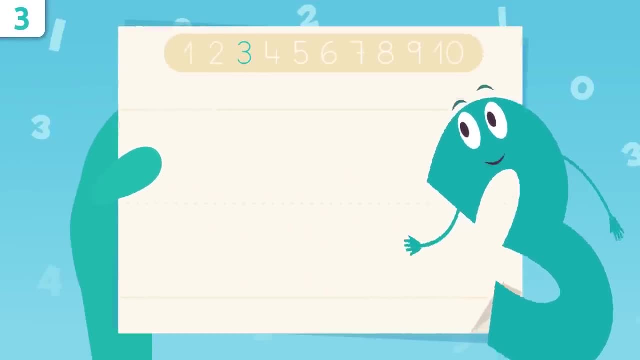 Two, One, Three, Louder Three. That's it Right. So now I'm going to show you how to write number three. Pay attention, We're going to start right here and we'll trace a curve, And then another curve, alllllll the way down. 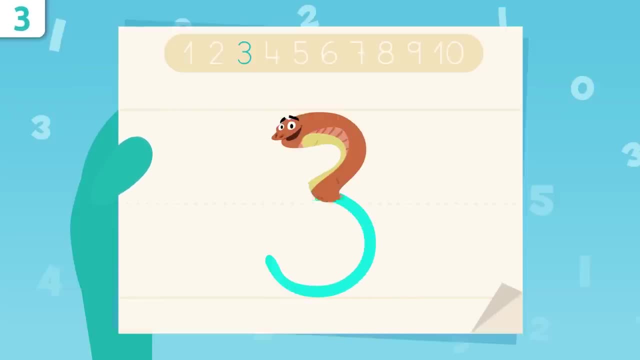 You got it. That was easy, right? Oh look, I look like a snake. Try it at home using some paper and a pencil. It's easy as pie. Let's look at some examples. Look, these are the athletes that won the race. 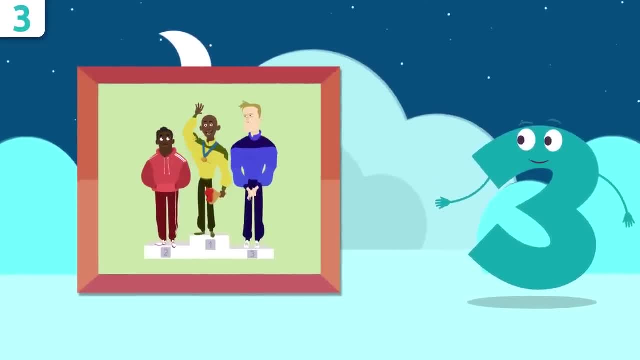 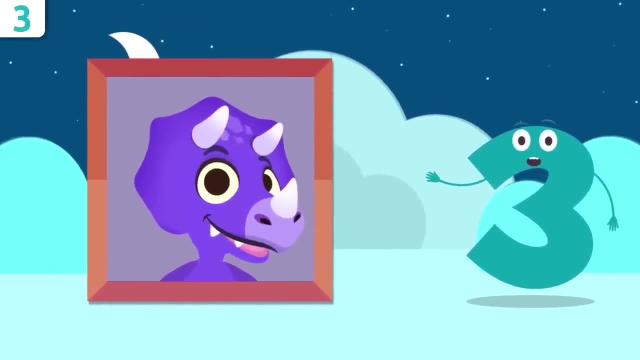 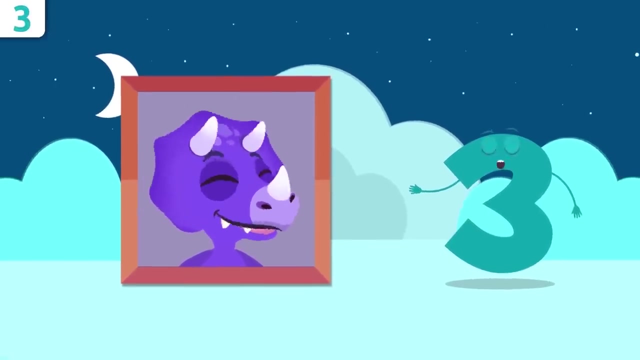 How many are there? One, two and three, But look, that's Sauri. Do you want to count how many horns our friend the dinosaur has got? One, two and three. Sauri has three horns. Will you sing with us later, Sauri? 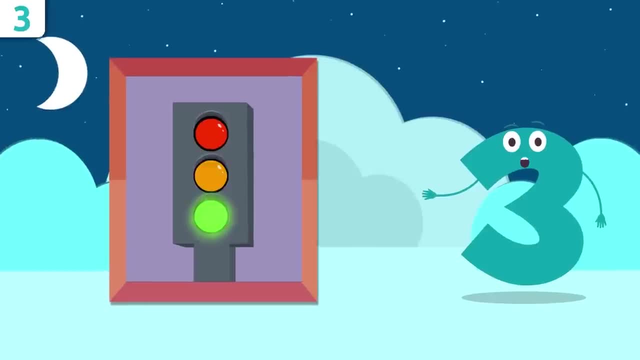 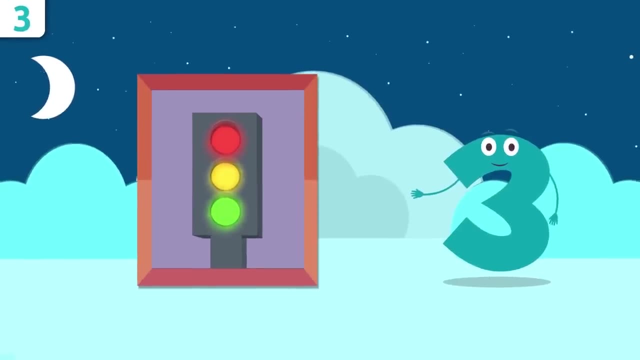 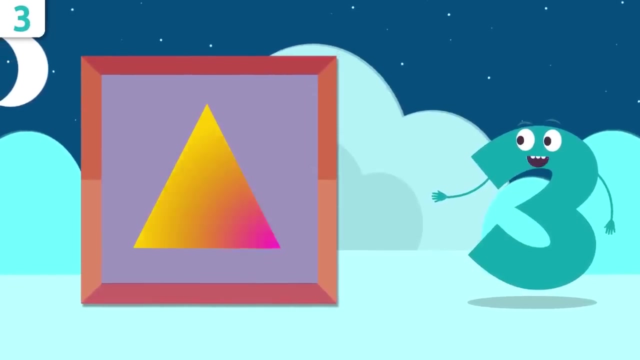 Look the traffic lights. How many circles are there? One, two and three. There are three circles on the traffic lights. Would you know how many points there are on this triangle? Let's see One, two and three. 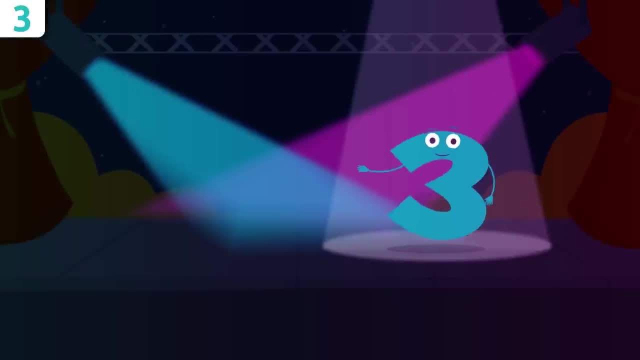 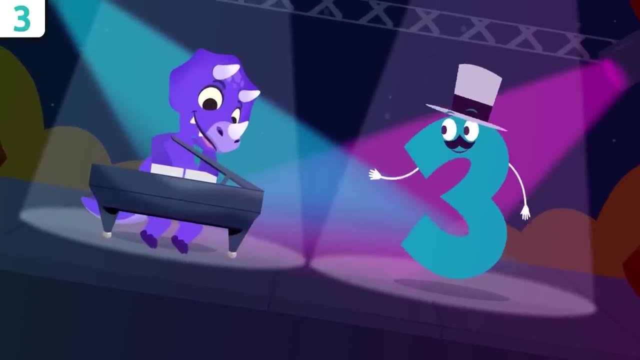 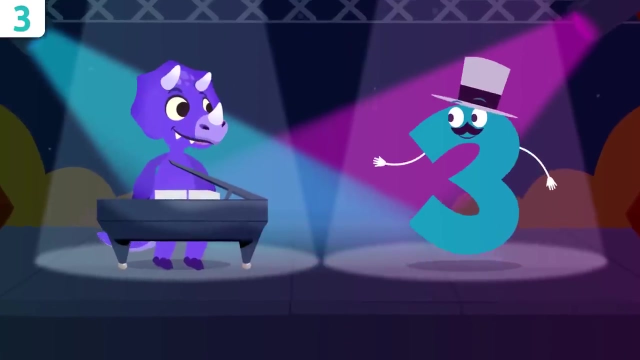 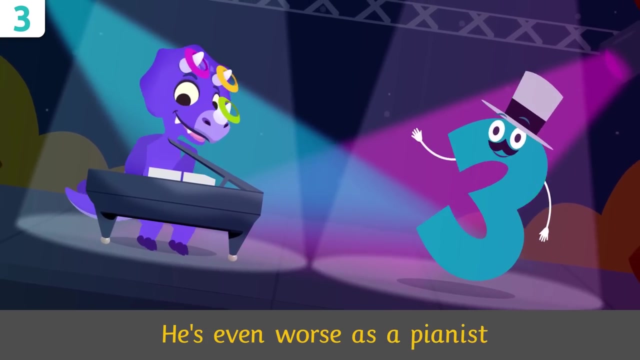 Way to go, friends. And now we're going to sing a little, as promised. Sauri Sauri's a really lousy artist. He's even worse as a pianist With his three horns, though The audience is going to wow. 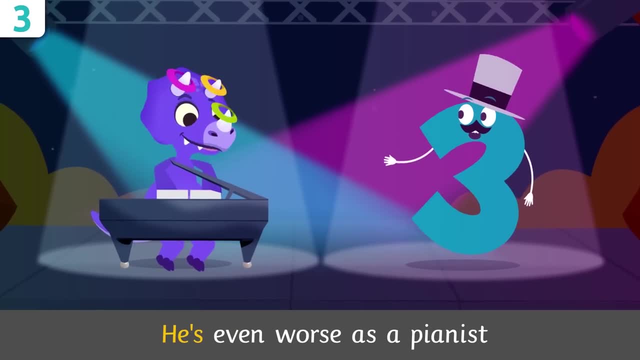 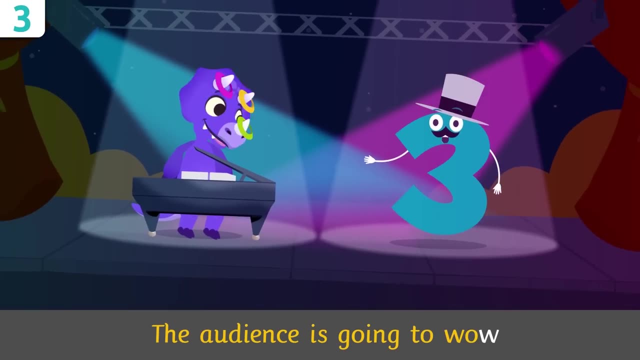 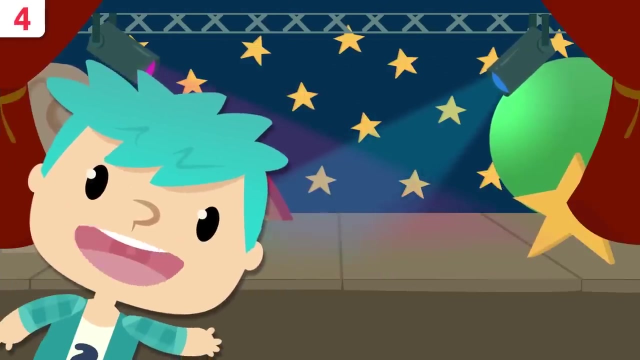 Sauri's a really lousy artist. He's even worse as a pianist. With his three horns, though, The audience is going to wow. He's even worse as a pianist. A very good morning to all of you. Today, I have the pleasure of presenting to you a very special number. 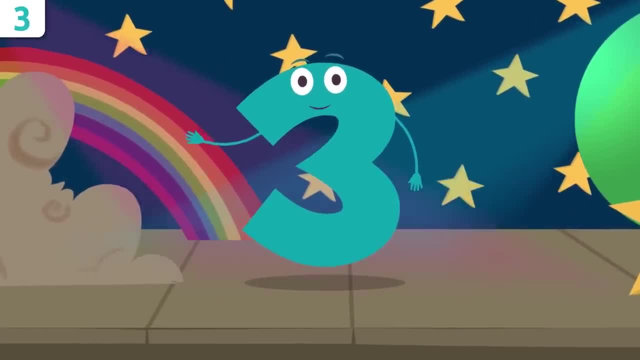 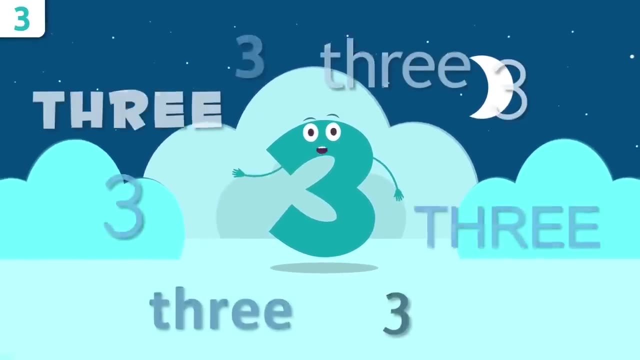 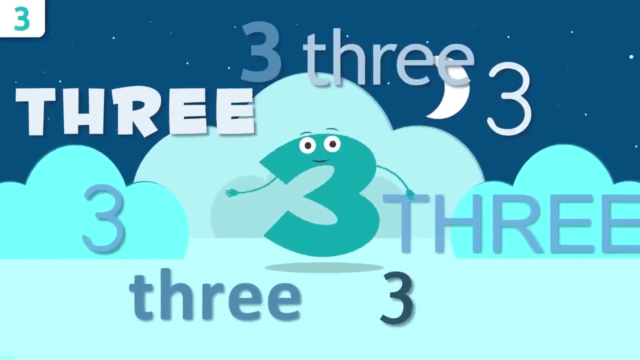 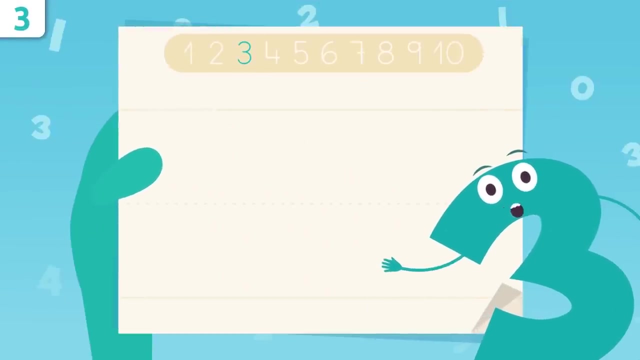 Oh, and don't forget, we'll be singing a song at the end. Let's start by saying my name loud and clear. Repeat after me Three, Three, Louder, Louder, Three. That's it Right. so now I'm going to show you how to write number three. 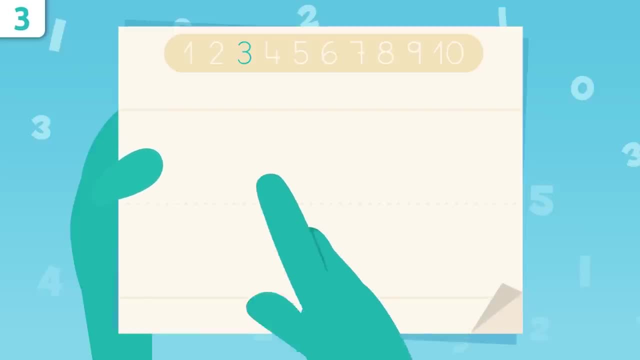 Pay attention. We're going to start right here and we'll trace a curve And then another curve all the way down. You got it. That was easy, right? Oh look, I look like a snake. Try it at home using some paper and a pencil. 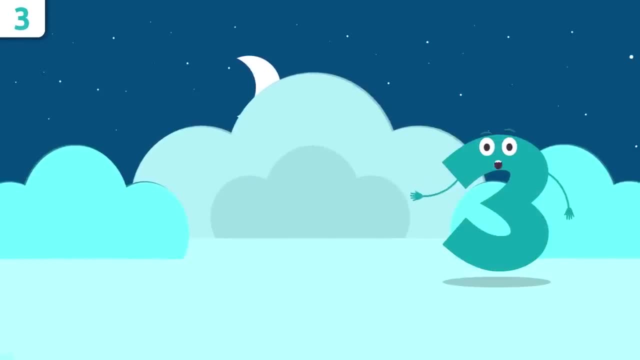 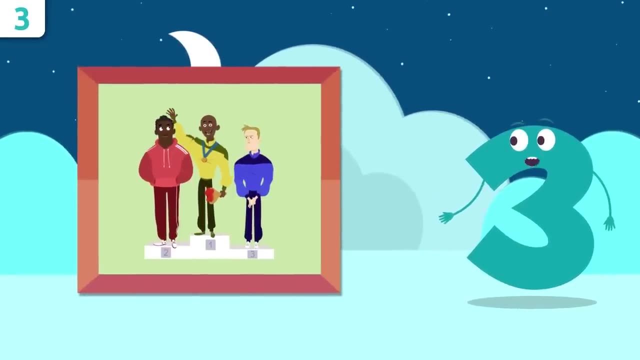 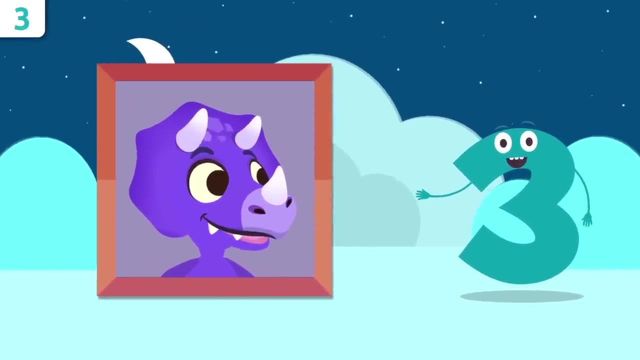 It's easy as pie. Let's look at some examples. Look, these are the athletes that won the race. How many are there? One, two and three. But look, that's Sauri. Do you want to count how many horns our friend the dinosaur has got? 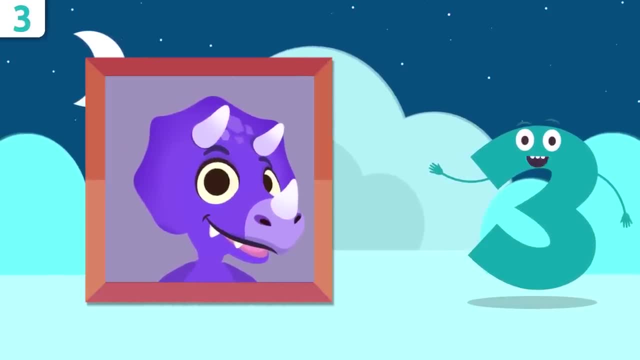 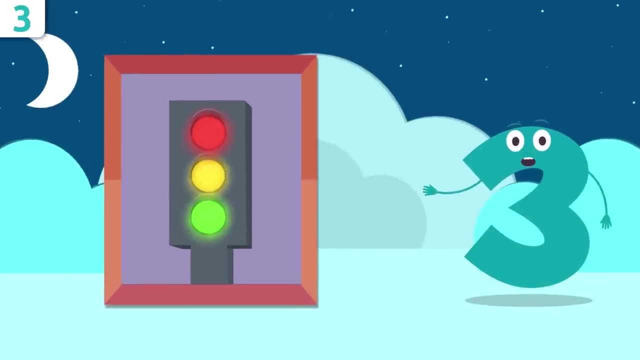 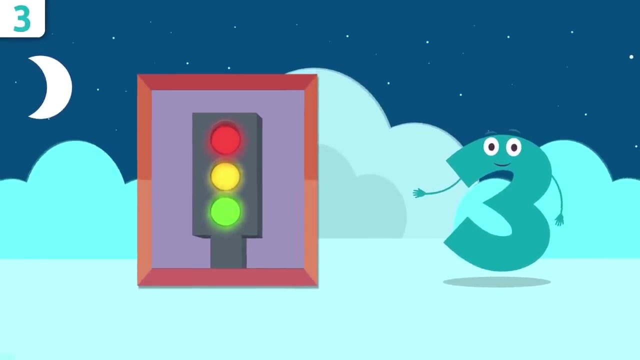 One, two and three. Sauri has three horns. Will you sing with us later, Sauri? Look the traffic lights. How many circles are there? One, two and three? There are three circles on the traffic lights. Would you know how many points there are on this triangle? 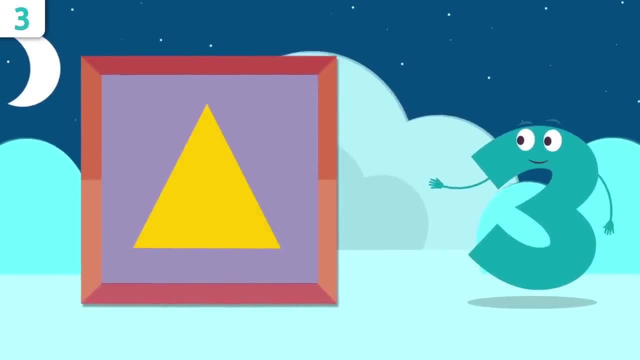 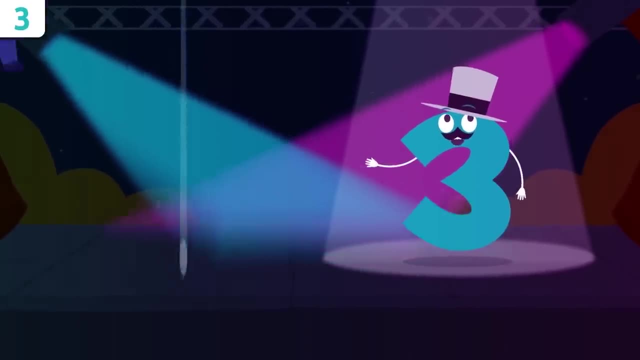 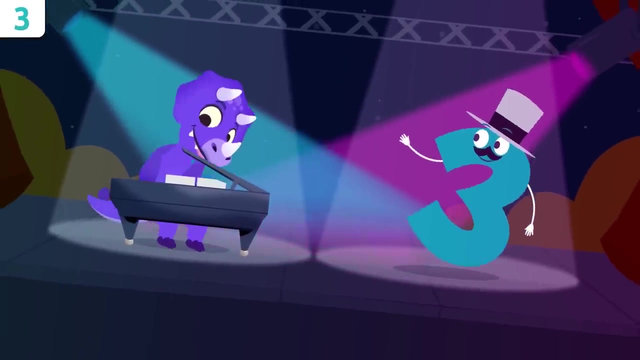 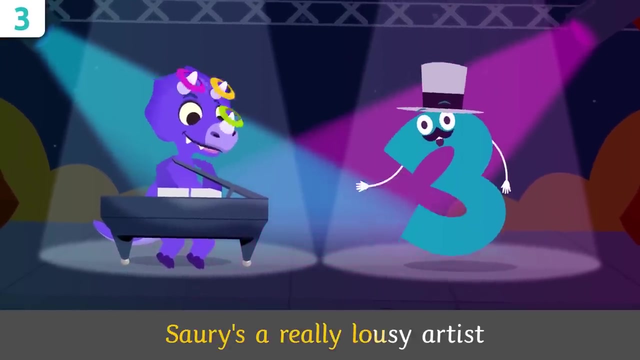 Let's see One, two and three Way to go, friends, And now we're going to sing a little, As promised. Sauri Sauri's a really lousy artist. He's even worse as a pianist, With his three horns, though. 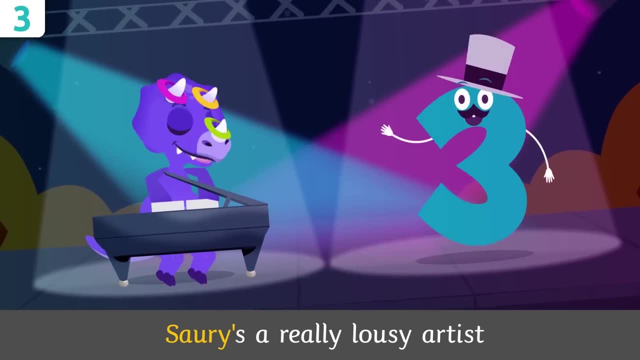 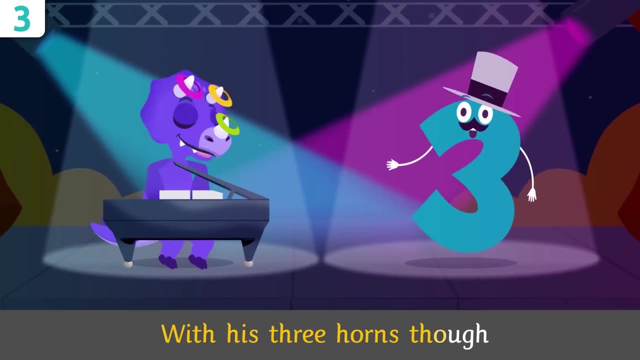 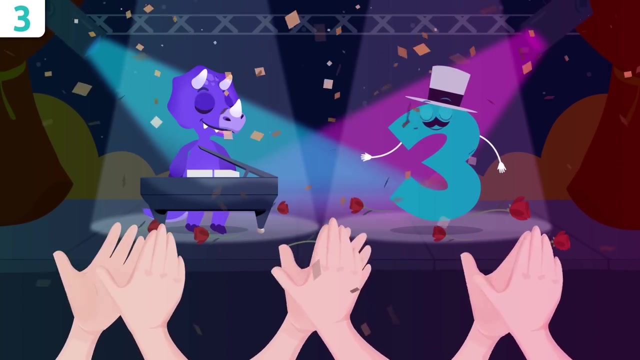 The audience is gonna wow. Sauri's a really lousy artist. He's even worse as a pianist With his three horns. though The audience Is going to wow- Applause. Thank you, Appreciate. A very good morning to all of you. 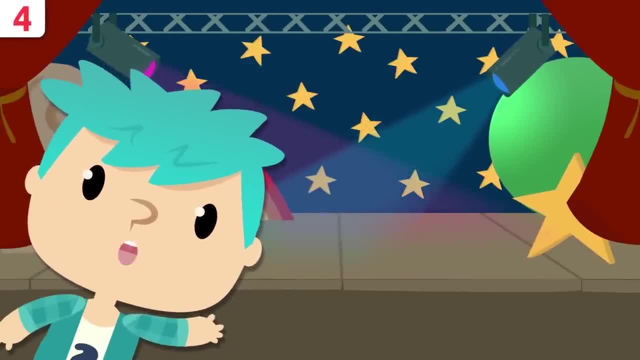 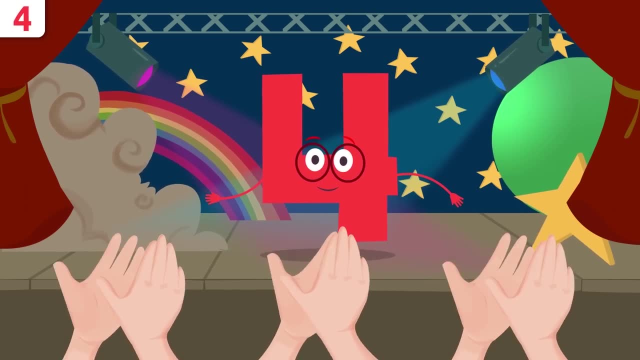 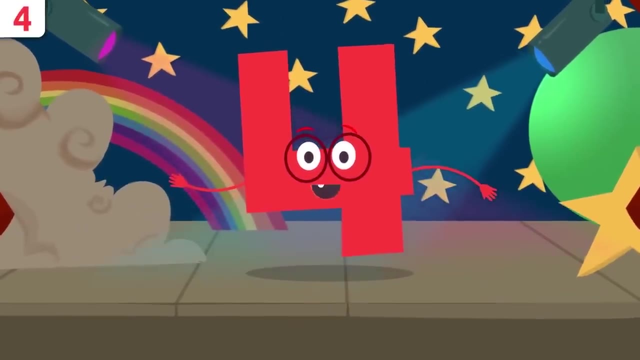 Today, I have the pleasure of presenting to you a very special number: Number 4!. Thank you all very much. Well, friends, I'm number 4!. Today, I'm going to tell you a few things about me. We'll be singing a song in the end. 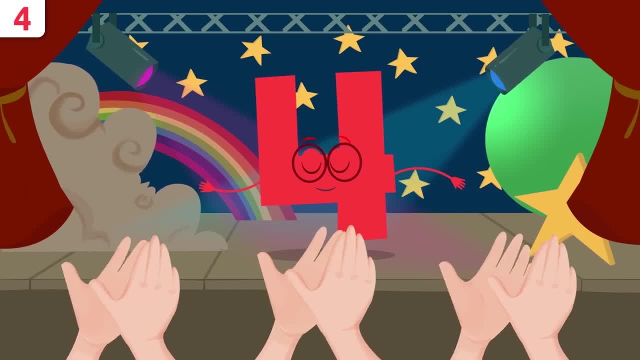 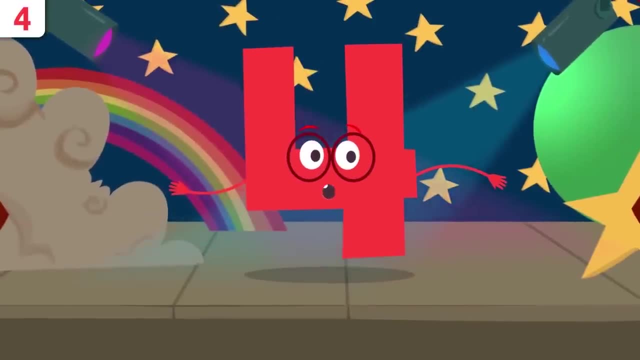 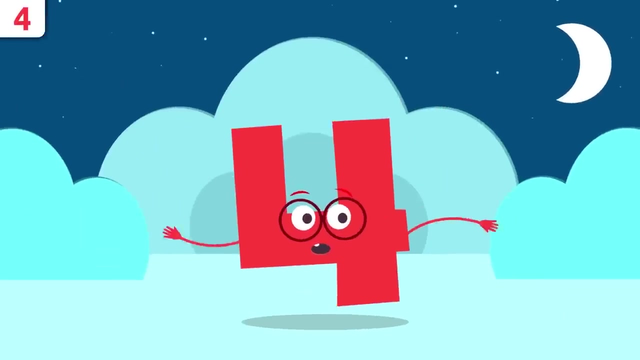 Number Four. Thank you all very much. Well, friends, I'm Number Four Today. I'm going to tell you a few things about me. We'll be singing a song in the end. Make sure you don't miss it. Sauri's a little lousy artist. He's even worse as a pianist. 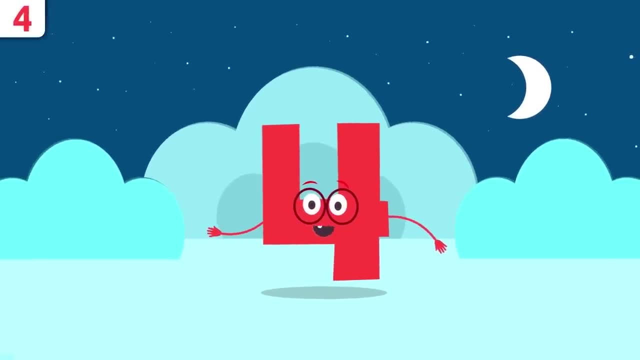 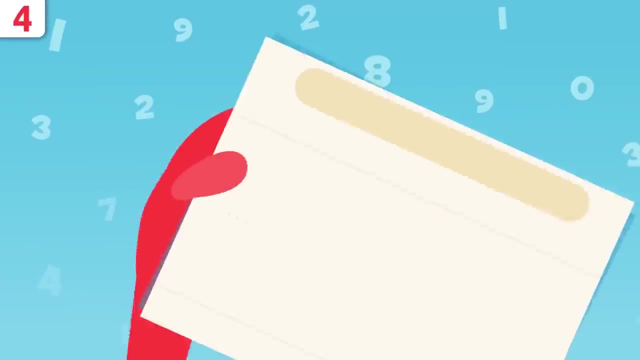 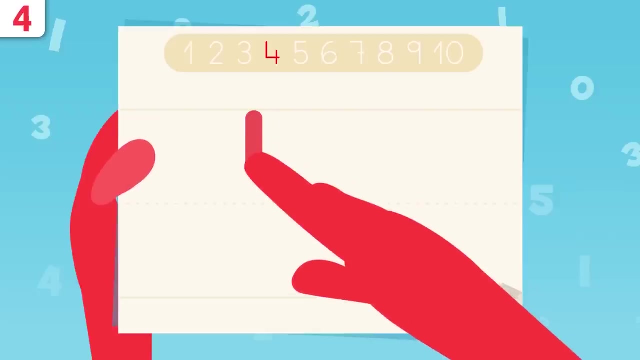 first of all, let me tell you my name. repeat after me: four, four, can't hear you- four, well done. now it's time to show you how we write number four. we start here and trace the line down. when we get to this point, we move to the right. 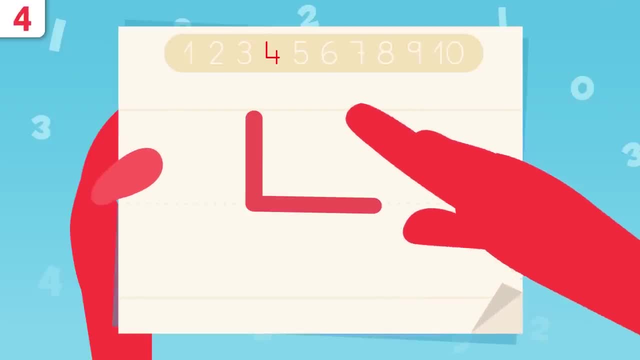 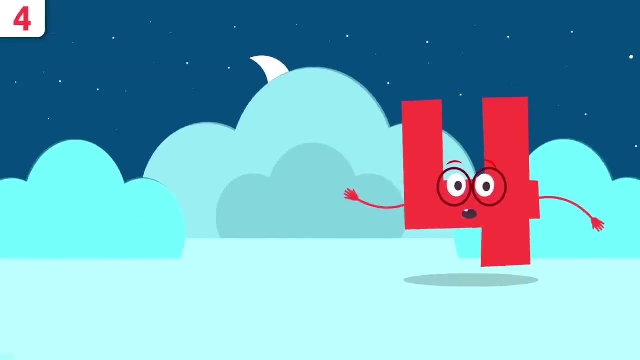 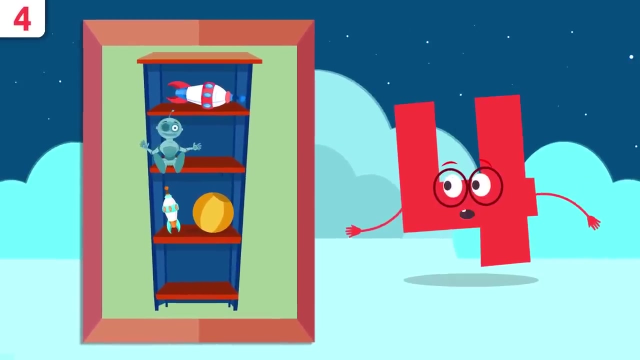 now we lift the pencil, we place it right here and we draw a straight line. that's it easy, right? have you noticed i look like a chair upside down? try tracing number four at home. it's easy as pie. let's look at some examples. how many toys are there on the shelves? there's one, two, three. 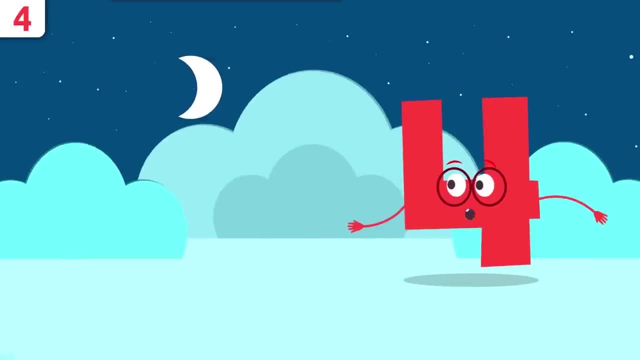 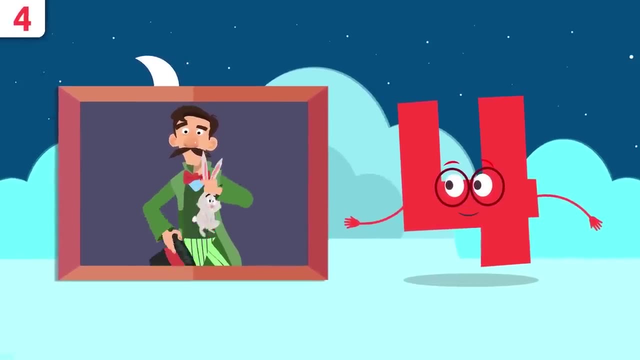 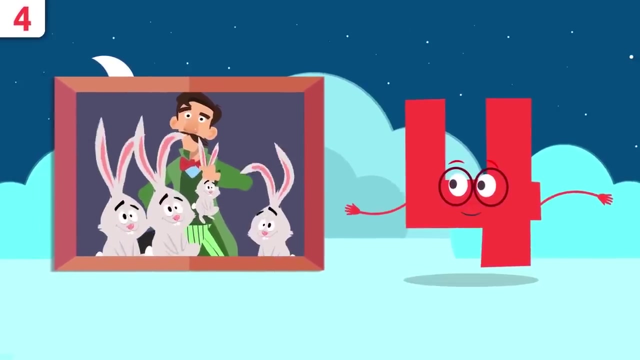 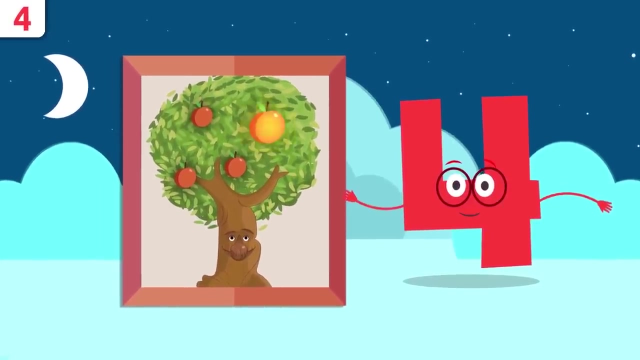 and four, four toys. look, it's our friend hazard the wizard. how many bunnies have you pulled out of your hat? let's see one, two, three and four. there are four bunnies. how many apples are there on the tree? let's see one, two, three and four. would you know how many legs? 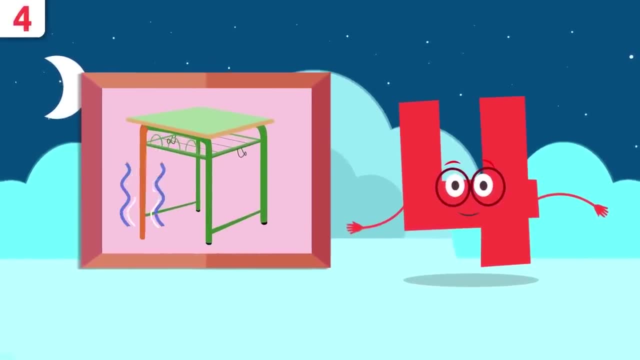 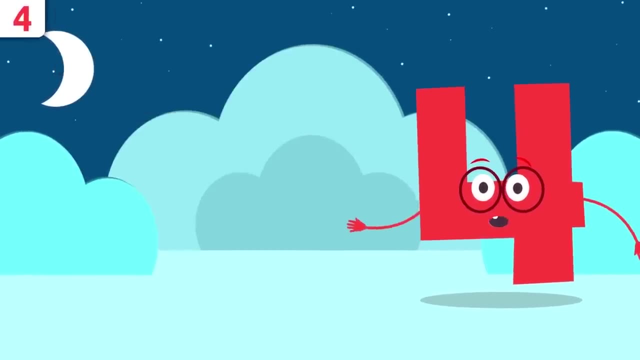 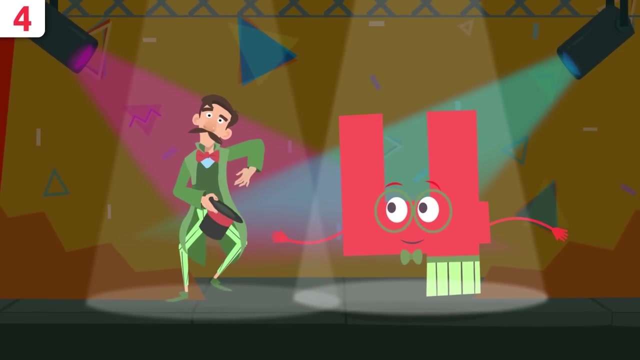 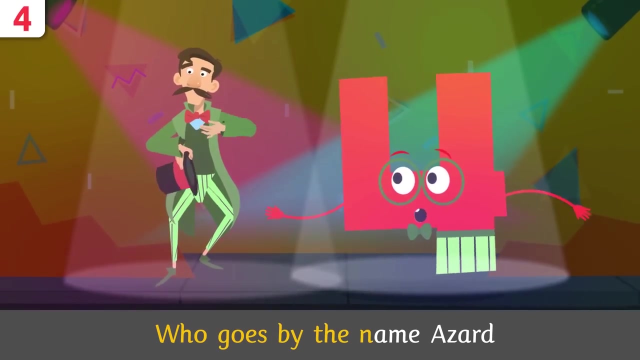 This table has one, two, three and four. The table has four legs. You did very well, friends. Time to jiggle and dance. a little Wizard Hazard. come join us. Four bunnies pulled the wizard who goes by the name Hazard. 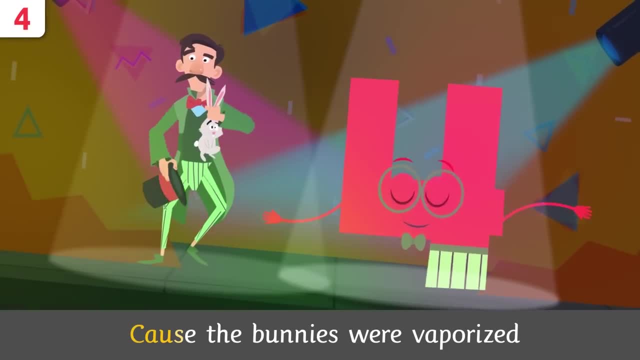 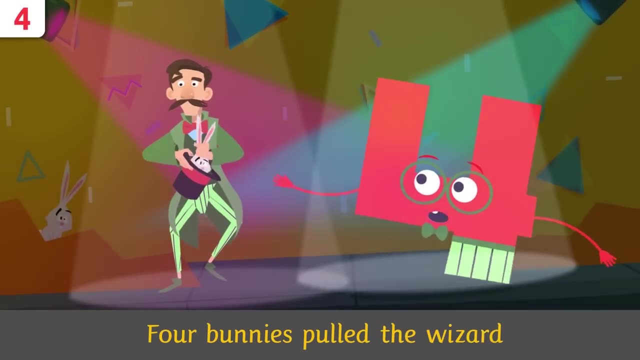 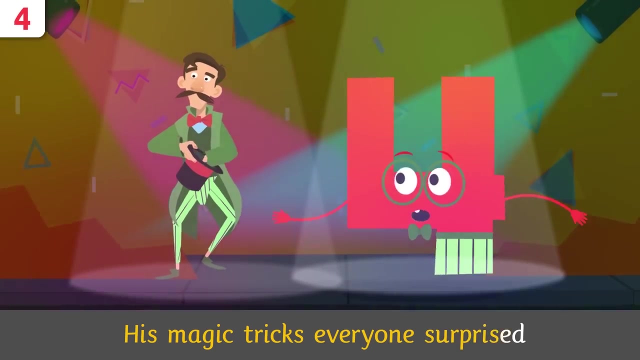 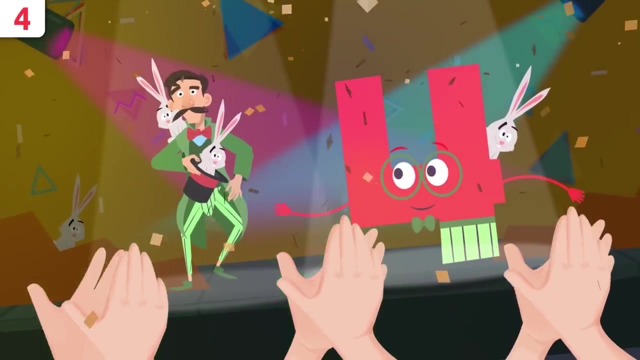 His magic tricks, everyone surprised, cause the bunnies were vaporized. Four bunnies pulled. the wizard who goes by the name Hazard. His magic tricks, everyone surprised, cause the bunnies were vaporized. Hello, How are you doing, friends of numbers? 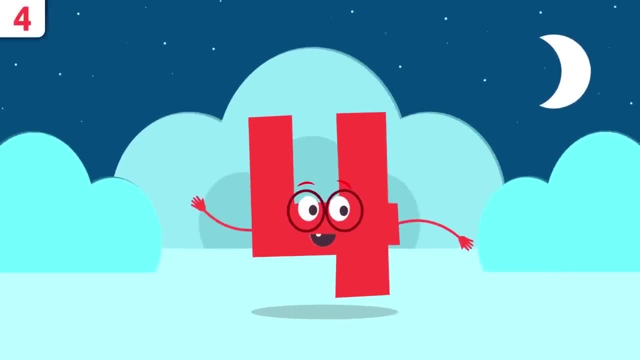 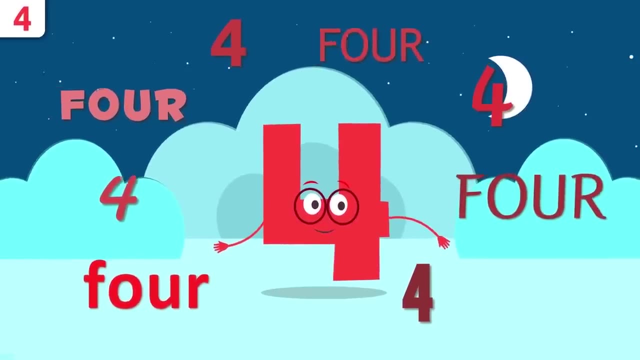 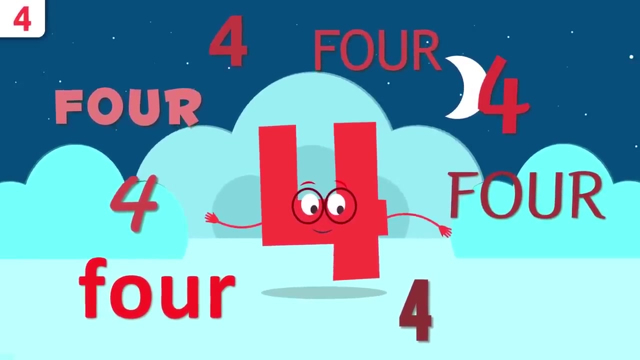 Make sure you don't miss it. First of all, let me tell you my name. Repeat after me: 4!, 4!, Can't hear you? 4!. Well done. Now it's time to show you how we write number 4.. 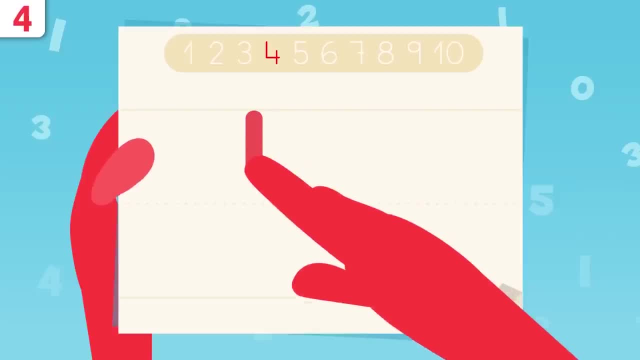 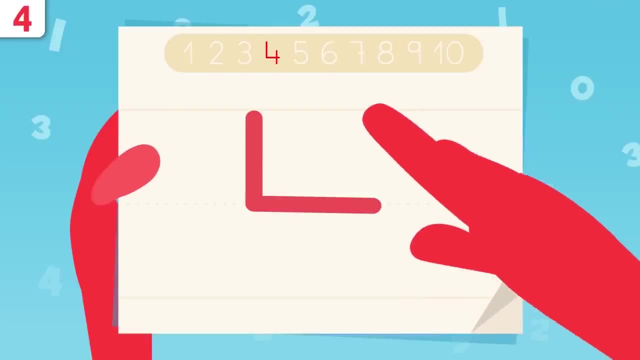 We start here and trace the line down. When we get to this point, we move to the right. Now we lift the pencil, we place it right here and we draw a straight line. That's it Easy, right? Have you noticed I look like a chair upside down? 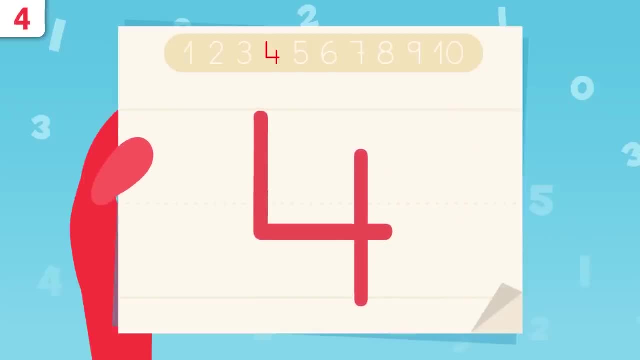 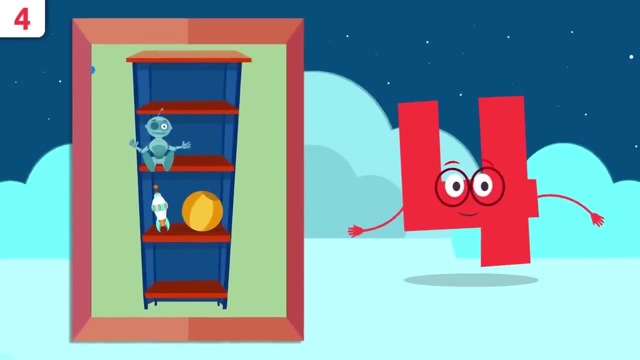 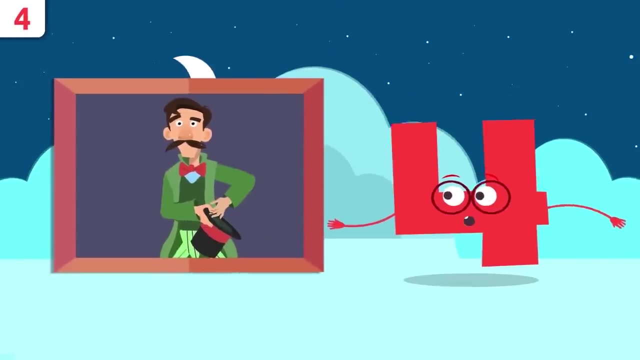 Try tracing number 4 at home. It's easy as pie. Let's look at some examples. How many toys are there on the shelves? There's 1,, 2,, 3, and 4! 4 toys. Look, It's our friend. 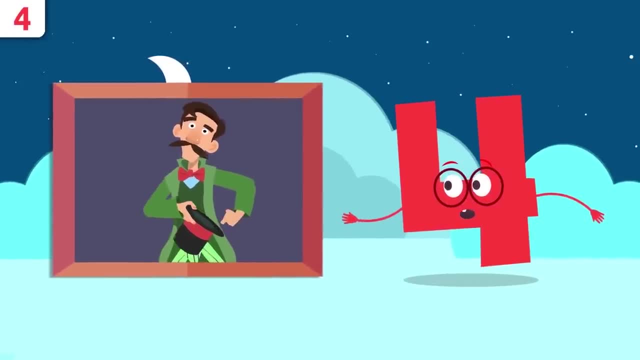 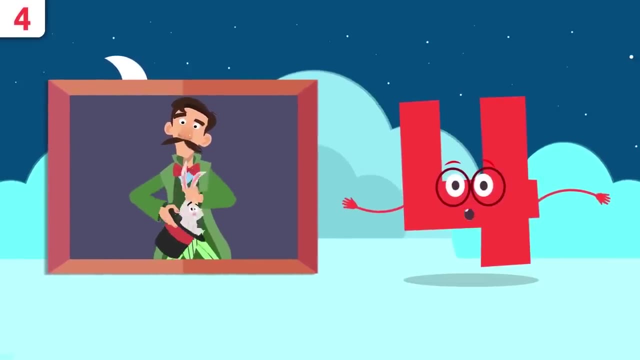 Hazard the Wizard. How many bunnies have you pulled out of your hat? Let's see 1,, 2,, 3, and 4!. There are 4 bunnies. How many apples are there on the tree? 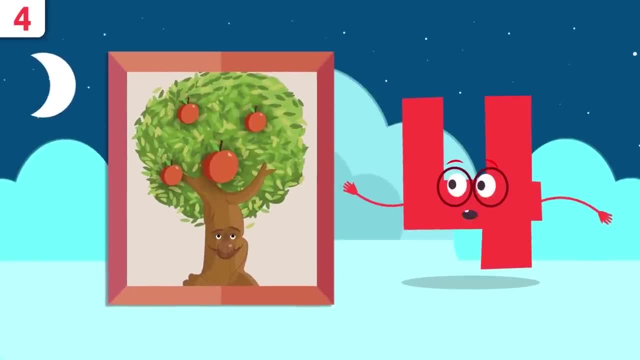 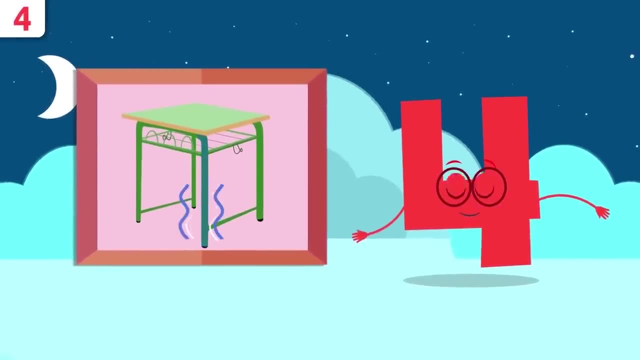 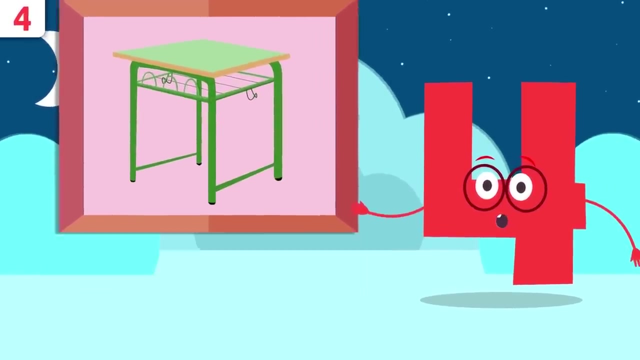 Let's see 1,, 2,, 3, and 4!. Would you know how many legs this table has? 1,, 2,, 3, and 4!. The table has 4 legs. You did very well, friends. Time to jiggle and dance a little. 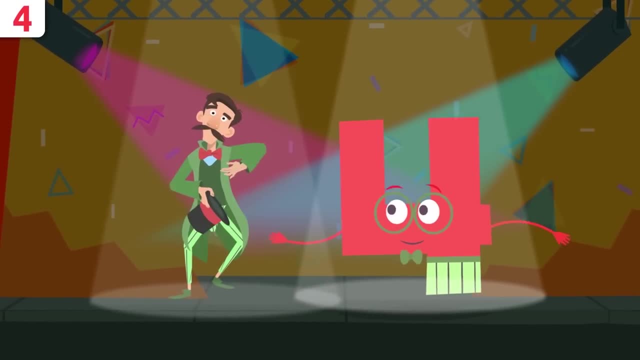 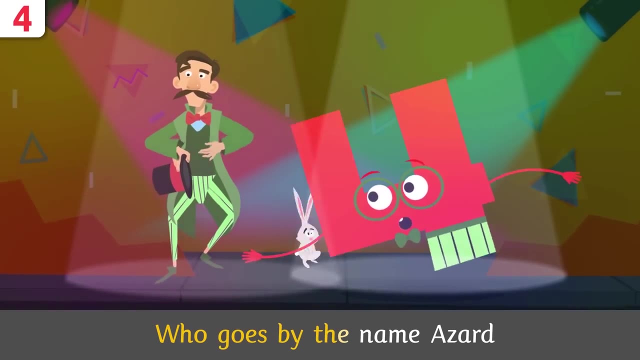 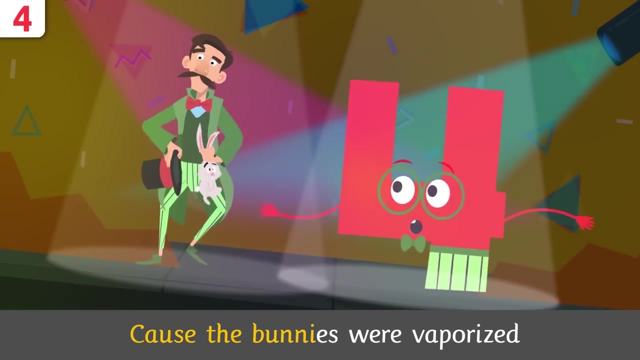 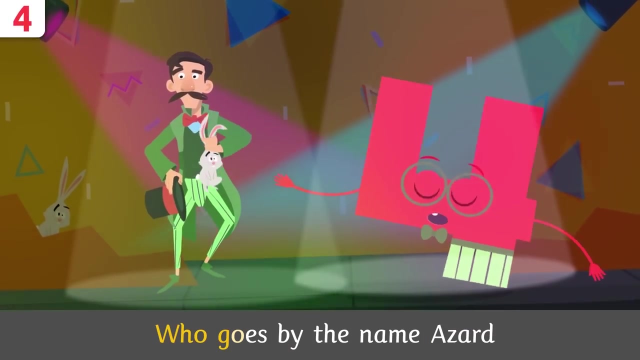 Wizard Hazard. come join us. Four bunnies pulled the wizard who goes by the name Hazard. His magic tricks everyone surprised, cause the bunnies were vaporized. Four bunnies pulled the wizard who goes by the name Hazard. 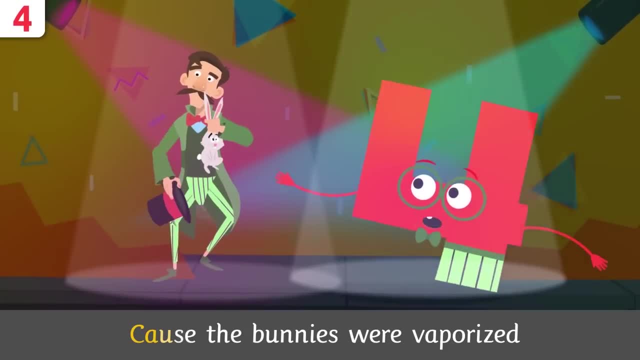 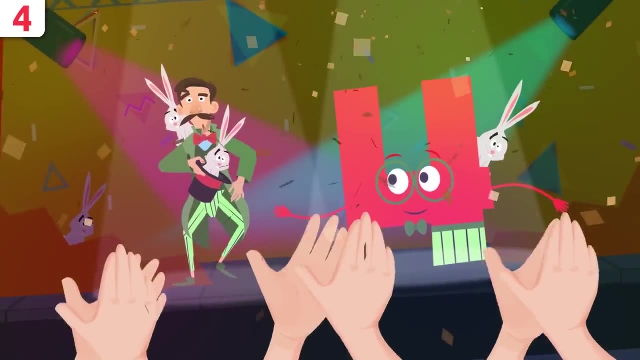 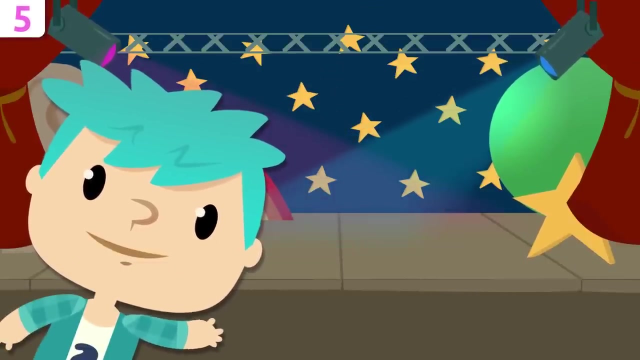 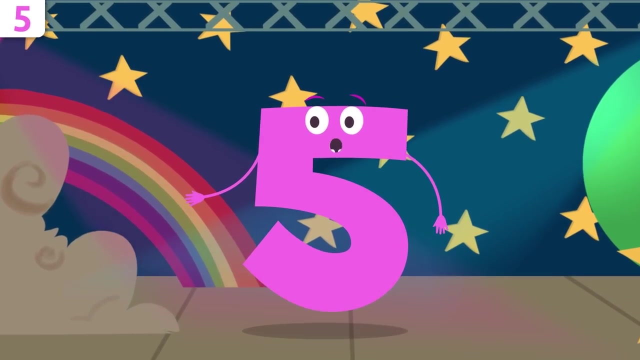 His magic tricks. everyone surprised cause the bunnies were vaporized. Hello, How are you doing? friends of numbers, I'm going to introduce to you number five. Hey, how's it going? I'm number five And I'm going to tell you a little bit about myself. 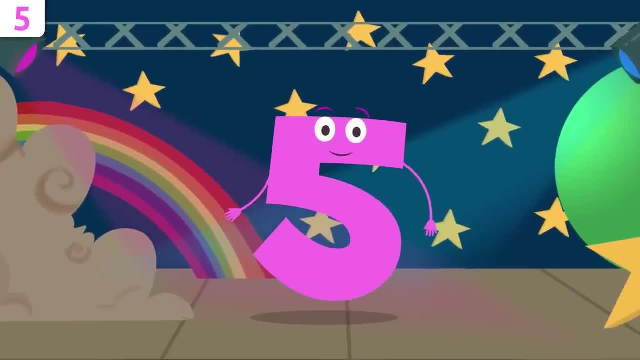 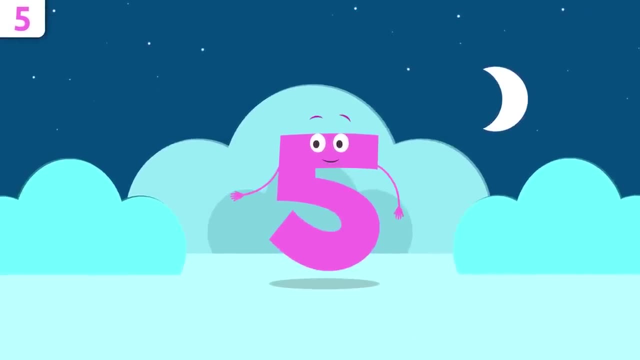 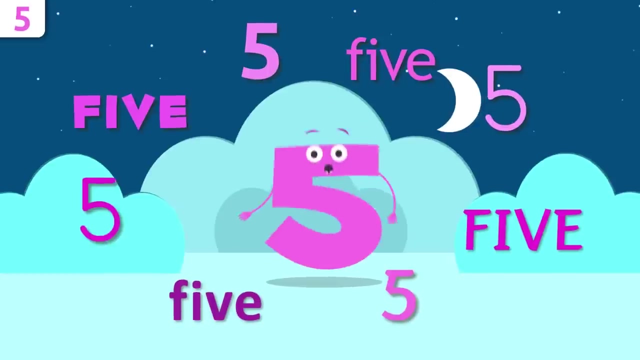 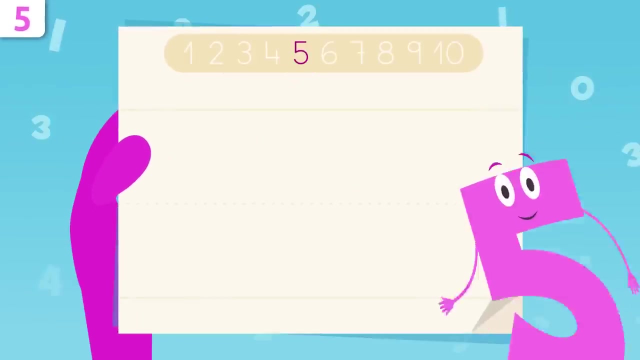 Are you ready? We'll be singing a song in the end. Would you like to stay? Let's start by saying my name. Repeat after me: Five, Five, Louder, Five, Five. That's it. Now I'm going to show you how to trace number five. 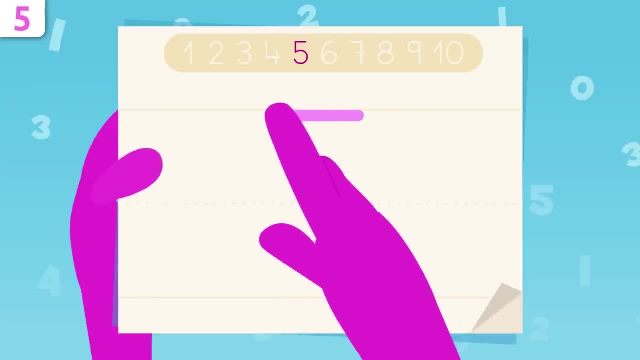 Let's start right here, tracing a straight line to the left. When we get to this point, we start tracing down, and now we draw a big curve, finishing right here. That's it, friends, Easy peasy, right. Look, I look like a penguin. 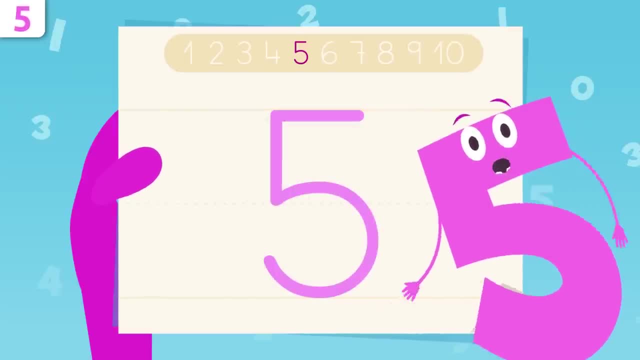 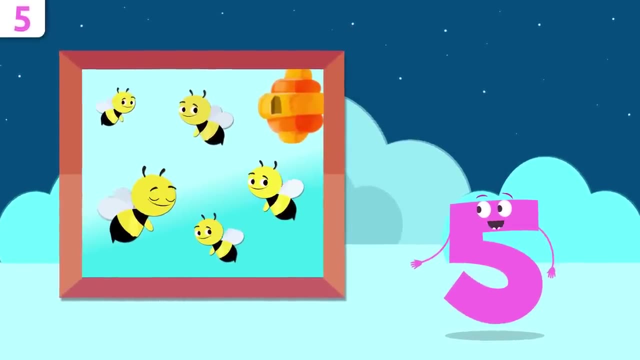 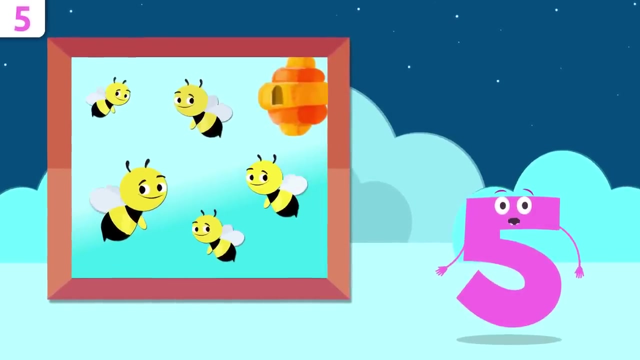 Try it at home using some paper and a pencil. It's really easy. Let's look at some examples. How many bees are there in this honeycomb? One, two, three, four and five? There are five bees. How many cars are there? 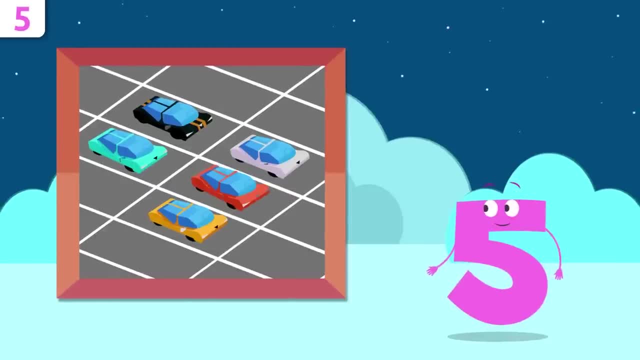 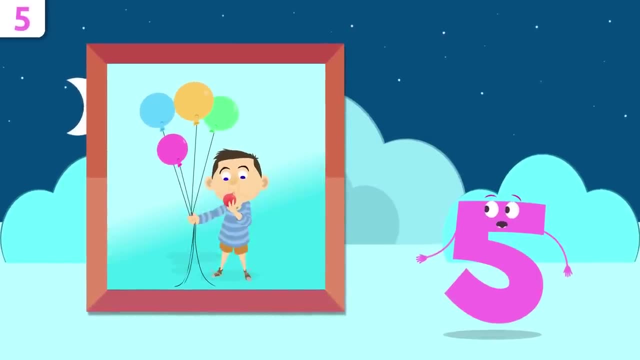 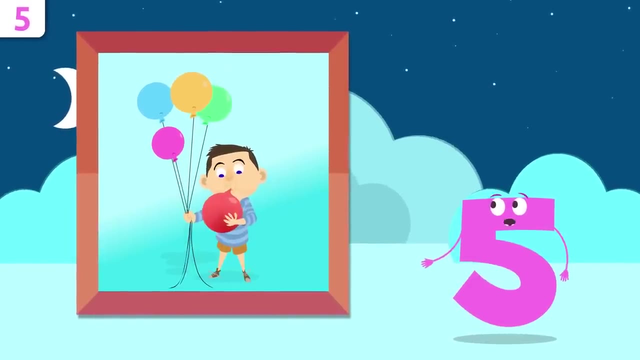 One, two, three, four and five. There are five cars. And how many balloons does our friend Mike have? One, two, three, four and five. He has five balloons. Don't go very far, Mike. We're going to be singing later. 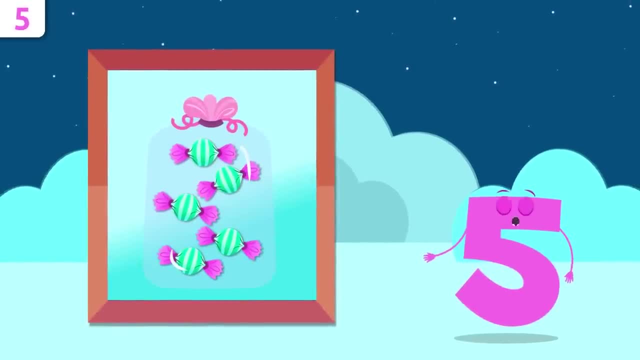 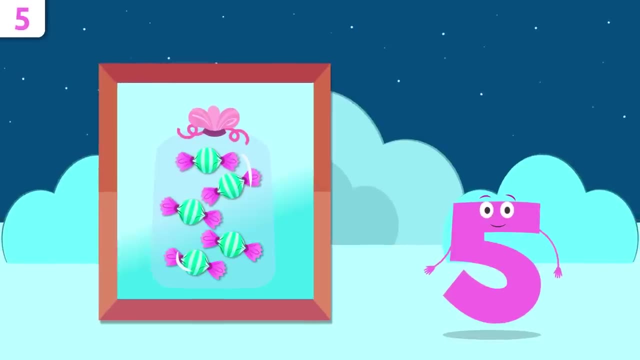 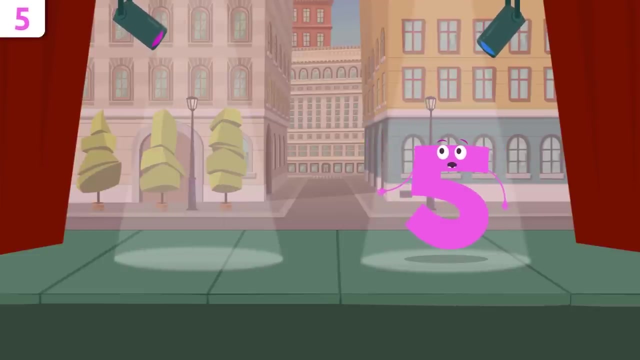 Mmm yum Candy. How many gummies are there? One, two, three, four and five. There are five gummies. You did very well, friends. Do you want to sing a little? Mike, Come join me. 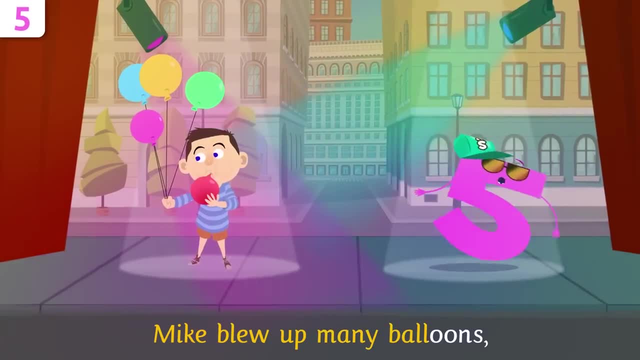 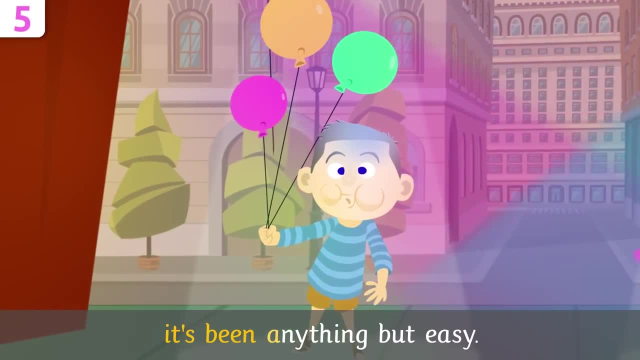 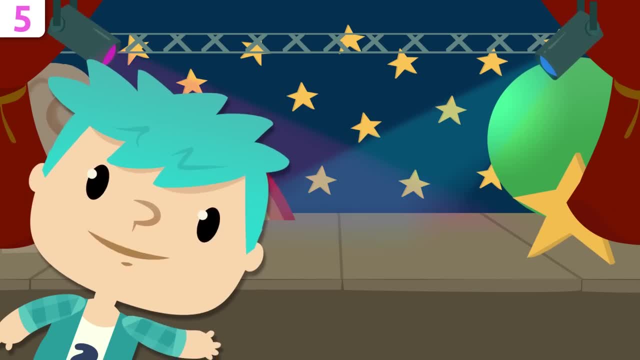 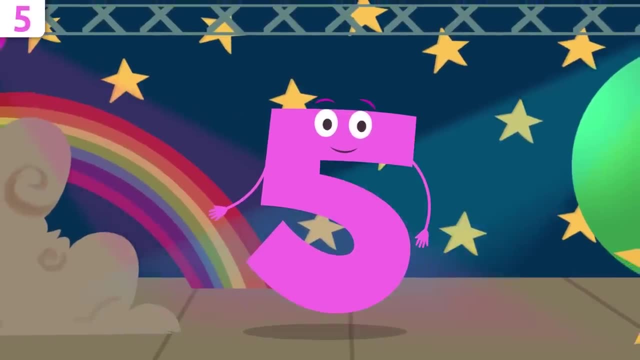 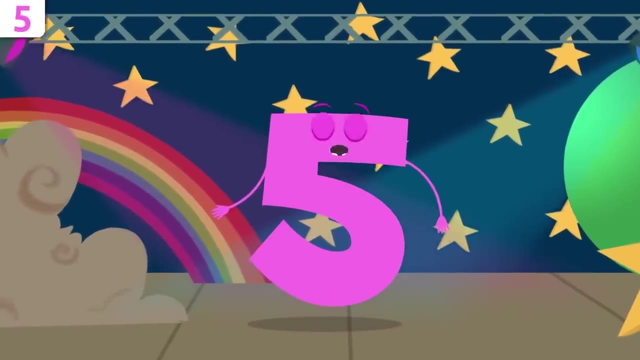 I'm going to introduce to you number five. Hey, how's it going? I'm number five And I'm going to tell you a little bit about myself. Are you ready? We'll be singing a song in the end. Would you like to stay? 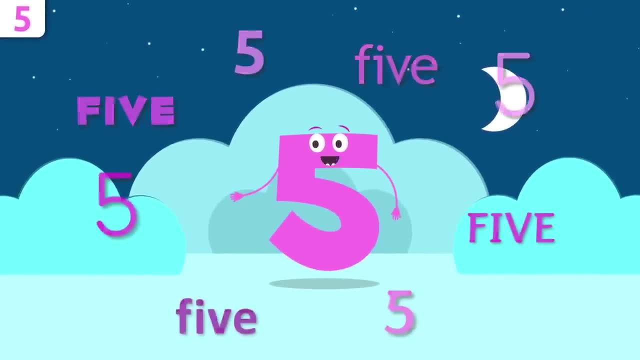 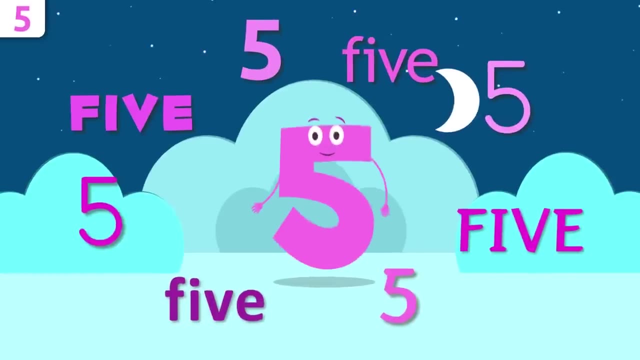 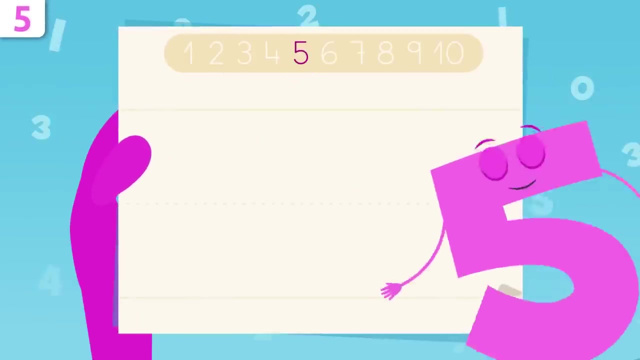 Let's start by saying my name. Repeat after me Five, Five, Louder Five. That's it. Now I'm going to show you how to trace number five. Let's start right here, tracing a straight line to the left. 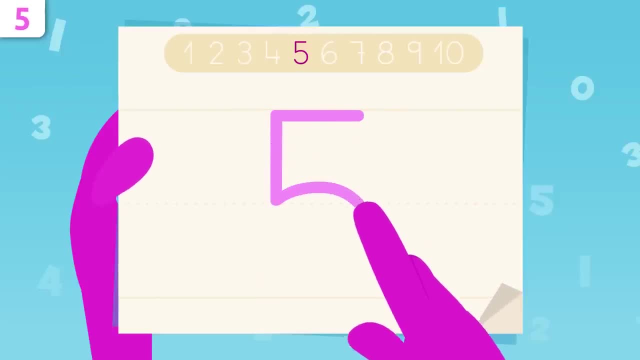 When we get to this point, we start tracing down, and now we draw a big curve, finishing right here. That's it, friends, Easy peasy, right. Look, I look like a penguin. Try it at home using some paper and a pencil. 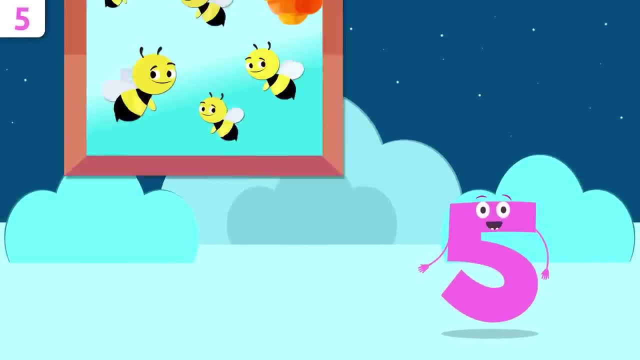 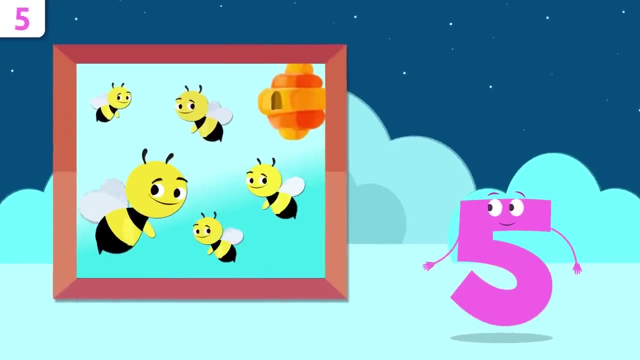 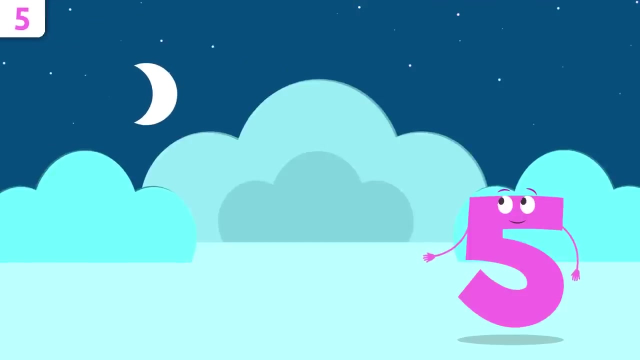 It's really easy. Let's look at some examples. How many bees are there in this honeycomb? One, two, three, four and five? There are five bees. How many cars are there? One, two, three, four and five? 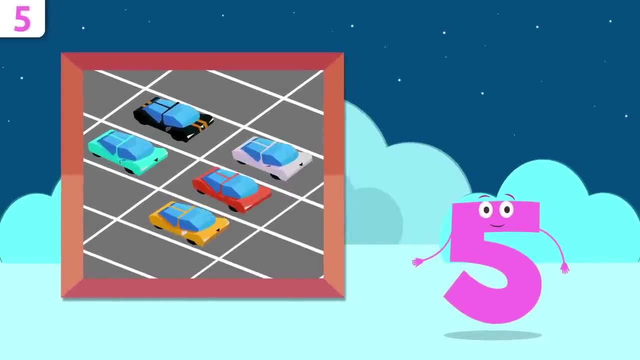 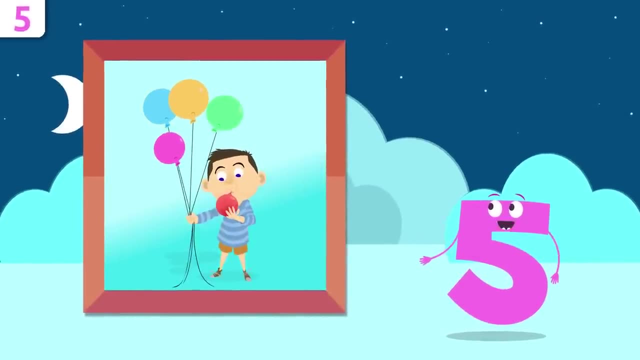 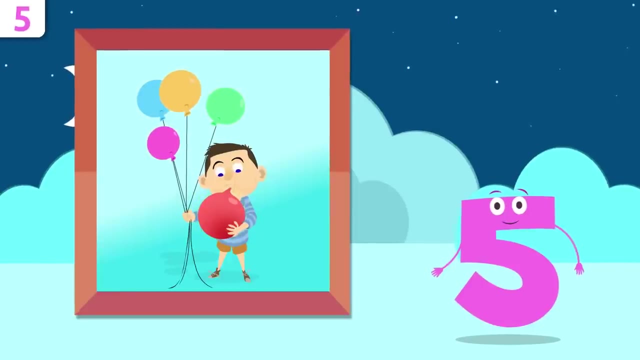 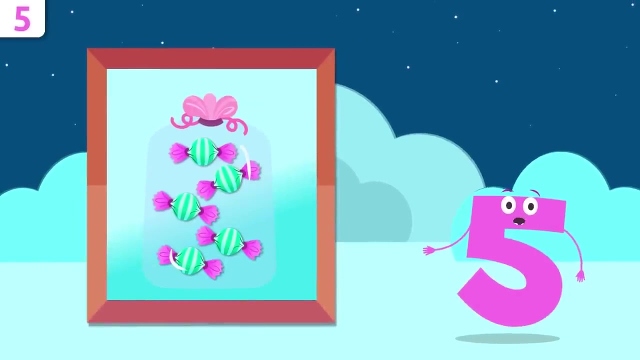 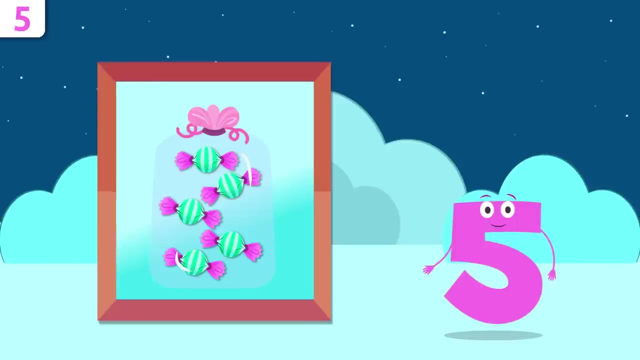 There are five cars. There are five cars. five, there are five cars. and how many balloons does our friend mike have? one, two, three, four and five. he has five balloons. don't go very far, mike. we're going to be singing later: um yum candy. how many gummies are there? one, two, three, four and five? there are five gummies. 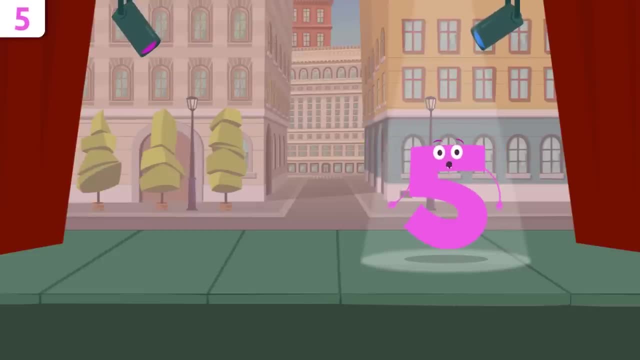 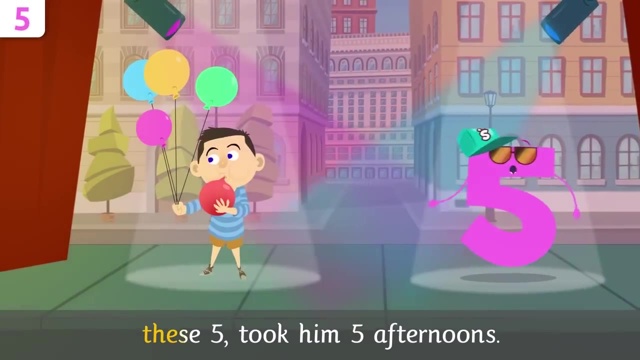 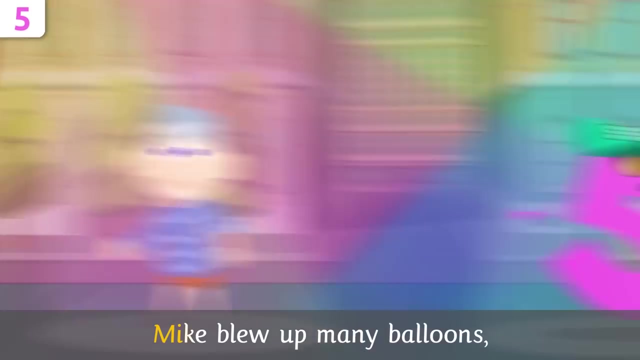 you did very well. friends, do you want to sing a little mike? come join me. mike flew up many balloons. these five took him five afternoons. he's been busy and so dizzy it's been anything but Mike flew up many balloons. These five took him five afternoons. 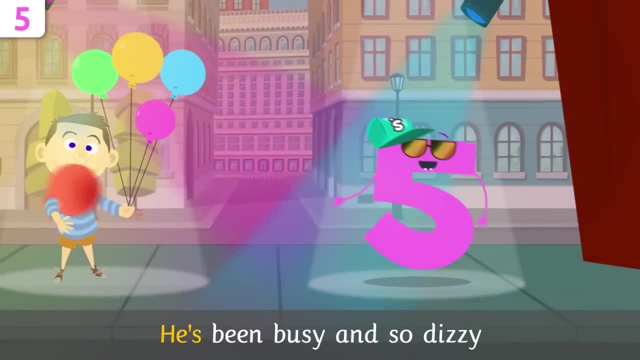 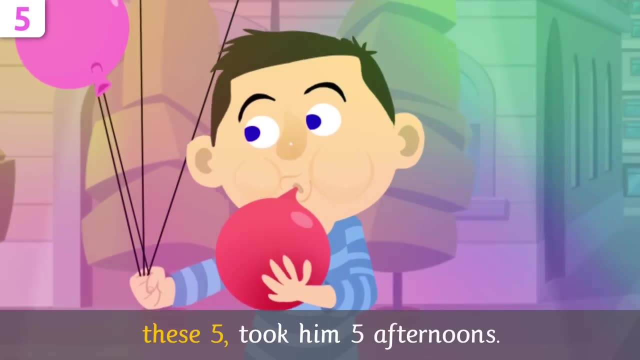 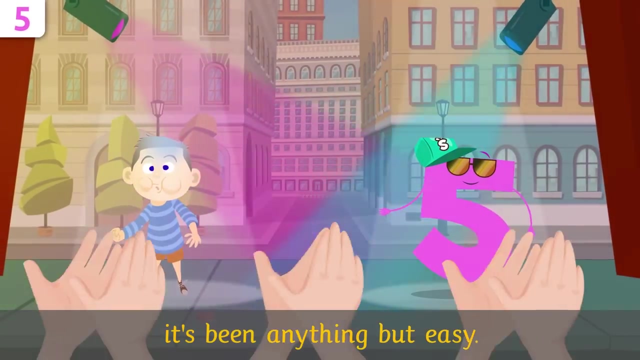 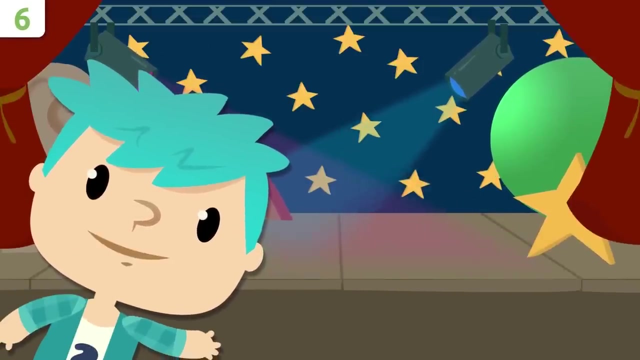 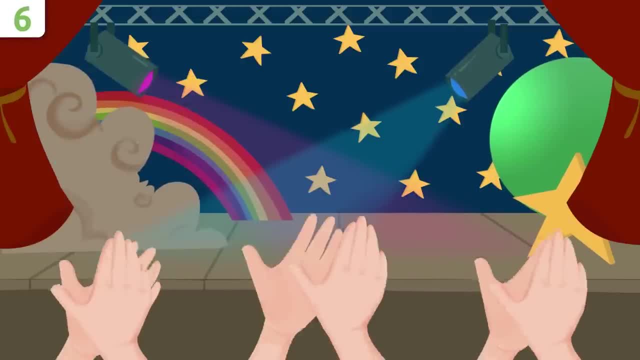 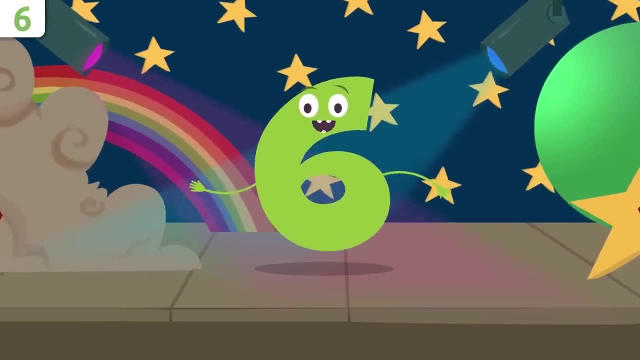 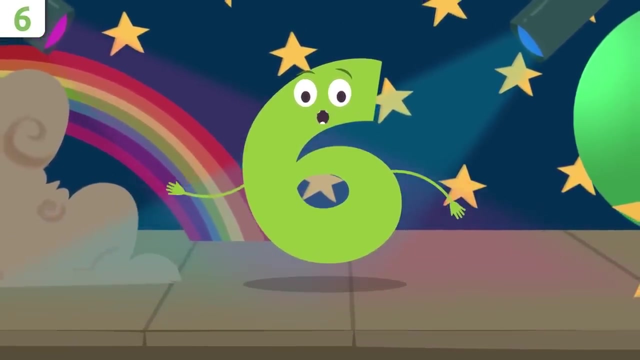 Today I'll be introducing number six. A very good morning to everyone. Do you know Which number I am? I'm number six. Stay with me till the end. We have a song for you. Let's start with my name. 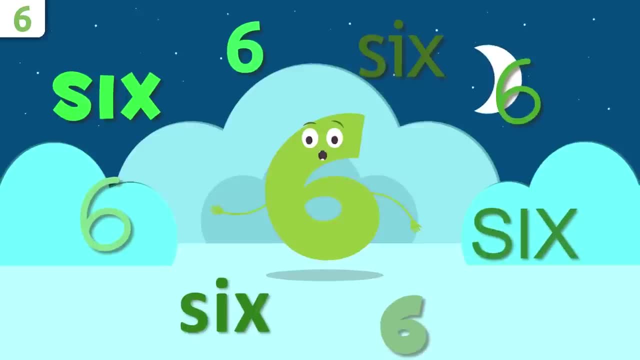 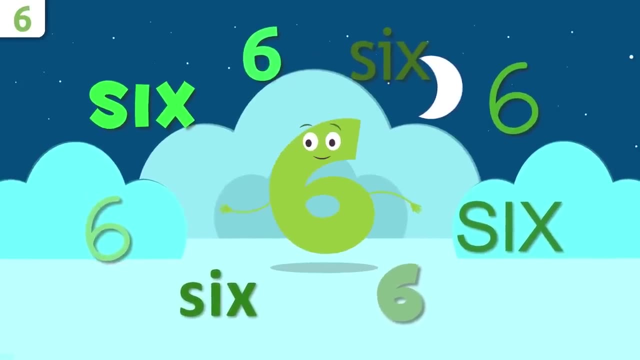 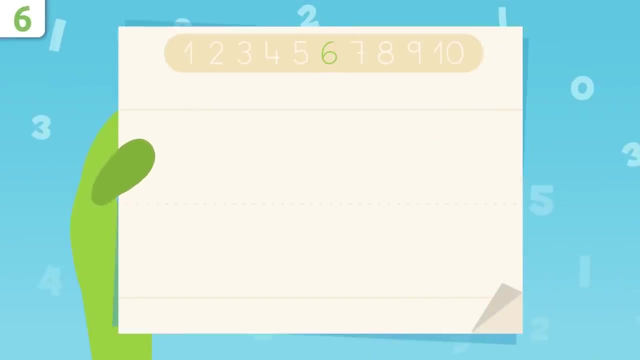 Repeat after me: Six, Six, Can hear you- Six. Excellent. Now I'll show you how to write number six. We start up here and trace down, drawing a curve. Now we trace like this, making a circle. You did great. 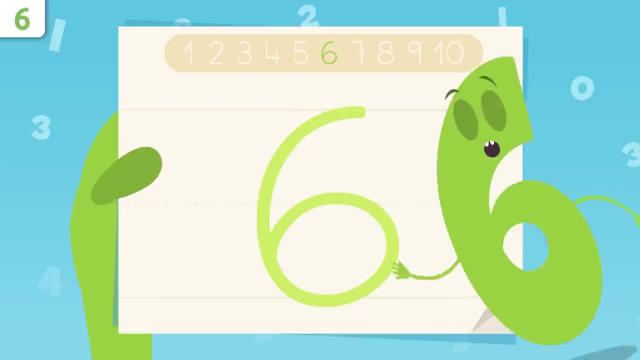 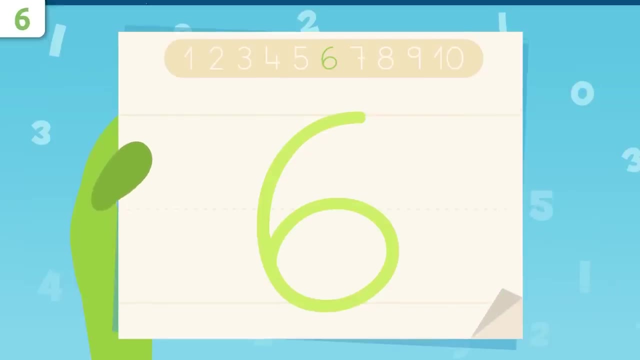 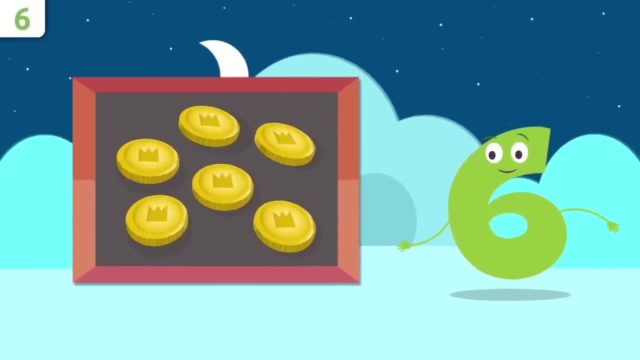 Look, I look like a whistle. Try it at home using some paper and a pencil. It's easy as pie. Did you want to look at some examples? Someone's dropped a few coins. How many are there? One, Two, Three. 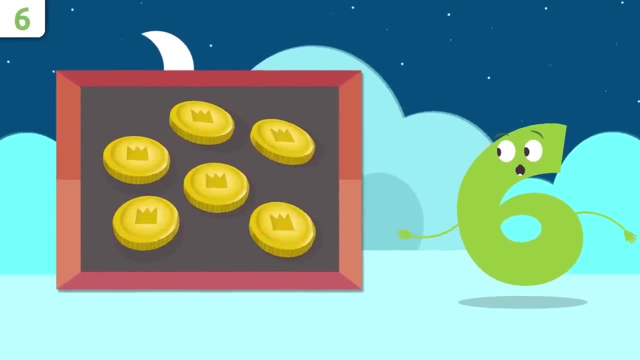 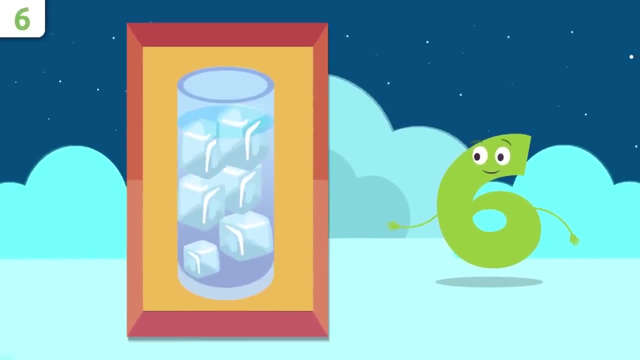 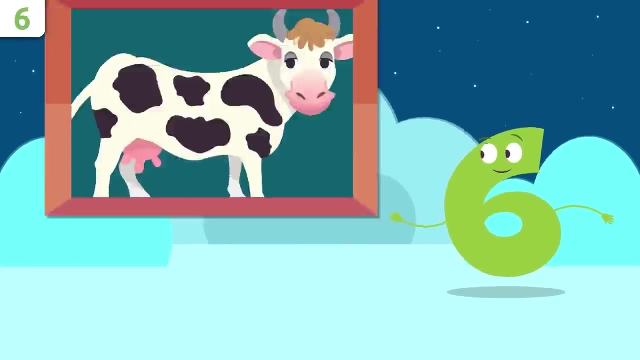 Four, Five And six. There are six coins. And how many ice cubes are there in this glass? One, Two, Three, Four, Five And six. There are six ice cubes. How many spots does this cow have? One. 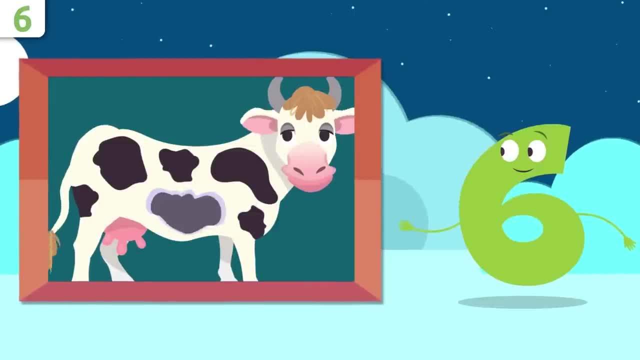 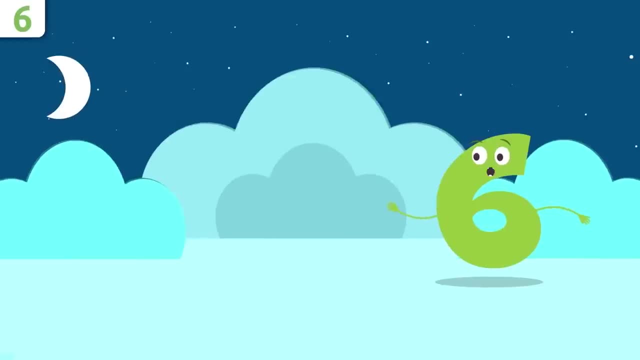 Two, Three, Four, Five And six. Our friend the cow has six spots Done. Do you want to sing with us later? We'll see you later in the ant hill. And how many ants are there in this ant hill? 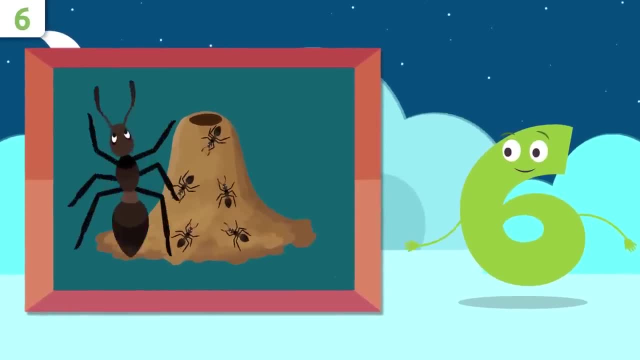 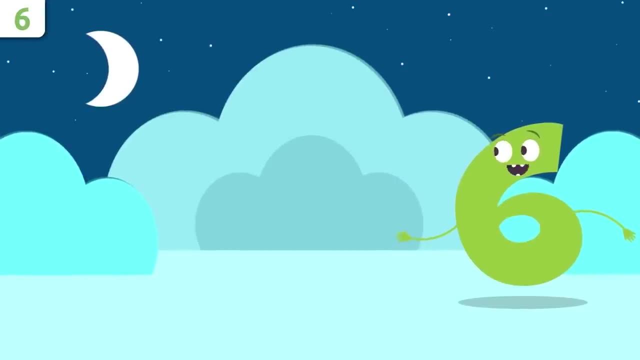 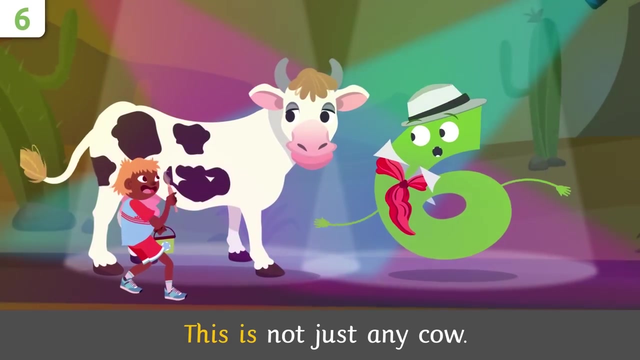 One, Two, Three, Four, Five And six. There are six ants. You did so well, my friends. Time to sing little cow. And how many are there in this ant hill? One, Two, Three, Four, Five. 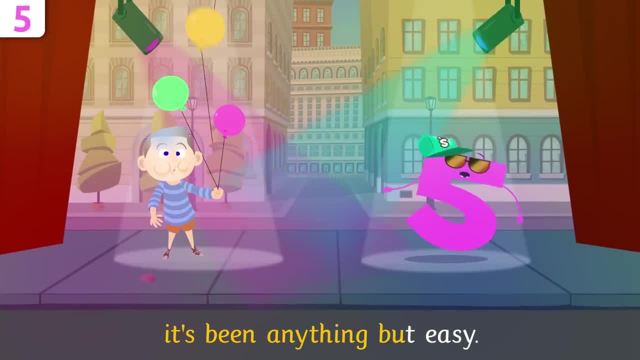 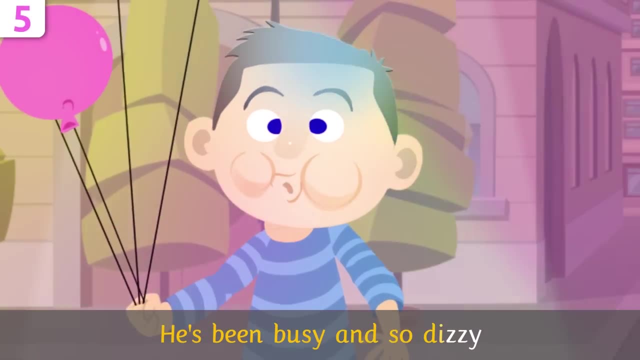 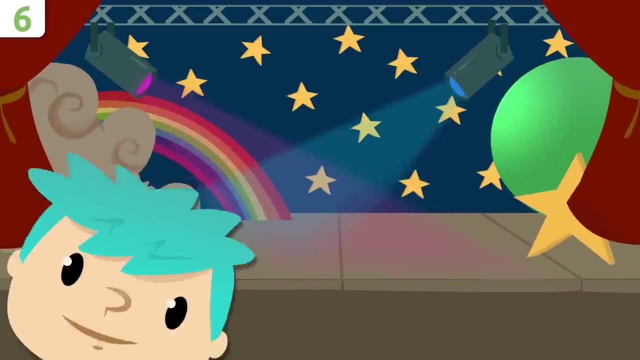 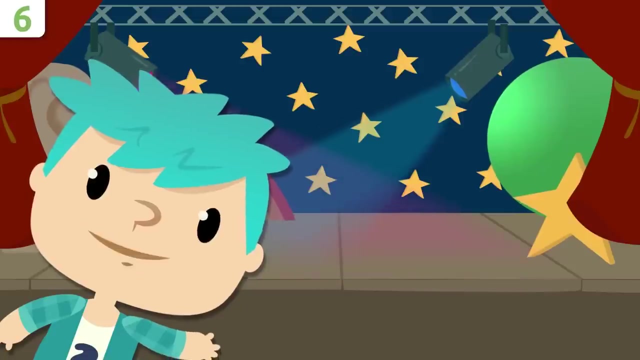 He's been busy and so dizzy, It's been anything but easy. Mike flew up many balloons. These five took him five afternoons. He's been busy and so dizzy, It's been anything but easy. Hello, hello, hello. Here we are again. Today I'll be introducing number six. 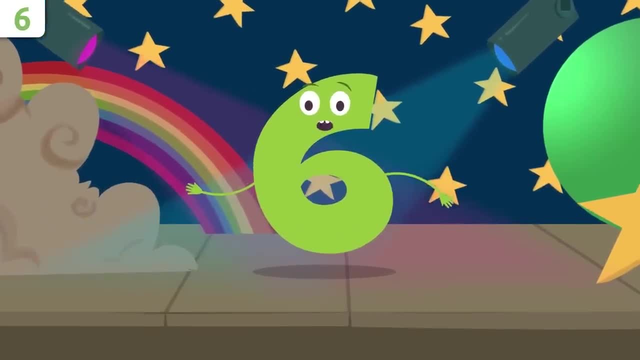 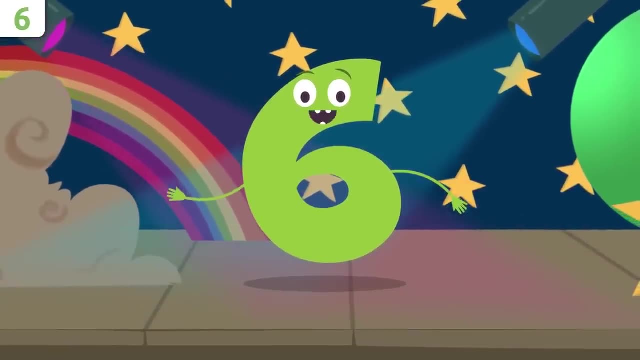 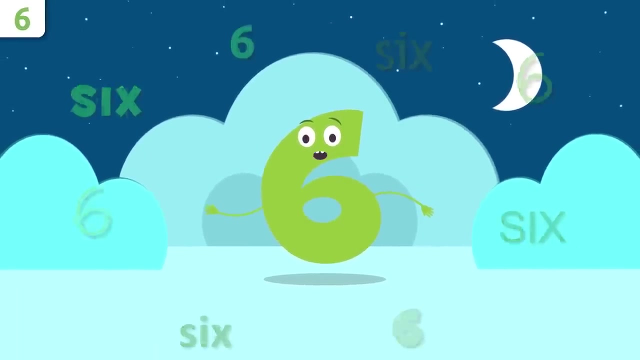 A very good morning to everyone. Do you know which number I am? I'm number six. Stay with me till the end. We have a song for you. Let's start with my name. Repeat after me: Six, Six Can hear you. 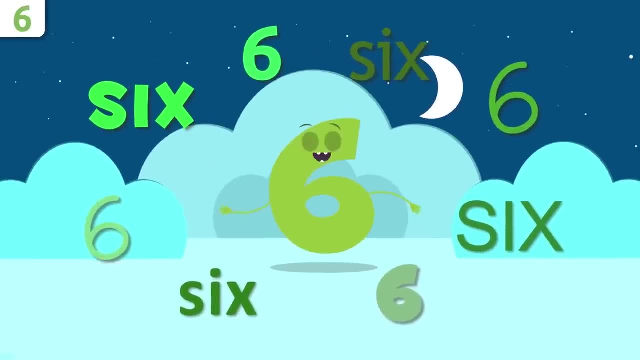 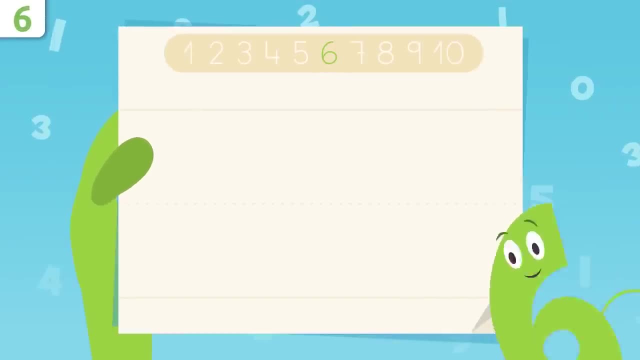 Six, Six, Excellent. Now I'll show you how to write number six. We start up here and trace down, drawing a curve. Now we trace like this, making a circle. You did great. Look, I look like a whistle. 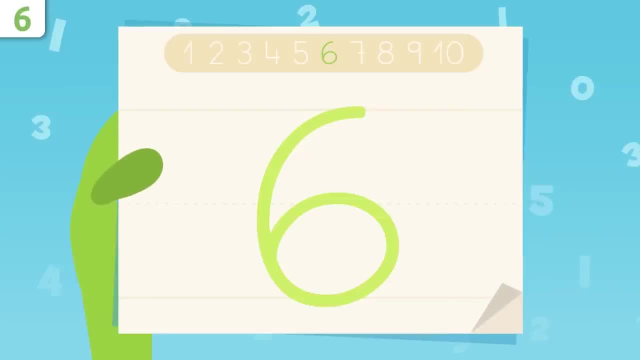 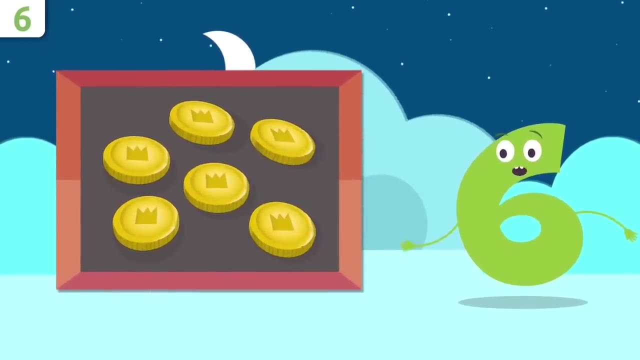 Try it at home using some paper and a pencil. It's easy. as pie, You did great. Let's try it as a young girl. JENNY Она, You're a great Percy Hi Showing off now. Do you have any compliments? 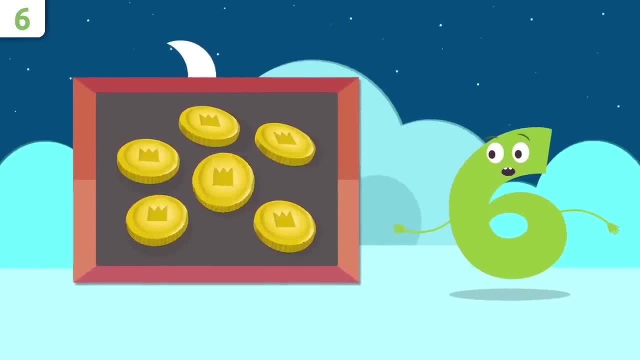 결혼이대. beating my keyboard can help you to get to move faster. Get faster or slow, Then you need to 2h without losing your balance. I tell you some tricks. Your eyes will kind of start polling when I read morepauses about this. 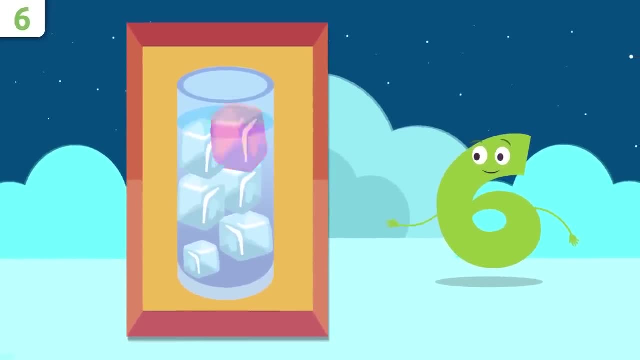 Let's see how I change you to be this disturbible eyes. How about? where are your records? laughing and looking forward the gonna even better. Did you want to look at some examples? Someone's dropped a few coins. How many are there? 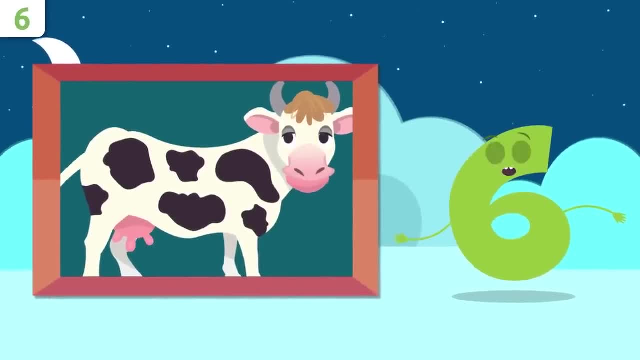 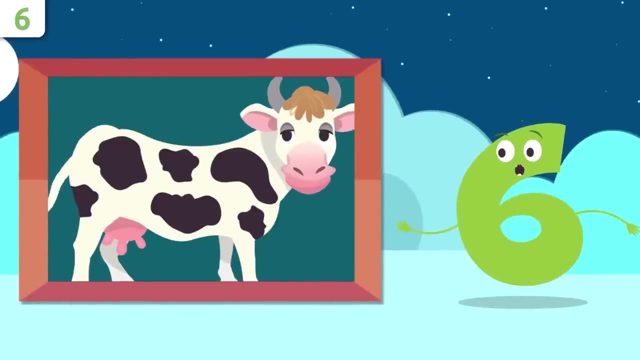 One, two, three, four, five and six. There are six coins. How many spots does this cow have? One, two, three, four, five and six. Our friend the cow has six spots. Do you wanna sing with us later? 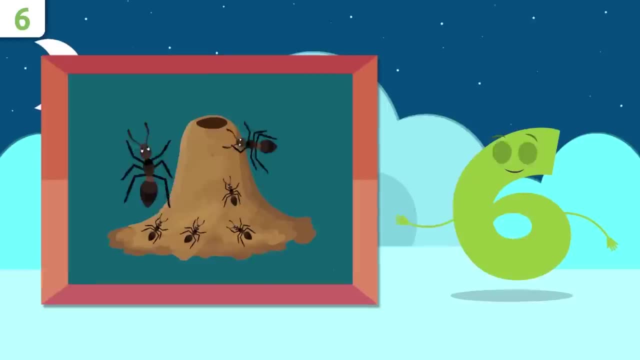 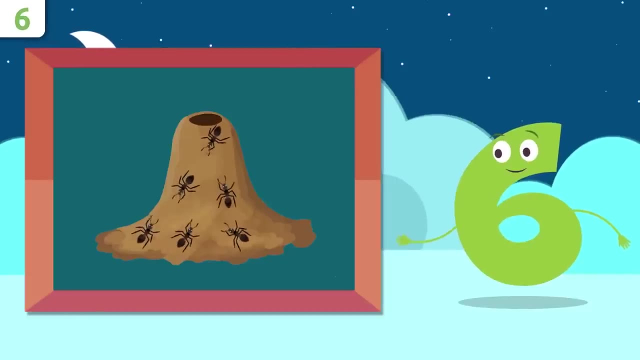 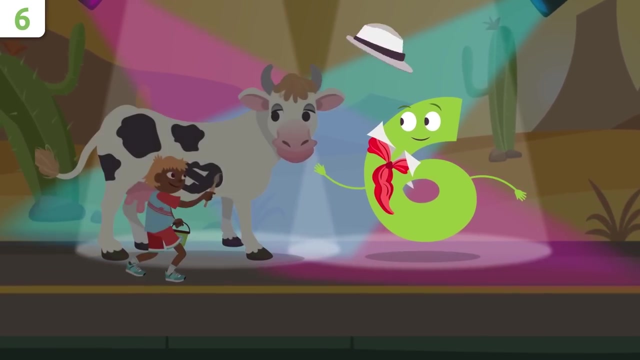 And how many ants are there in this ant hill? One, two, three, four, five and six. There are six ants. You did so well, my friends. Time to sing little cow. This is not just any cow. 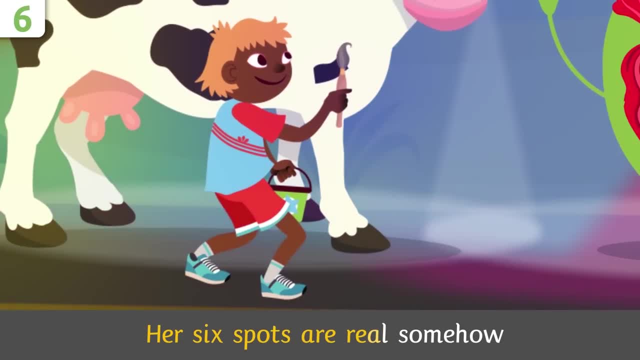 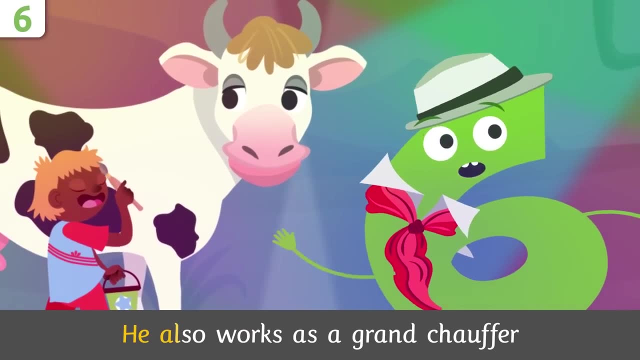 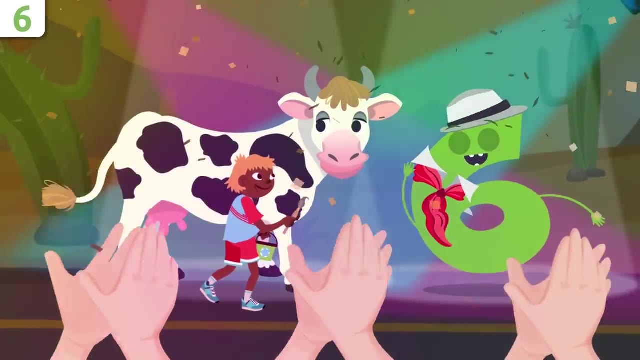 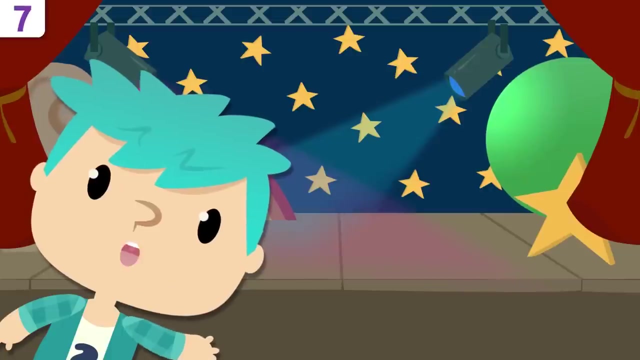 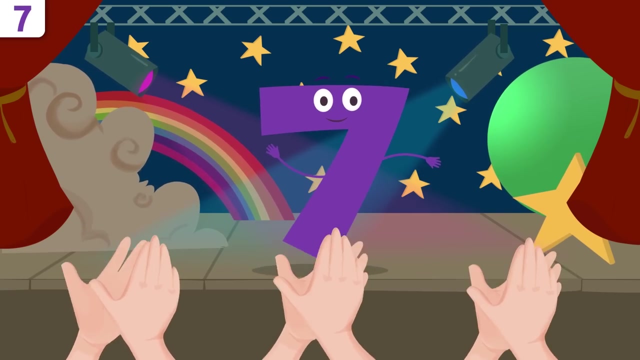 Her six spots are real. somehow A footballer painted them for her. He also works as a grand chauffeur. Good morning everyone. Let's give a huge welcome and a huge round of applause to my friend number seven, Howdy doody. 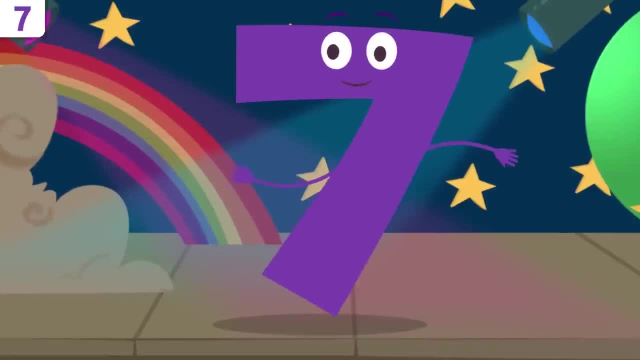 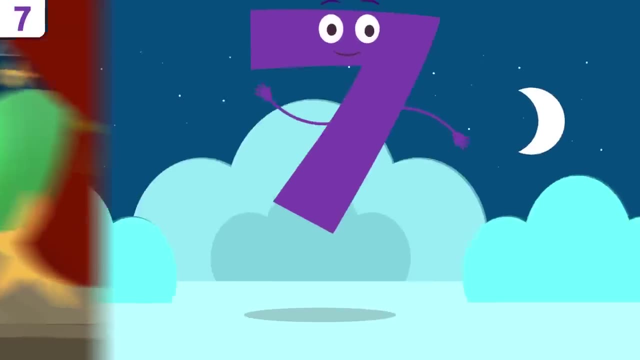 How are you doing? I'm number seven. I'm going to tell you a few things about me. Remember, I've got a song ready for you in the end. Don't go very far. Let's start saying my name. Repeat after me. 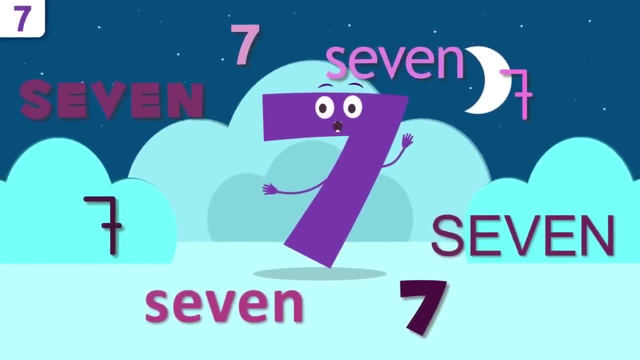 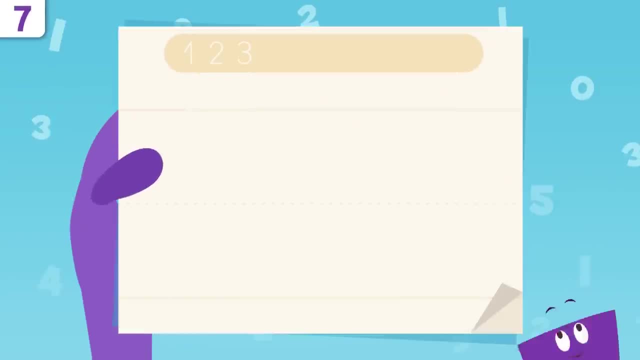 Seven, Seven- Can't hear you- Seven, Awesome. Do you want to learn how to write number seven? Don't miss any details. We start right here tracing a straight line. Now we draw a line all the way down. One more little line to go. 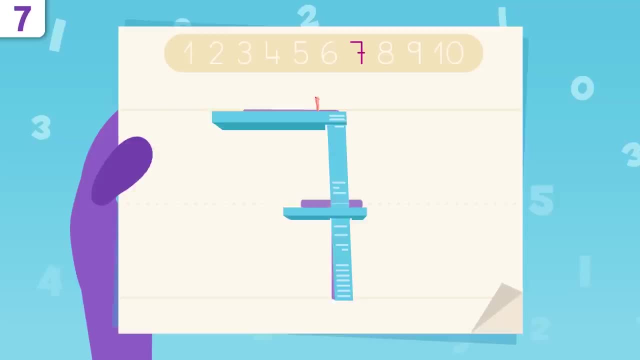 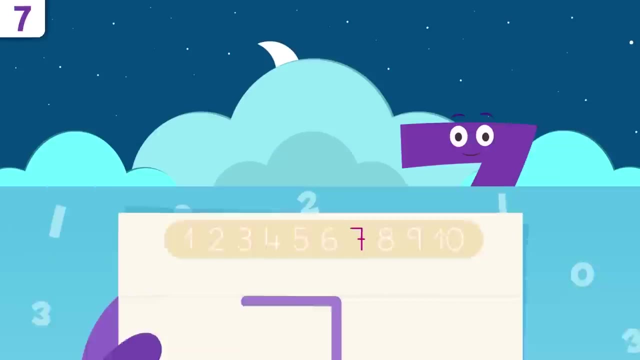 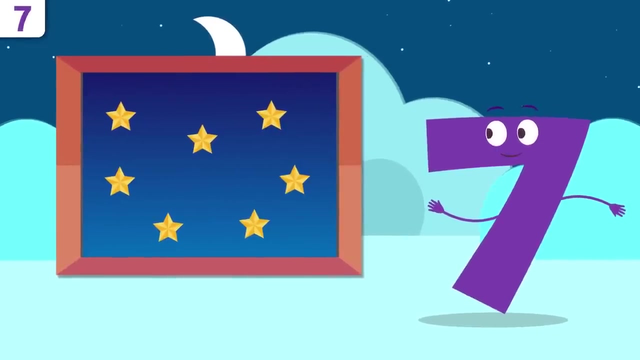 It goes right here. Try it at home using some paper and a pencil. Easy peasy, right? Do you want to look at some examples? Whoa the sky. How many stars can you count? One, two, three, four, five, six and seven. 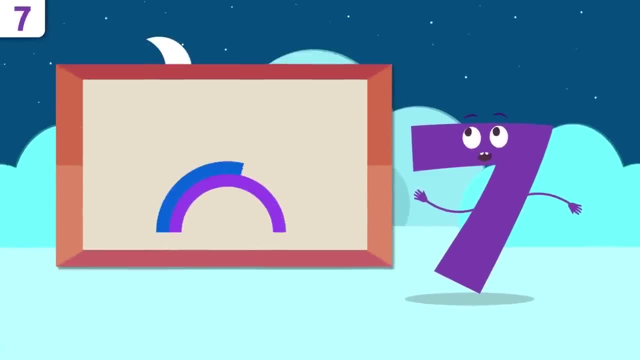 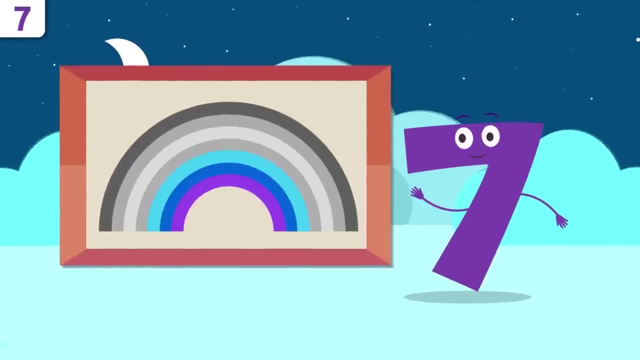 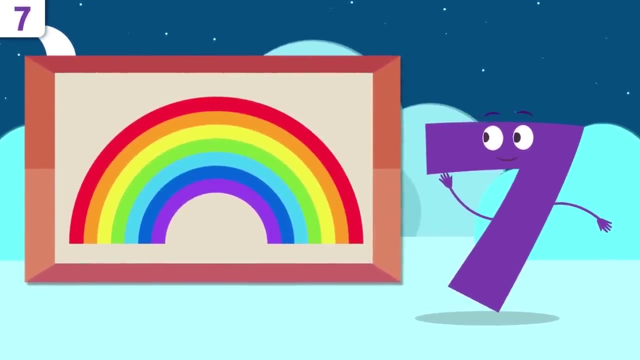 There are seven stars in the sky. Do you know how many colors there are in a rainbow? Let's see One, two, three, four, five, six, Four, five, six and seven. There are seven colors in the rainbow. 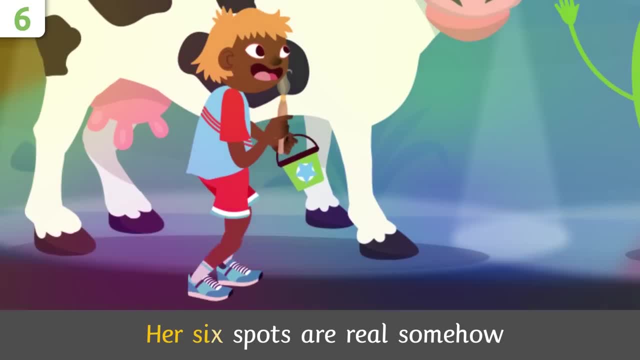 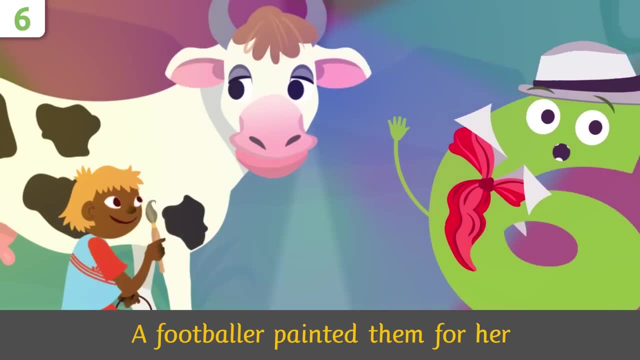 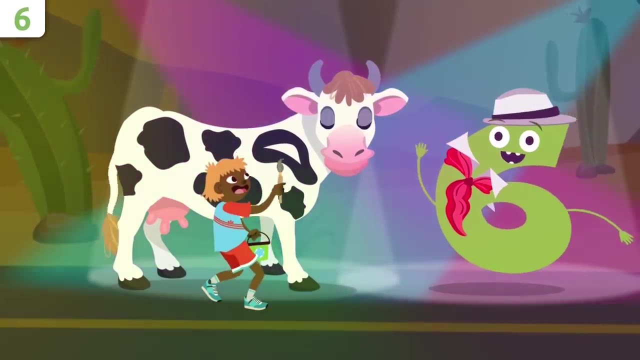 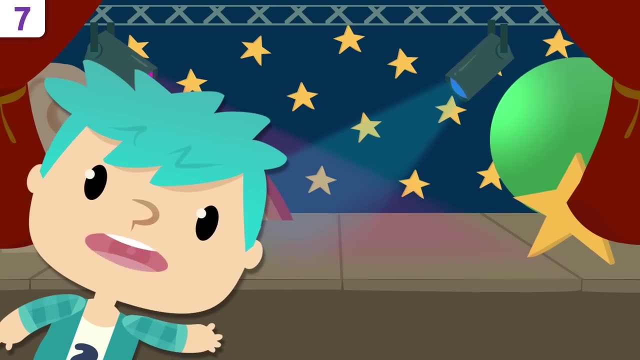 And six. There are six ants. You did so well, my friends. Time to sing little cow. This is not just any cow, somehow a footballer painted them for her. he also works as a grand chauffeur. good morning everyone. let's give a huge round of applause to my friend number seven. 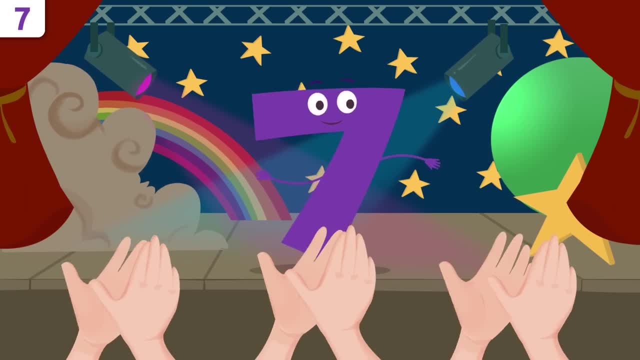 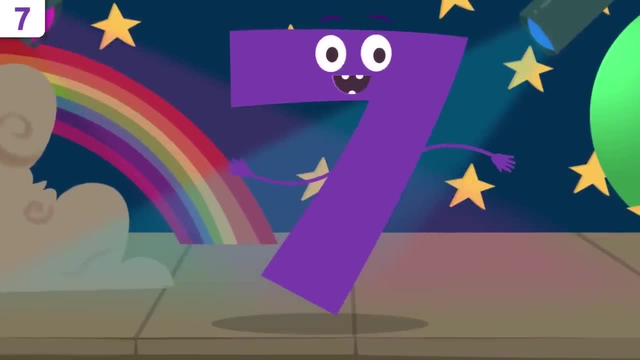 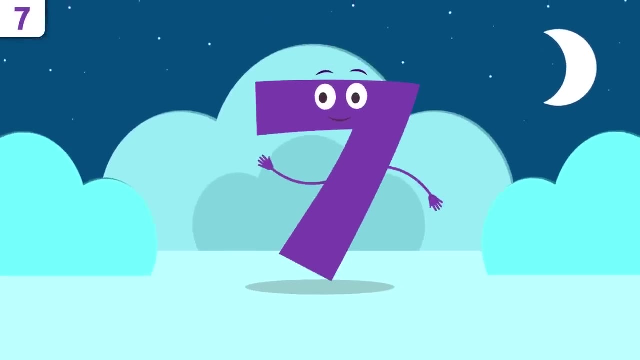 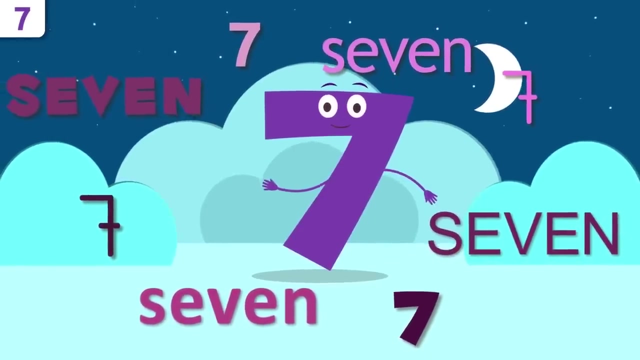 howdy, doody, how are you doing? i'm number seven. i'm going to tell you a few things about me. remember, i've got a song ready for you in the end. don't go very far. let's start saying my name. repeat after me: seven, seven, can't hear you. seven, awesome. 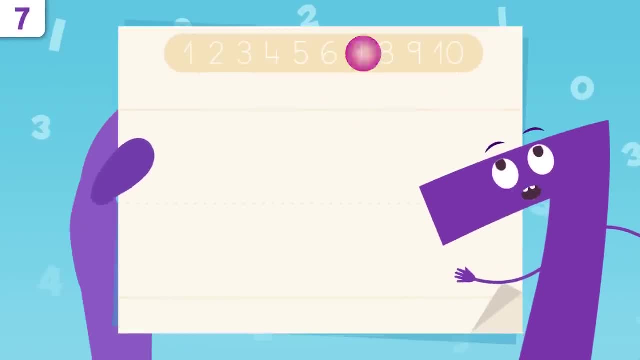 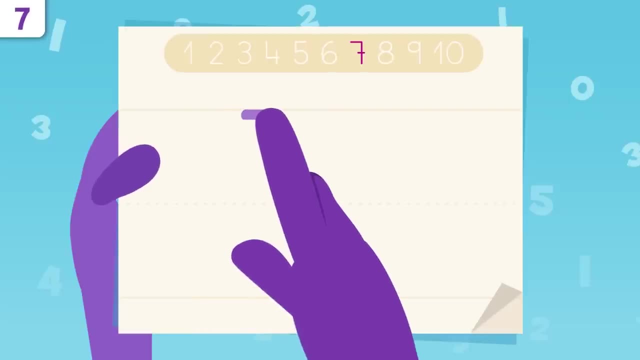 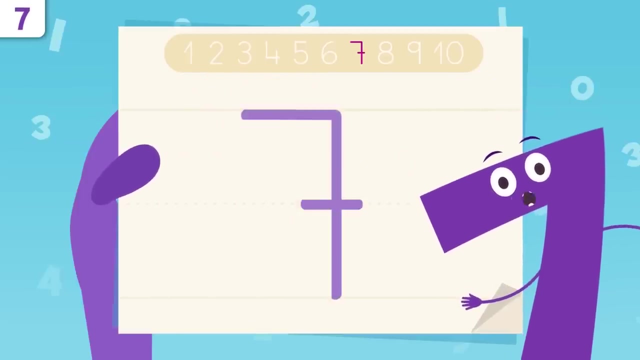 do you want to learn how to write number seven? don't miss any details. we start right here, tracing a straight line. now we draw a line all the way down. one more little line to go. it goes right here. try it at home using some paper and a pencil. easy peasy, right? do you want to look at some? 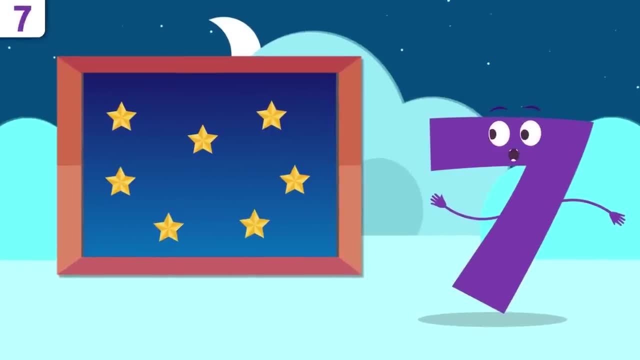 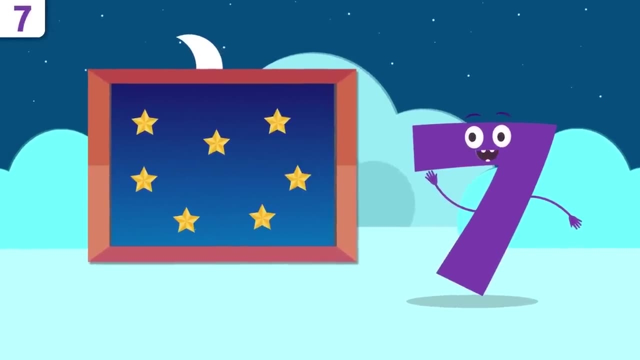 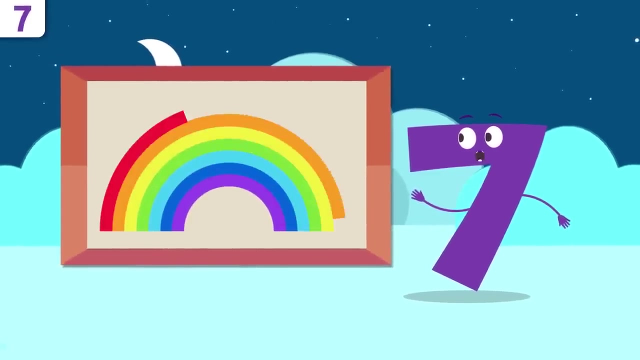 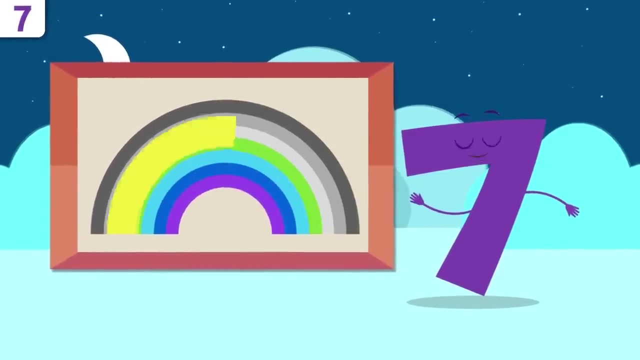 examples: whoa, the sky. how many stars can you count? one, two, three, four, five, six and seven? there are seven stars in the sky. do you know how many colors there are in a rainbow? let's see: one, two, three, four, five, six and seven. there are seven colors in the rainbow. 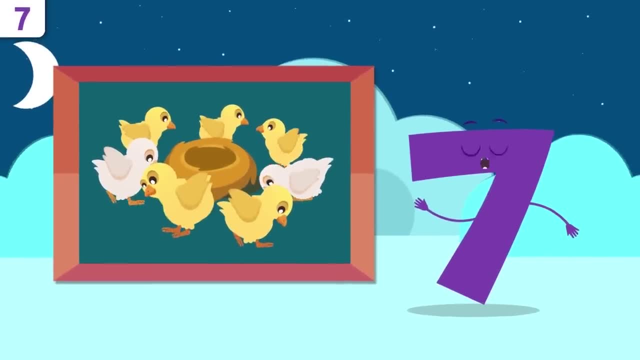 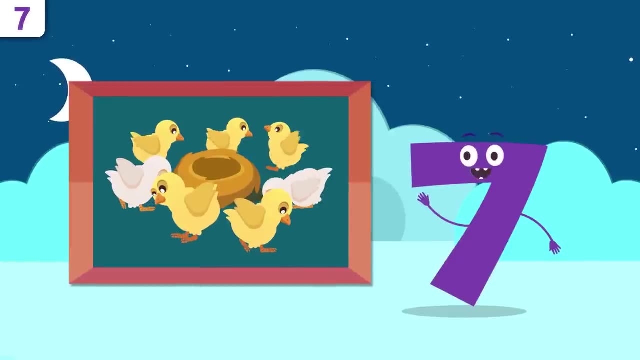 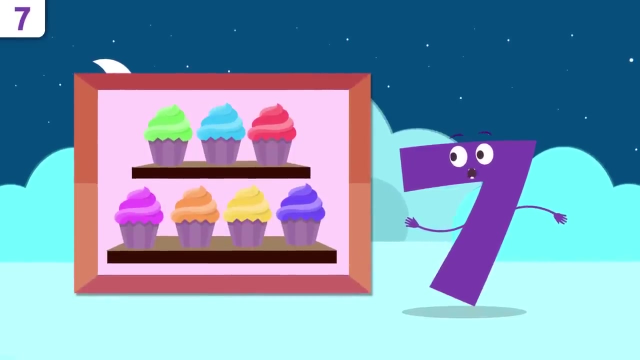 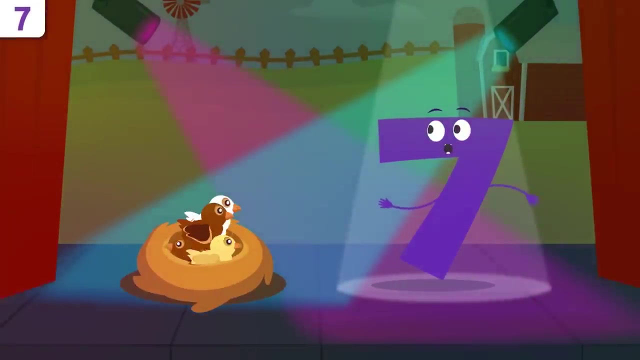 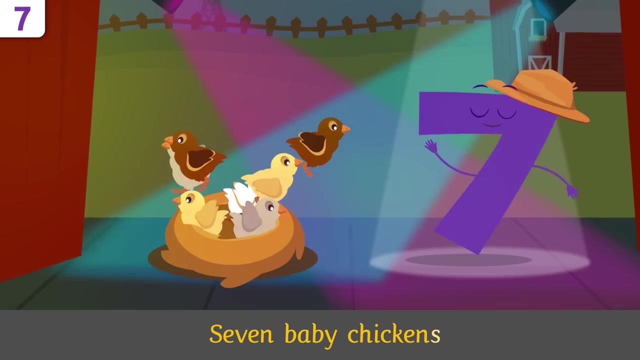 how many baby chickens are there? one, two, three, four, five, six and seven? there are seven baby chickens we're going to be singing later, friends, yum, cupcakes. how many are there? one, two, three, four, five, six and seven? there are seven cupcakes. way to go, friends, baby chickens, will you sing along with me? seven baby chickens in the nest. 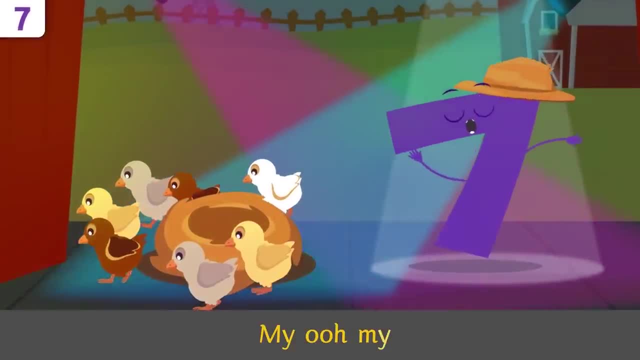 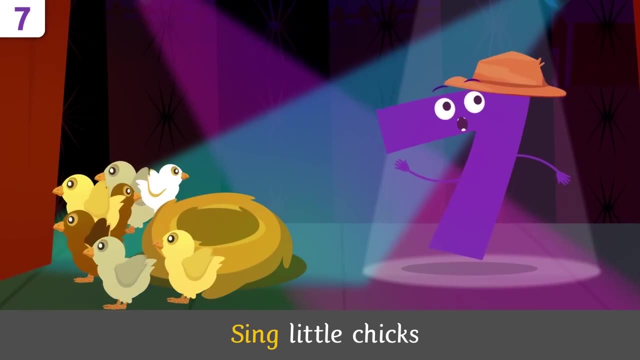 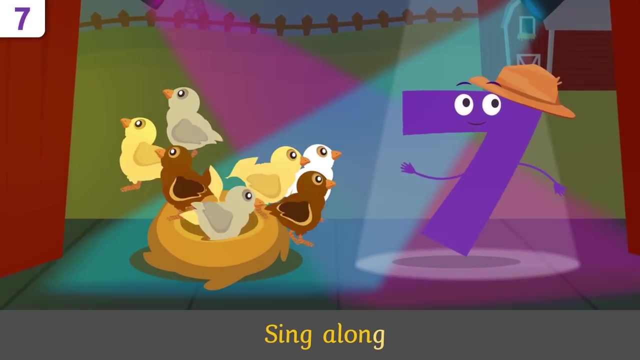 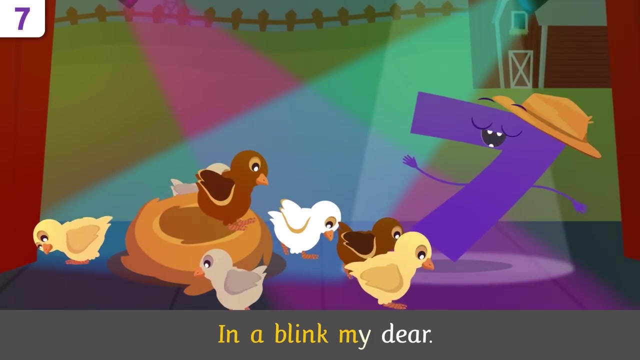 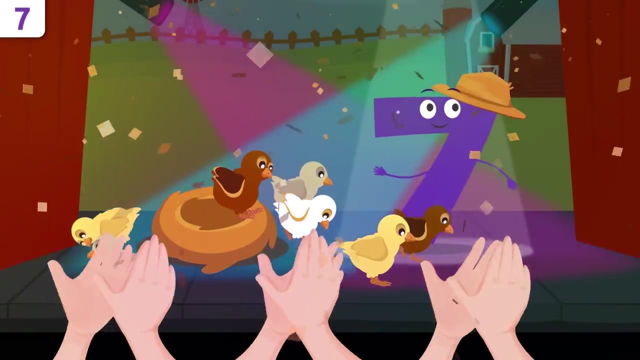 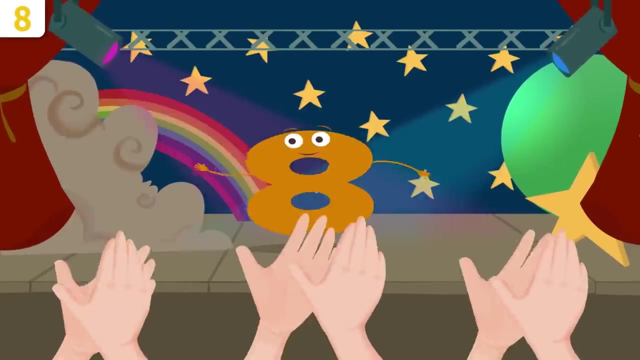 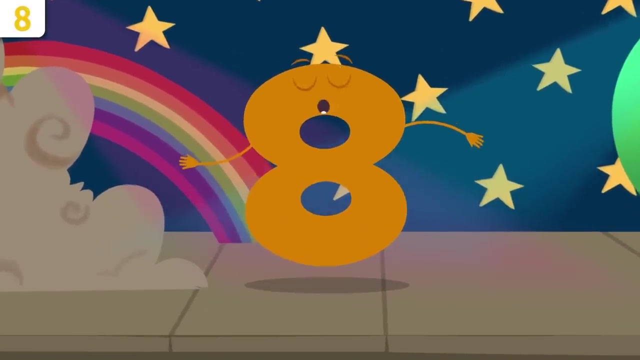 my, oh my. they look. they look so stressed. sing little cheeks, sing along, sing along, scare away your fear in a blink. my dear, here we are again, friends of numbers introducing number eight. hello everyone. do you know which number i am? you don't? i'm number eight. would you like me to tell you a few things about myself? 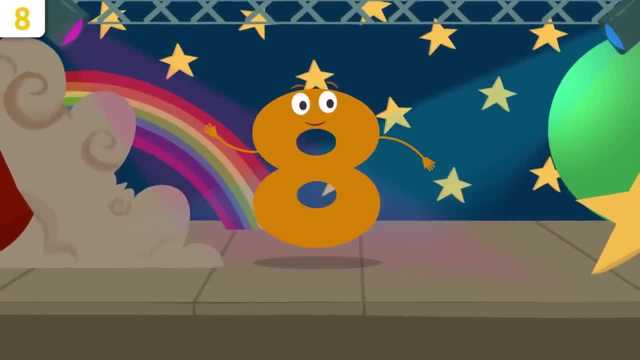 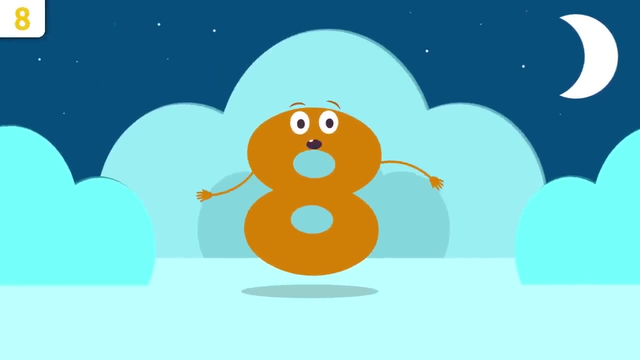 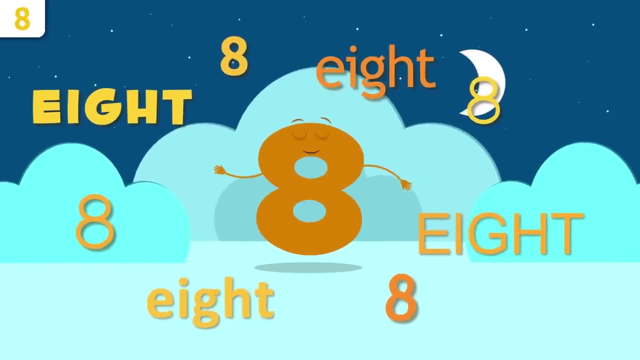 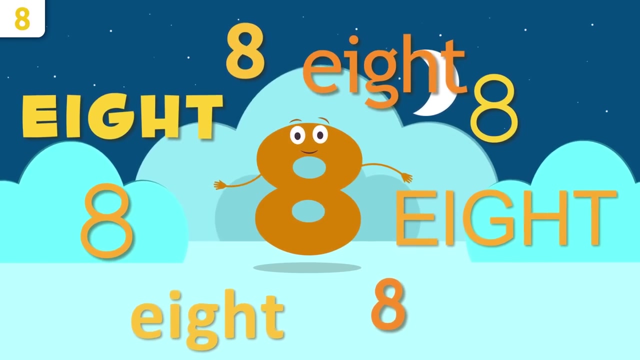 pay attention. oh, at the end of the video we're gonna be singing a song. you can't miss it. let's start with my name. repeat after me: eight, eight, much louder. eight, awesome. would you like me to show you how to write number eight? pay close attention. 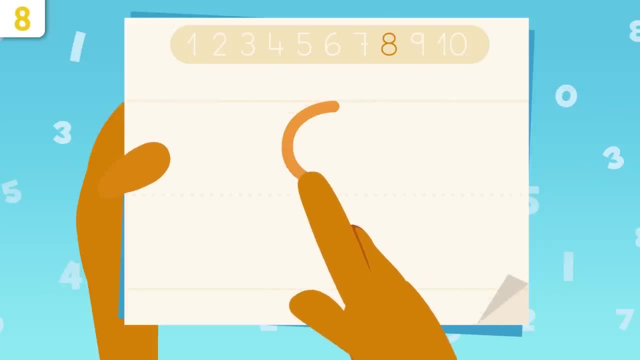 we're gonna start right here tracing a small curve and then another one. this way now we go all the way up tracing the same curves we did before. oh look, i look like two donuts. try it at home using some paper and a pencil. it's easy as pie. 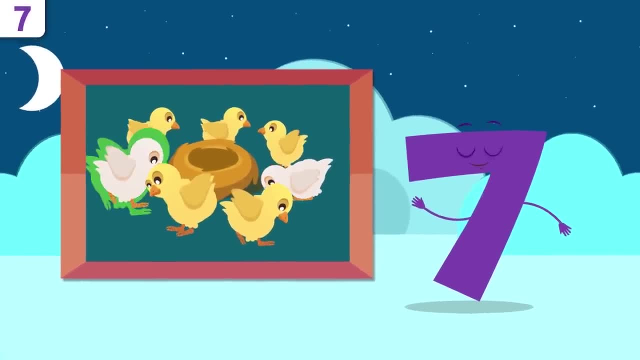 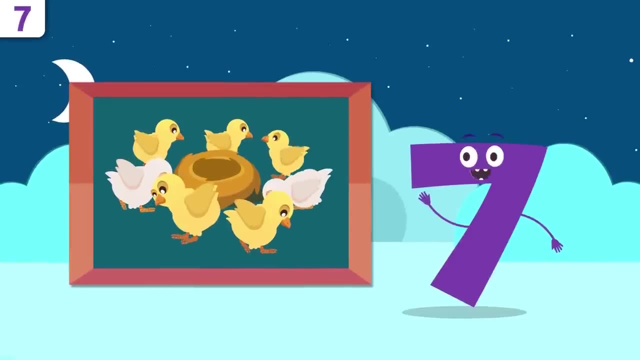 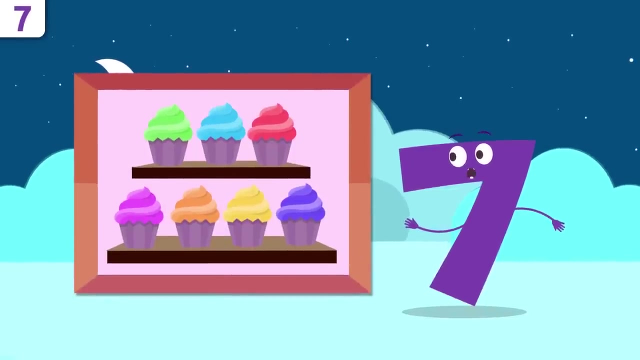 How many baby chickens are there? One, two, three, four, five, six and seven? There are seven baby chickens. We're going to be singing later: friends, Yum, cupcakes. How many are there? One, two, three, four, five, six and seven? 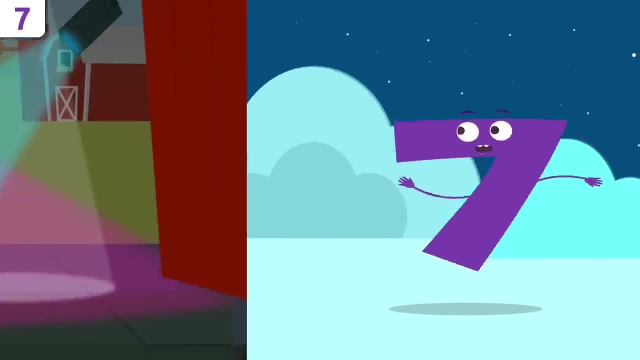 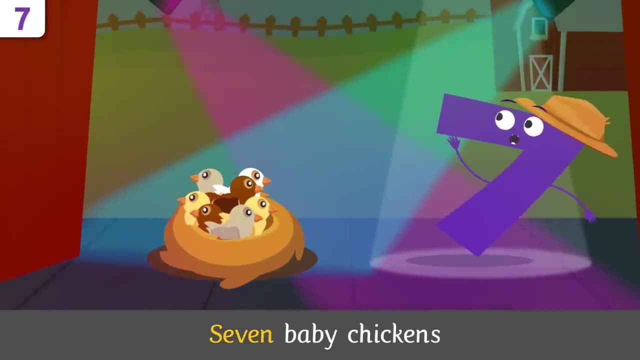 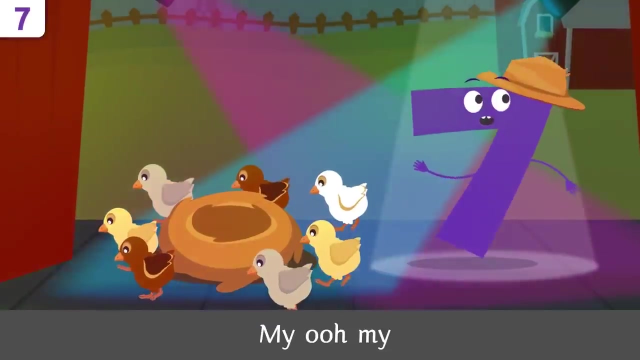 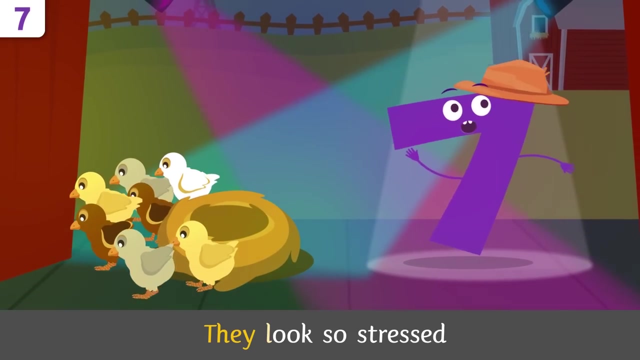 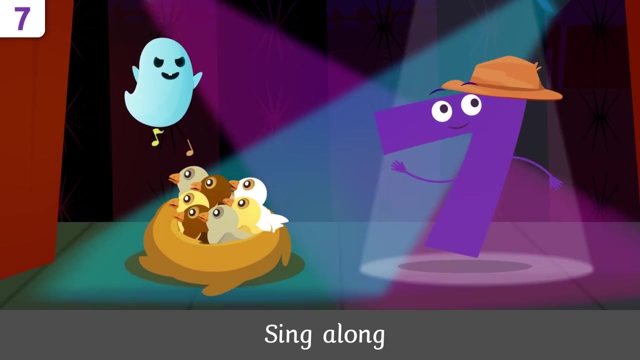 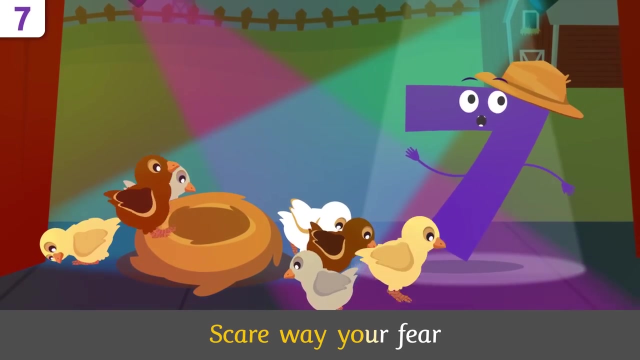 There are seven cupcakes. Way to go, friends. Baby chickens. will you sing along with me? Seven baby chickens in the nest. My, oh my, They look. They look so stressed. Sing, little chicks, Sing along, Scare away your fear. 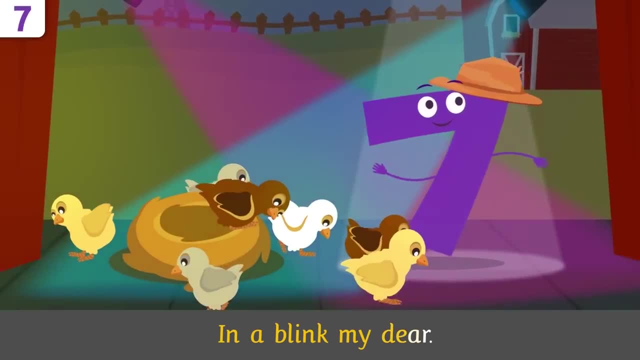 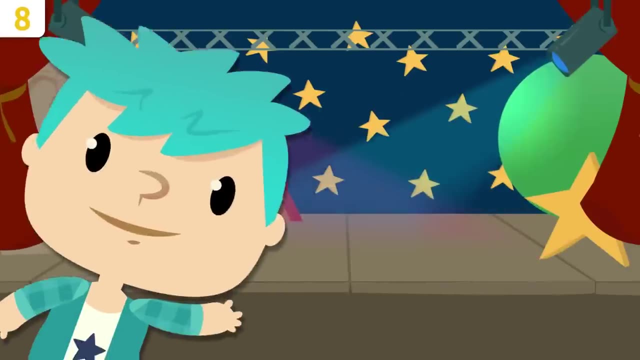 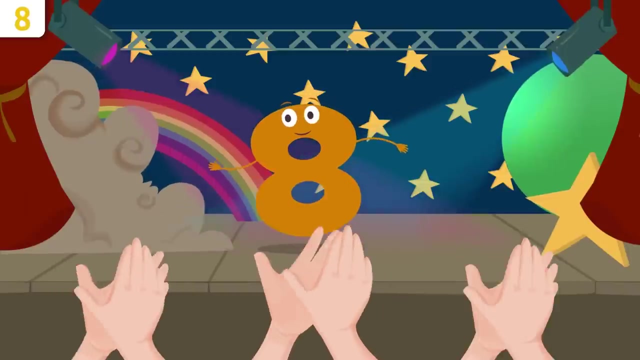 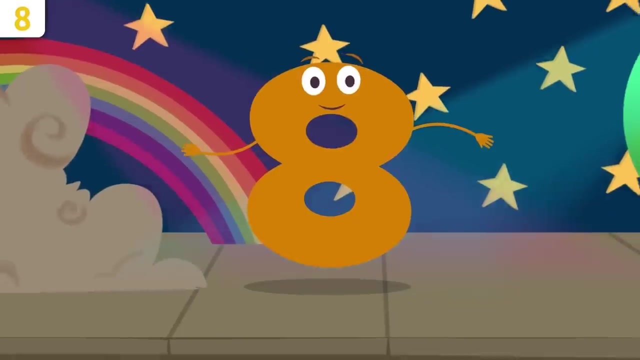 In a blink, my dear, Here we are again, friends of numbers. Introducing number eight. Hello everyone. Do you know which number I am? You don't. I'm number eight. Would you like me to tell you a few things about myself? 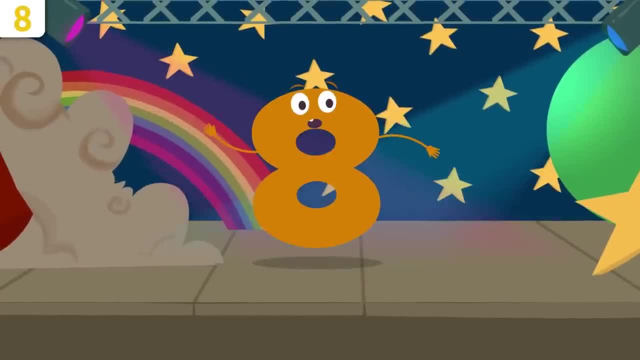 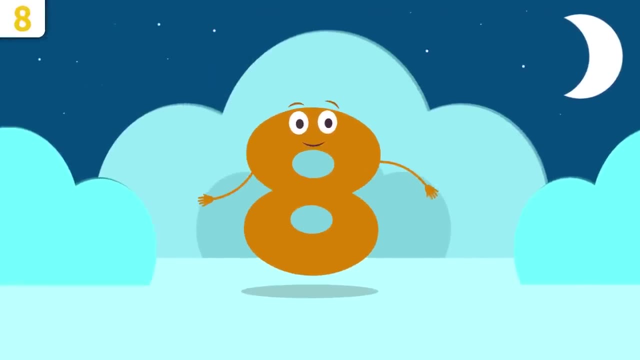 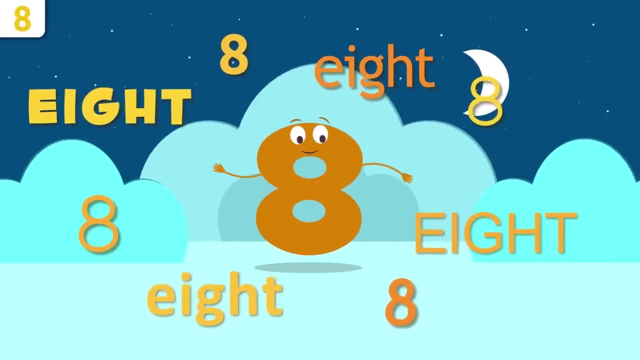 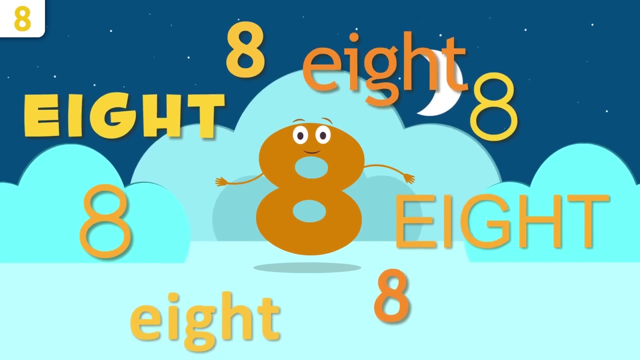 Pay attention. Oh, at the end of the video we're going to be singing a song. You can't miss it. Let's start with my name. Repeat after me: Eight, Eight, Much louder. Eight, Awesome. Would you like me to show you how to write number eight? 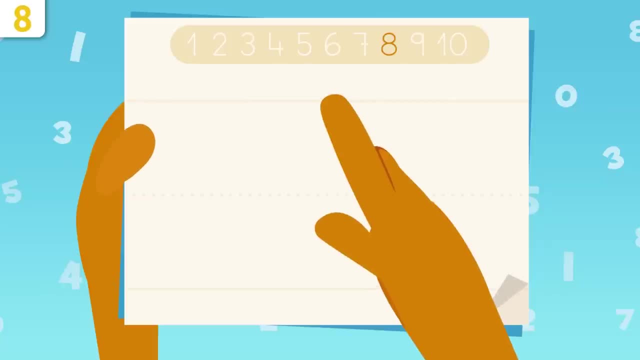 Pay close attention. We're going to start right here tracing a small curve and then another one. this way, Now we go all the way up tracing the same curves we did before. Oh look, I look like two donuts. 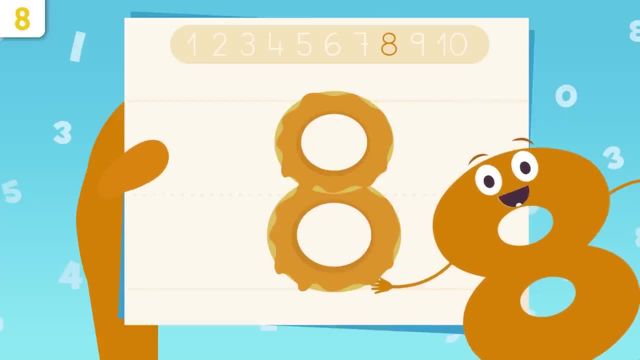 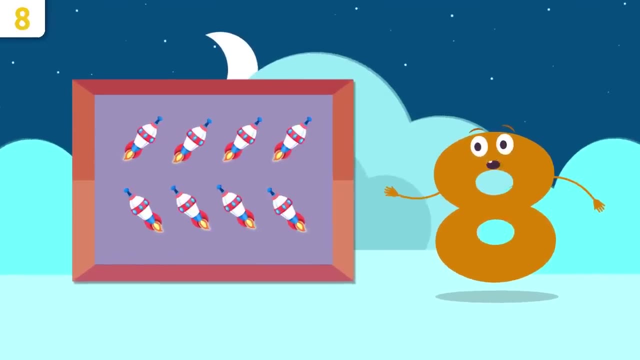 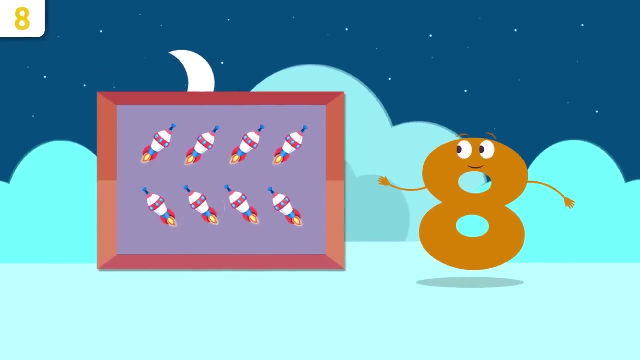 Try it at home using some paper and a pencil. It's easy as pie. Did you want to see some examples? Whoa spaceships. How many can you count? One, two, three, four, five, six, seven and eight? 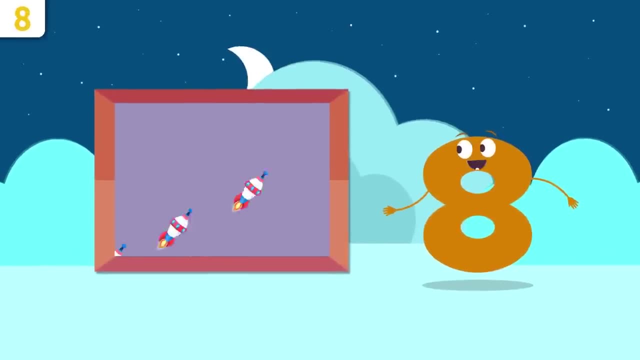 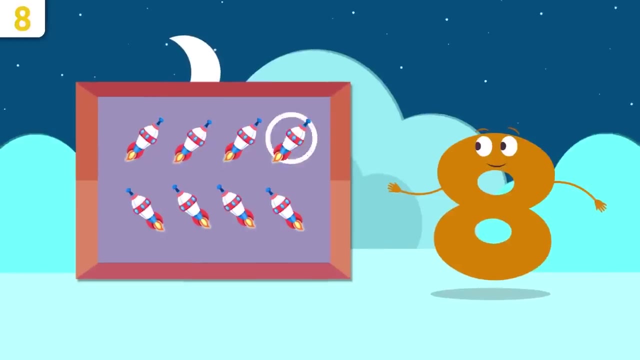 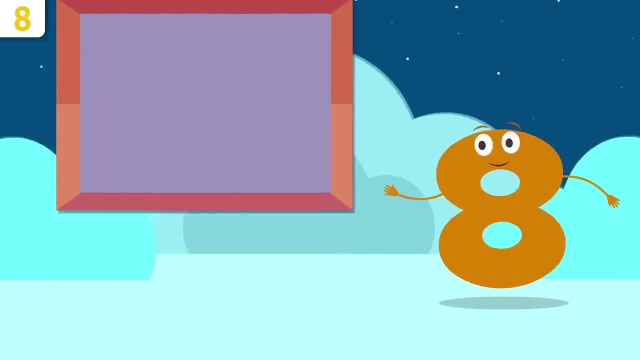 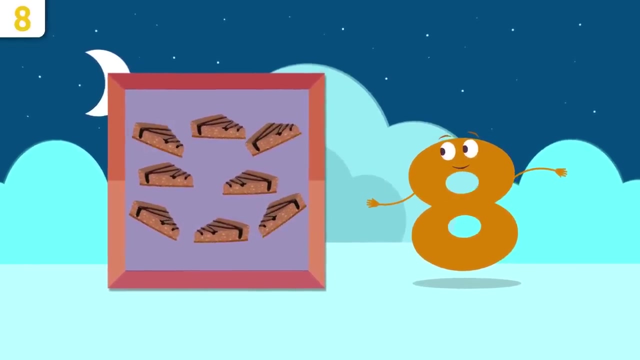 do you want to start? do you want to see some examples? whoa spaceships, how many can you count? one, two, three, four, five, six, seven and eight? there are eight spaceships. um yum cake. how many slices did we cut? one, two, three, four, five, six, seven and eight. there are. 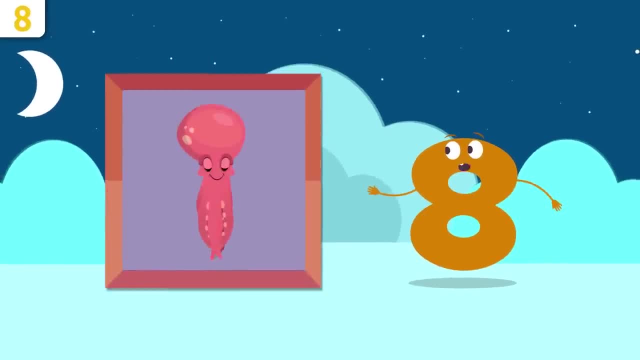 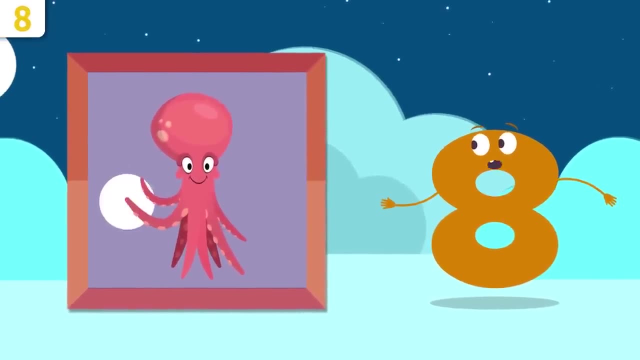 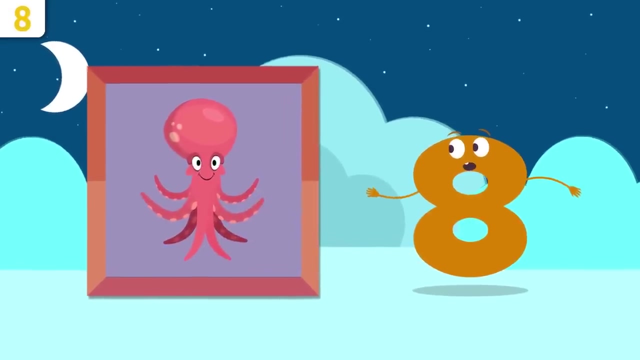 eight slices of cake. hey look, it's tom the octopus. hey there, buddy. how many arms does an octopus have? let's count them: one, two, three, four, five, six, seven and eight. tom the octopus has eight arms. don't go very far, tom. we'll be singing a song. 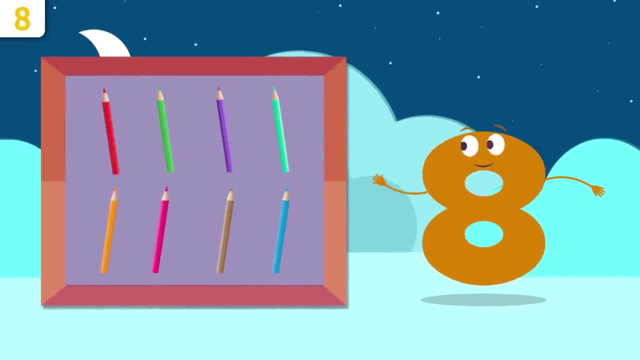 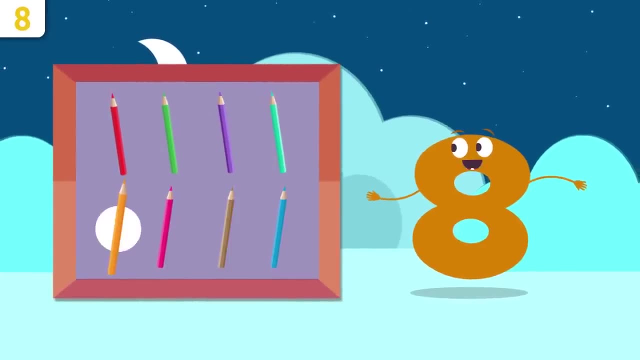 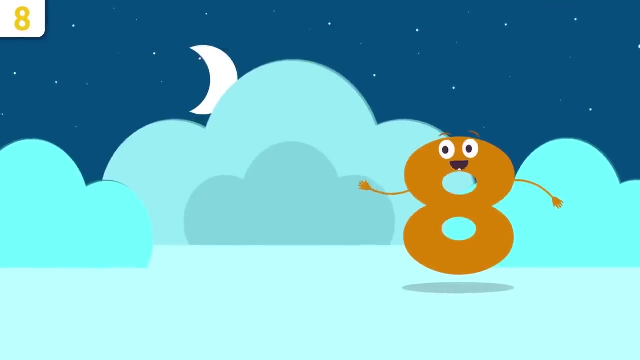 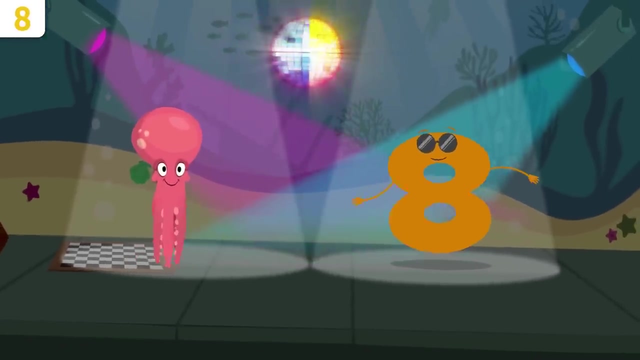 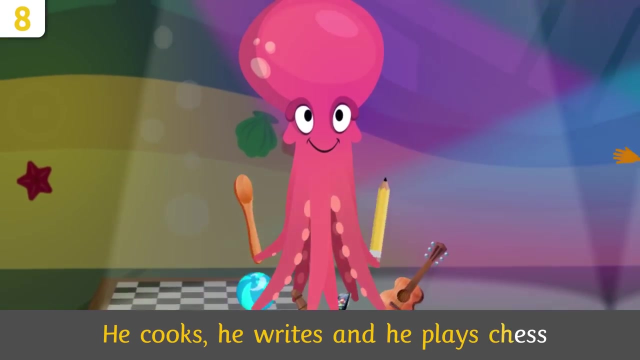 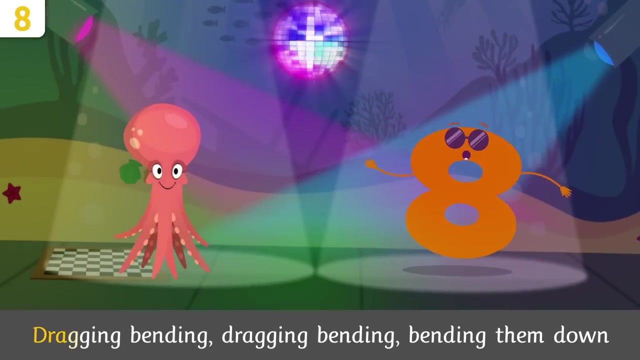 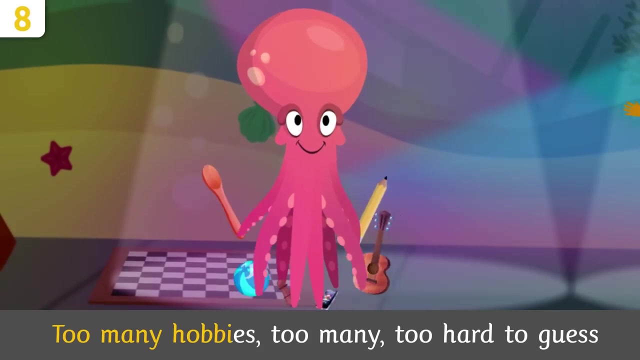 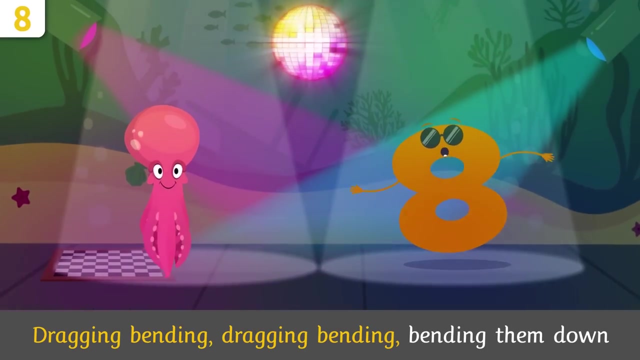 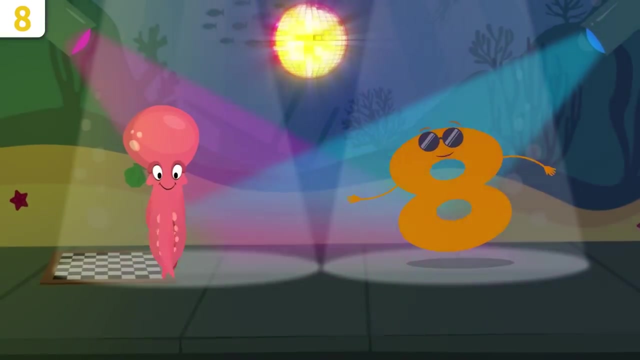 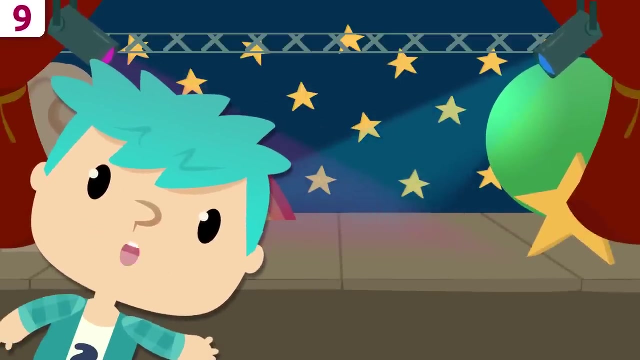 later color crayons. i love coloring. how many are there? one, two, three, four, five, six, seven and eight. there are eight color crayons. great job everyone. time to sing octopus time come along, so so, so so the so. good morning everyone. let's give a huge round of applause to my friend number nine. 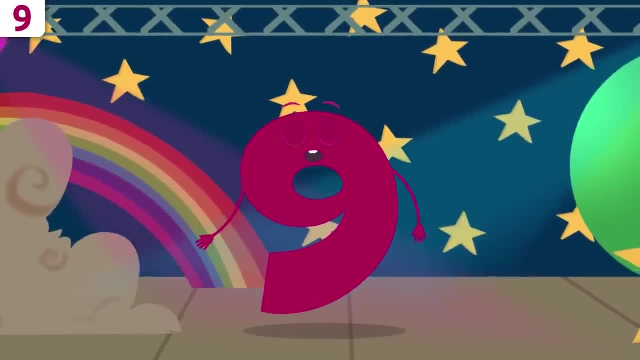 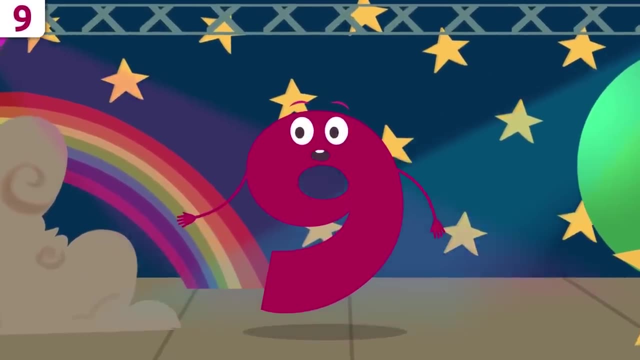 that's right. little buddies, it's me number nine. today i'll be telling you a few things about myself. how would you like that? At the end of the video we'll be singing a song. You don't want to miss that. Let's start with my name. 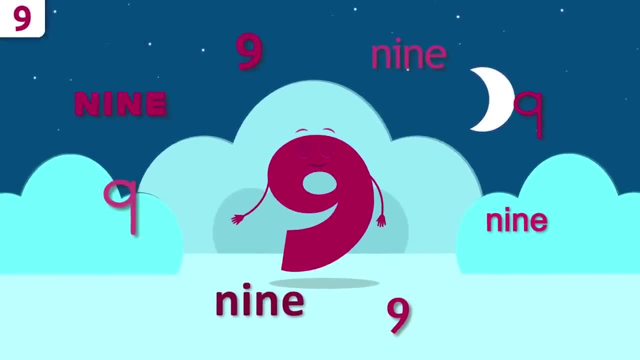 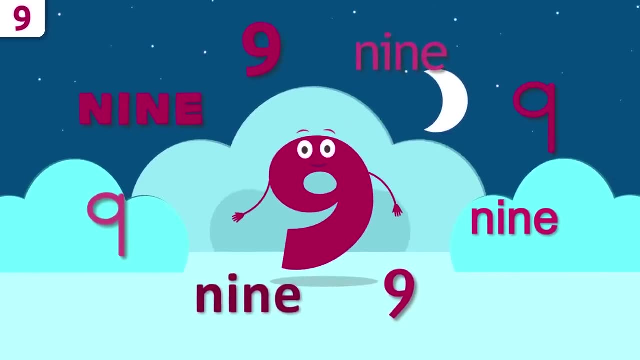 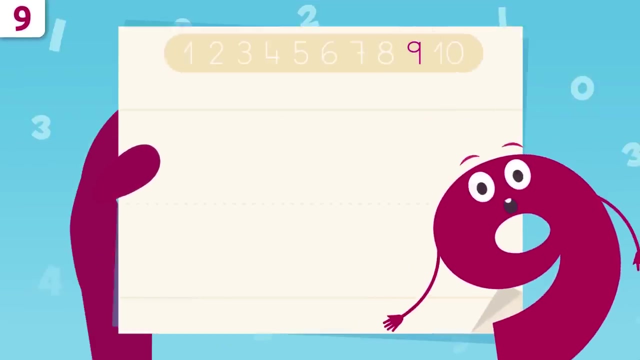 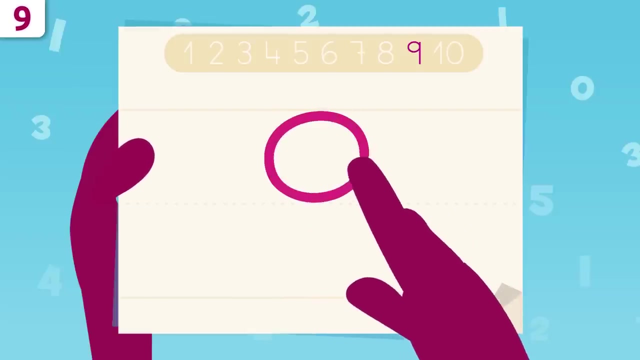 Repeat after me: Nine, Nine, Can't hear you. Nine, Awesome, Now I'm going to show you how to write number nine. We're going to start right here and we'll trace a circle. When we get here, we'll trace a vertical line all the way down. 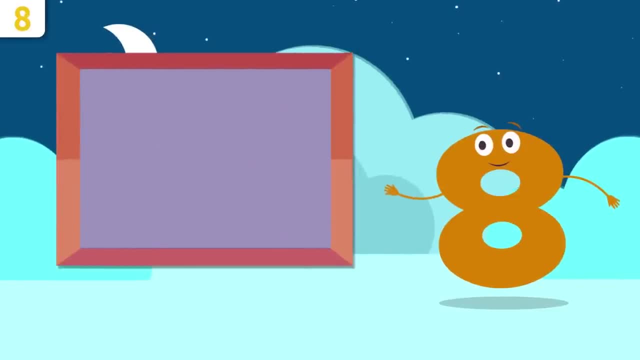 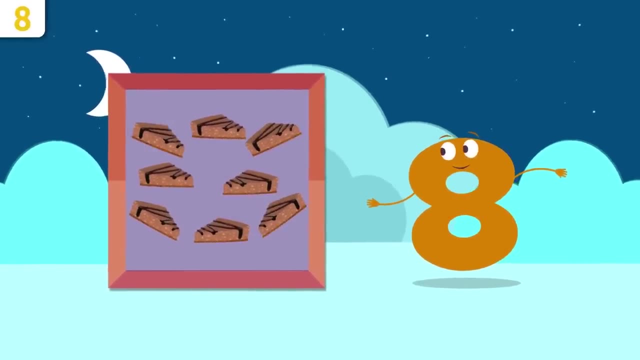 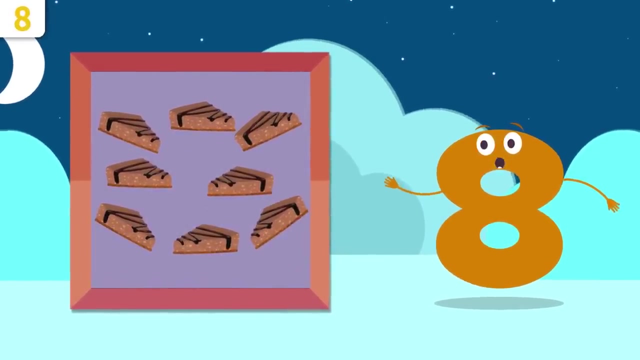 There are eight spaceships. Mm yum Cake. How many slices did we cut? One, two, three, four, five, six, seven and eight. There are eight slices of cake. Hey look, It's Tom the octopus. 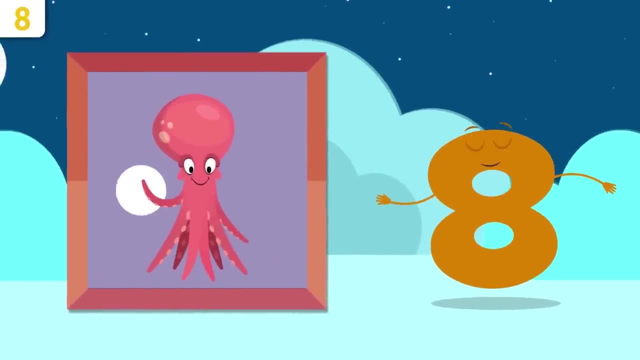 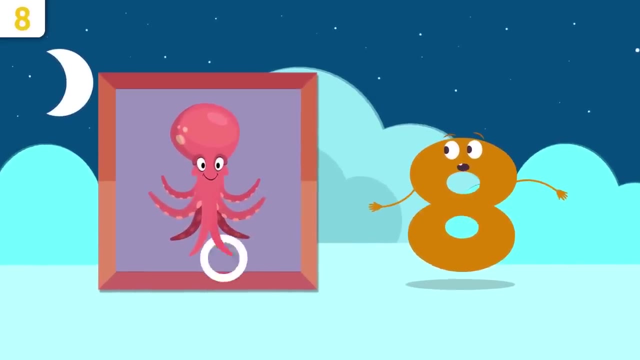 Hey there, buddy. How many arms does an octopus have? Let's count them: One, two, three, four, five, six, seven and eight. Tom, the octopus has eight arms. Don't go very far, Tom. 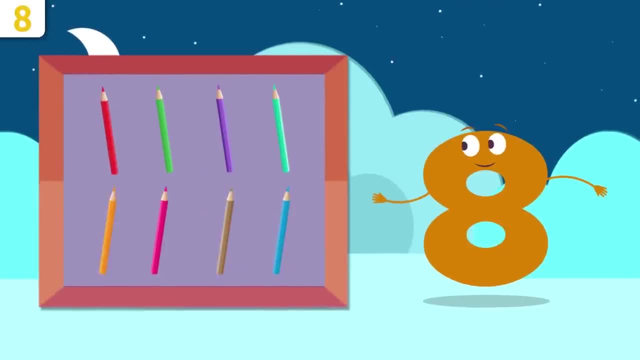 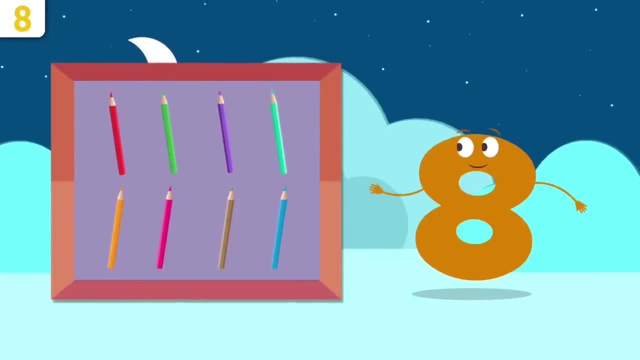 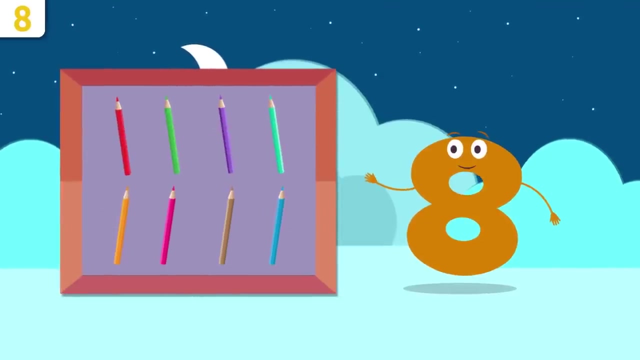 We'll be singing a song later. Color crayons. I love coloring. How many are there? One, two, three, four, five, six, seven and eight? There are eight color crayons. Great job everyone. Time to sing. 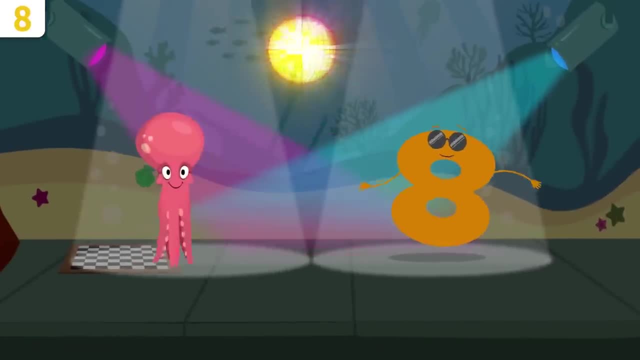 Octopus Tom. come along, He cook, he write and he play chess. Too many hobbies, too many, too hard to guess. His eight arms move so quickly around Draggin' bendin' draggin' bendin' bendin' them down. 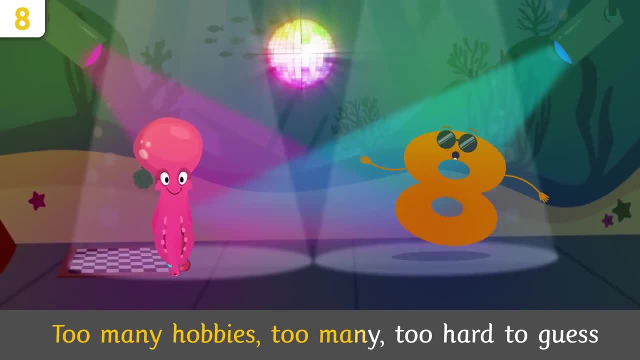 He cook, he write and he play chess. Too many hobbies, too many, too hard to guess. His eight arms move so quickly around Draggin' bendin' draggin' bendin' bendin' them down. He cook, he write and he play chess. 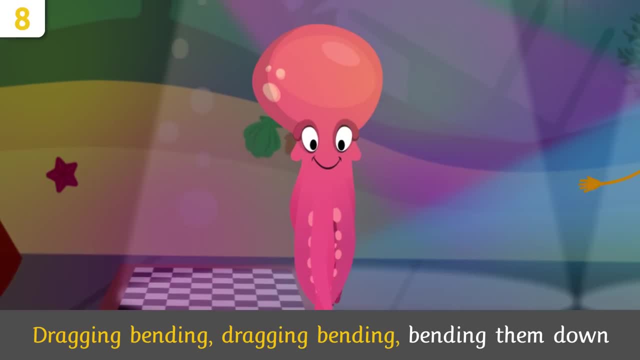 Too many hobbies too many, too hard to guess. His eight arms move so quickly around, Draggin' bendin', draggin' bendin' bendin' them down. He cook, he write and he play chess. Too many hobbies, too many, too hard to guess. 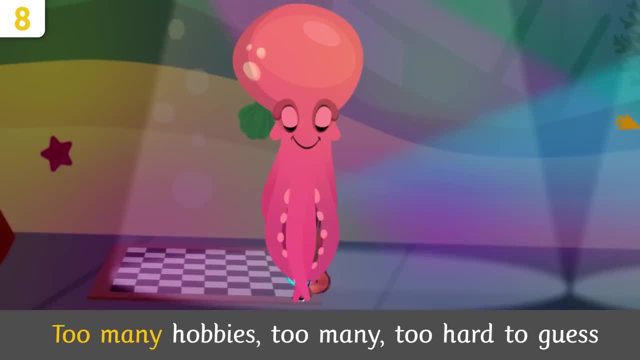 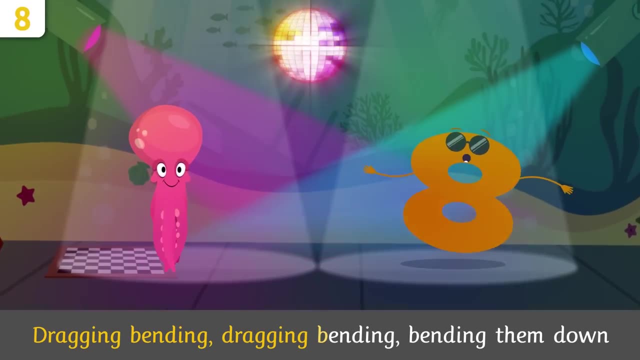 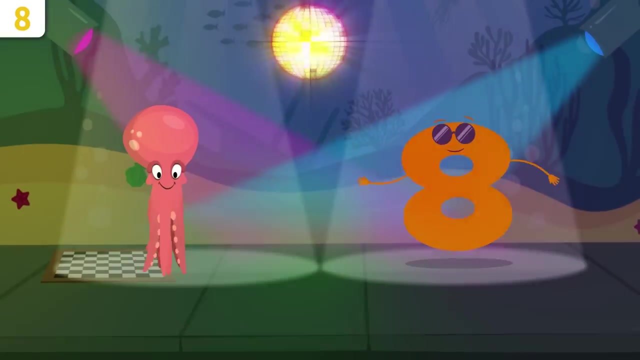 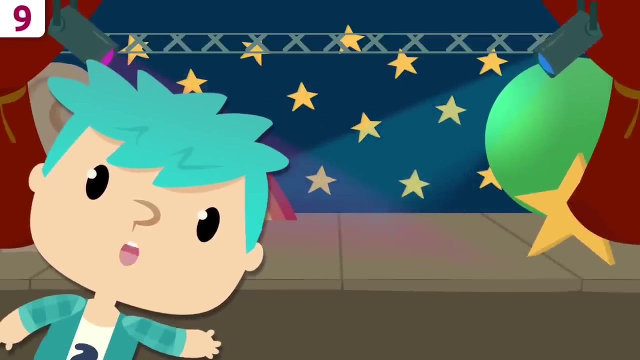 His eight arms move so quickly around. And he played chess. too many hobbies, too many, too hard to guess. His eight arm move so quickly around, Dragging, bending, dragging, bending, bending him down. Good morning everyone. Let's give a huge round of applause to my friend number nine. 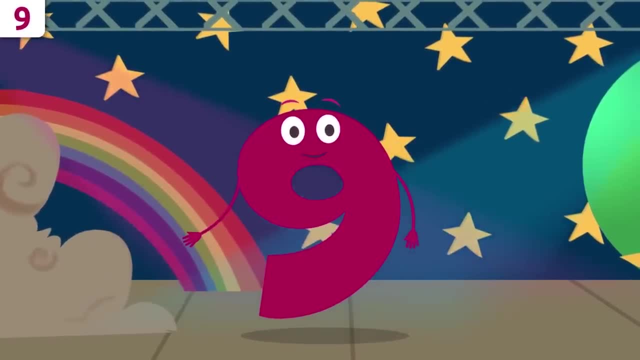 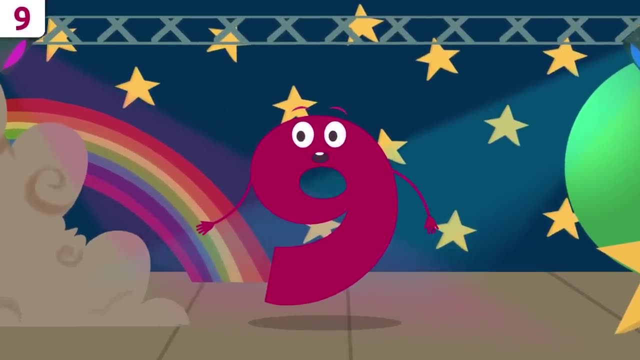 That's right. little buddies, it's me number nine. Today, I'll be telling you a few things about myself. How would you like that? At the end of the video we'll be singing a song. You don't want to miss that. 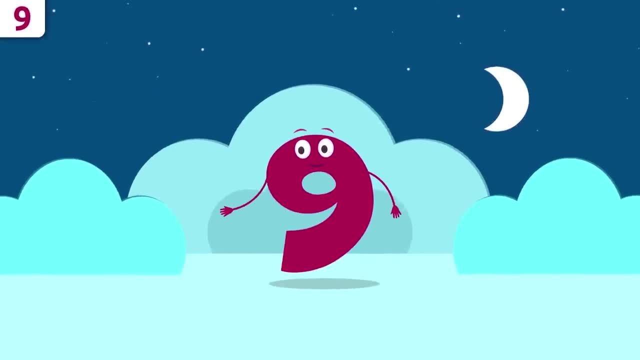 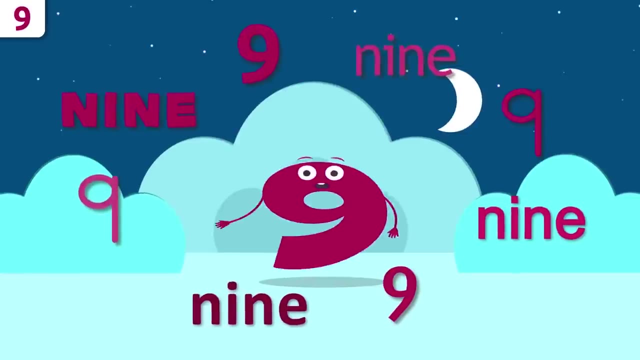 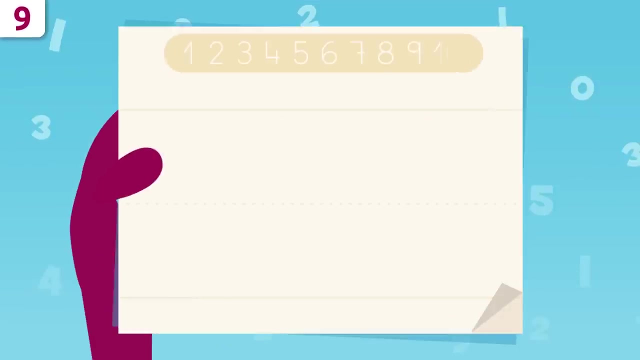 Let's start with my name. Repeat after me: Nine, Nine, Can't hear you. Nine, Awesome. Now I'm going to show you how to write number nine. We're going to start right here and we'll trace a circle. When we get here, we'll trace a vertical line all the way down. 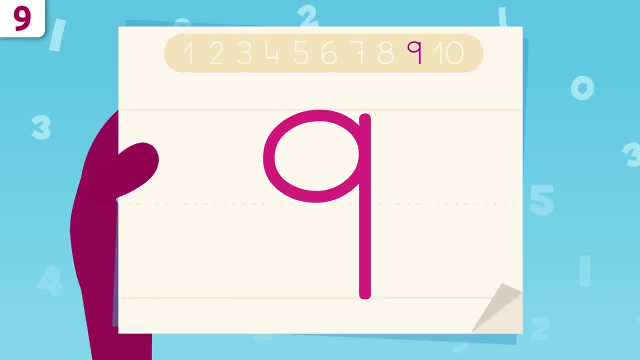 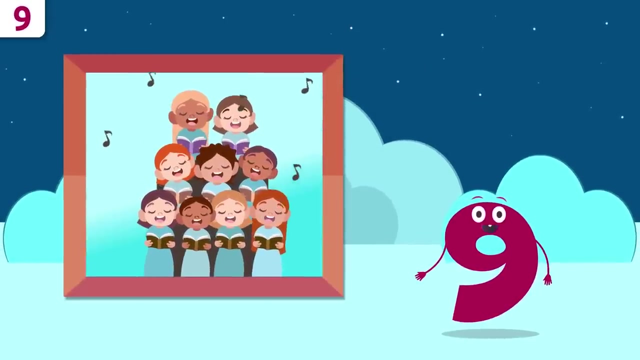 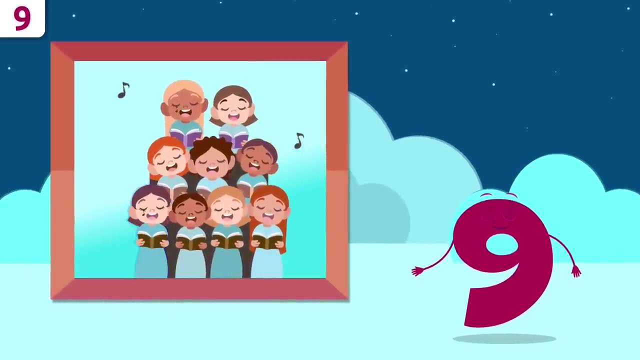 And this is number nine. Oh look, I look like a cowboy lasso. Try it at home using some paper and a pencil. Would you like to look at some examples? Whoa, It's a choir. How many singers are there? One, two, three, four, five, six, seven, eight and nine. 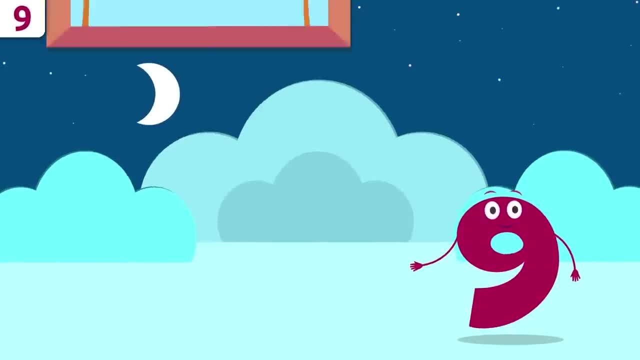 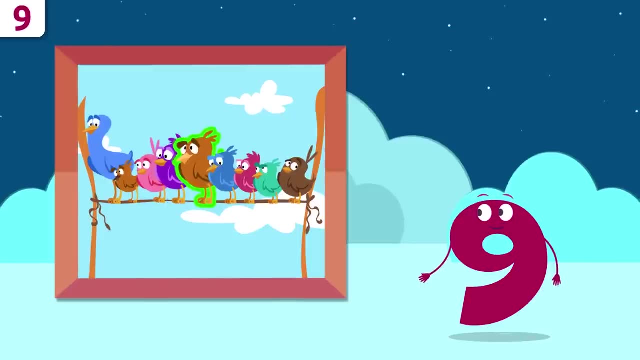 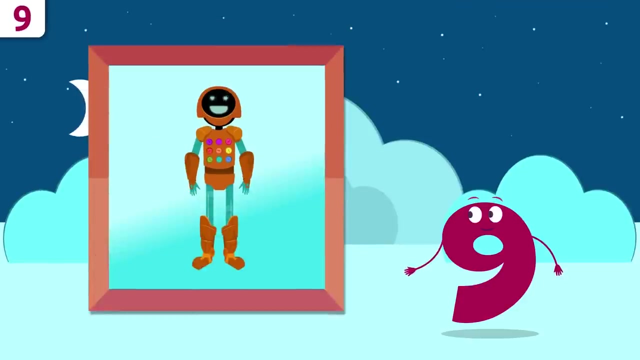 There are nine singers. There are so many birds: One, two, three, four, five, six, seven, eight and nine. There are nine birds. Hey look, It's Bot the Robot. Let me see how many buttons you have. 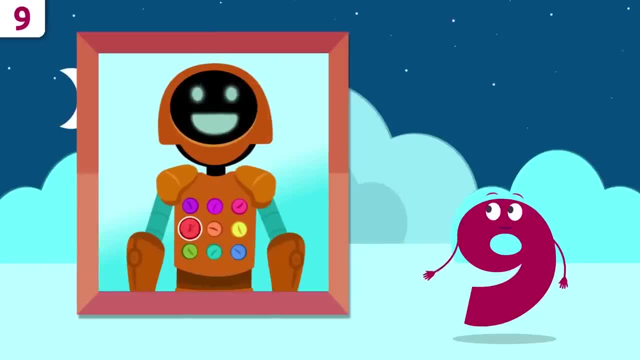 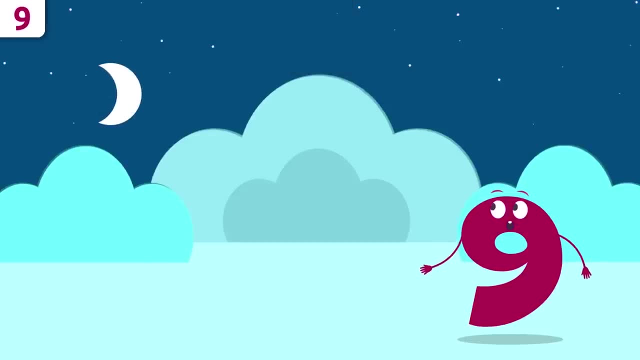 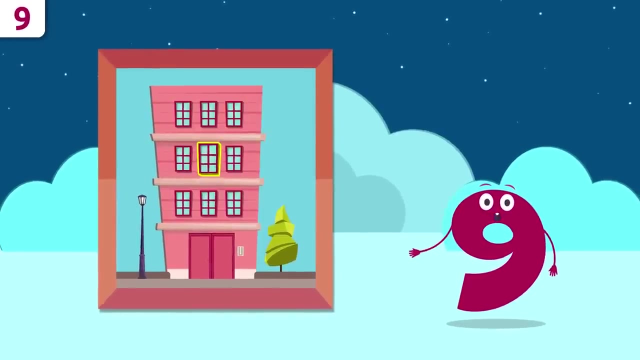 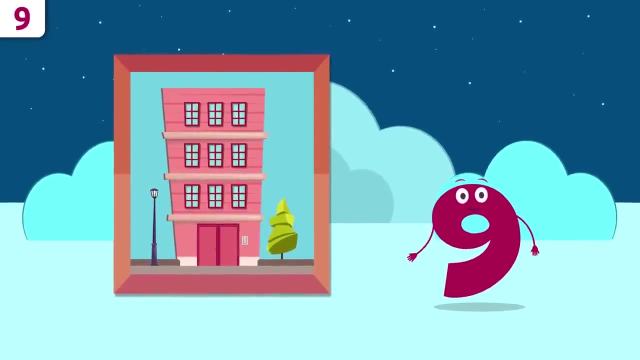 One, two, three, four, five, six, seven, eight and nine. How about this building? How many windows are there? One, two, three, four, five, six, seven, eight and nine. This building has nine windows. 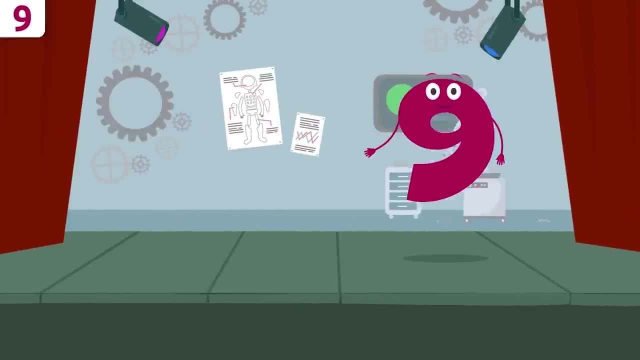 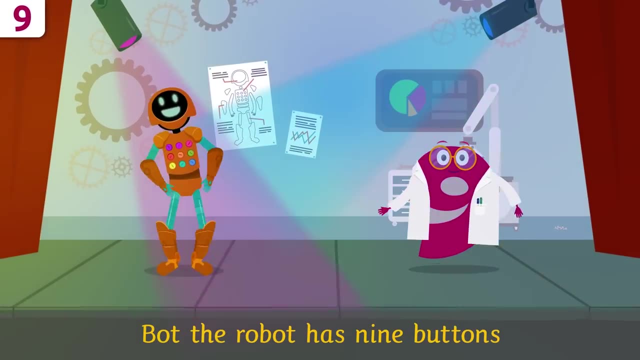 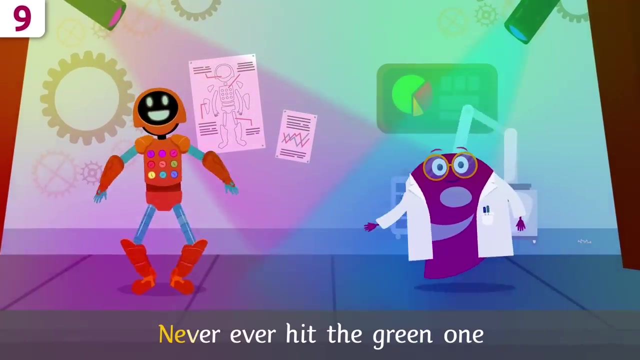 Great job, friends. Time to sing Bot. do you want to sing along, Bot? the Robot has nine buttons Pressed by nine fluffy buttons. Never, ever hit the green one. If you did, you'd have to run. Never, ever hit the green one. 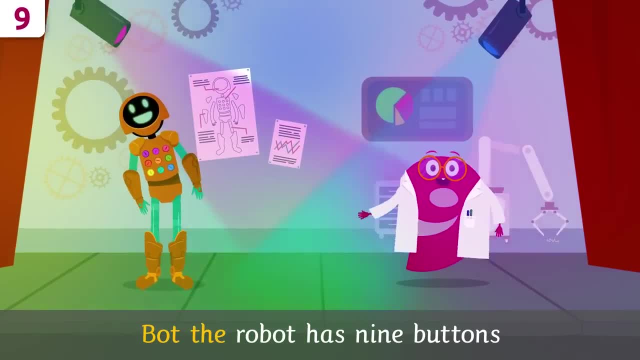 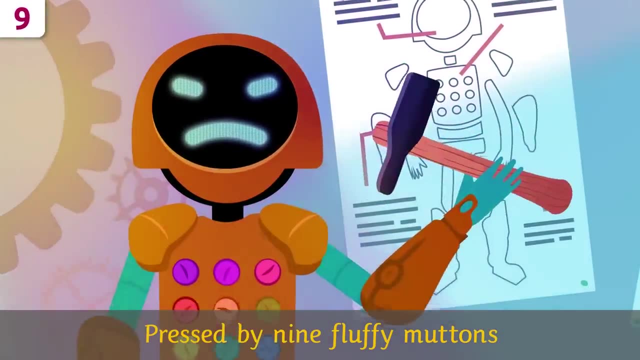 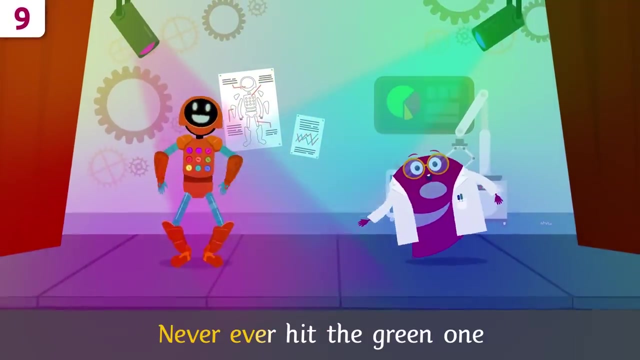 If you did, you'd have to run Bot. the Robot has nine buttons Pressed by nine fluffy buttons. Never ever hit the green one. If you did, you'd have to run. Never ever hit the green one. If you did, you'd have to run. 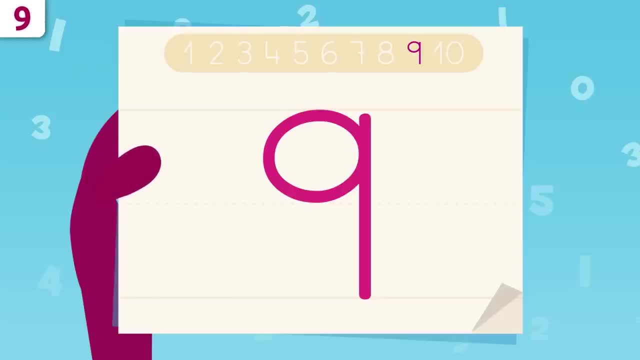 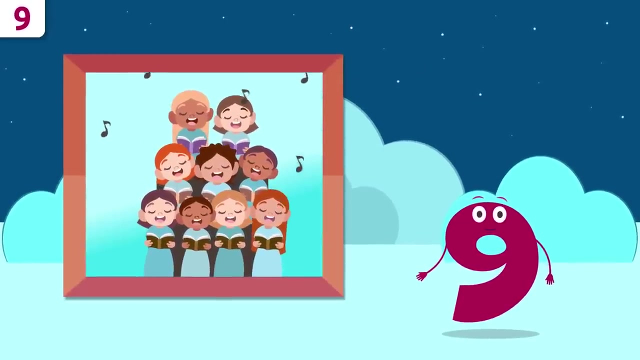 And this is number nine. Oh look, I look like a cowboy lasso. Try it at home using some paper and a pencil. Would you like to look at some examples? Whoa, It's a choir. How many singers are there? 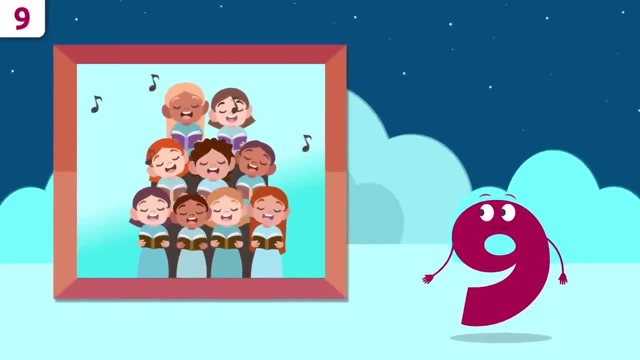 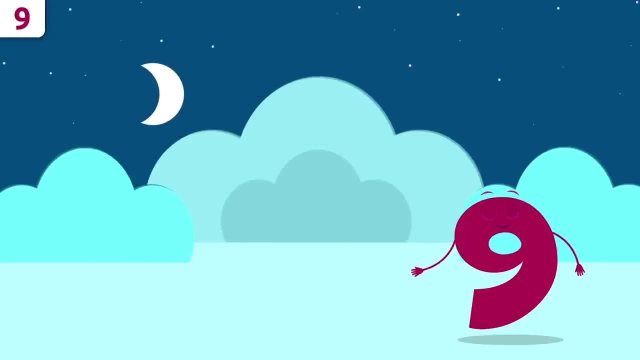 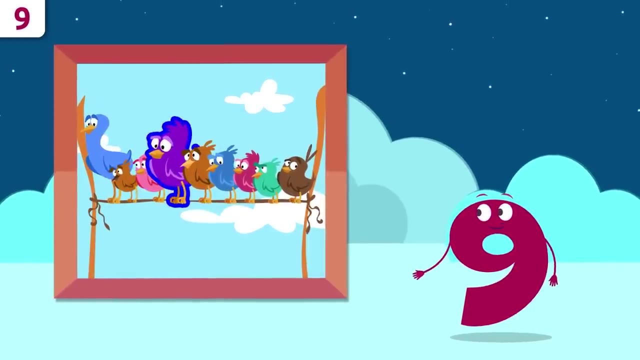 One, two, three, Four, five, six, seven, eight and nine. There are nine singers. There are so many birds: One, two, three, four, five, six, seven, eight and nine. There are nine birds. 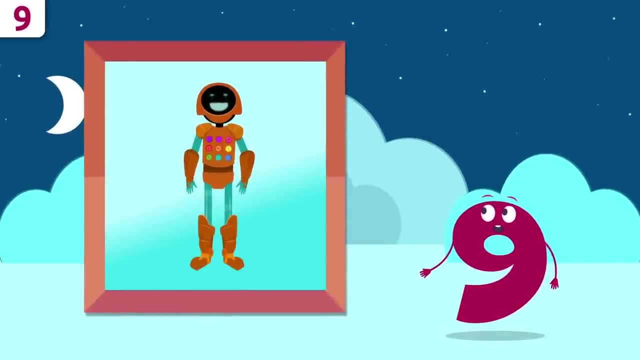 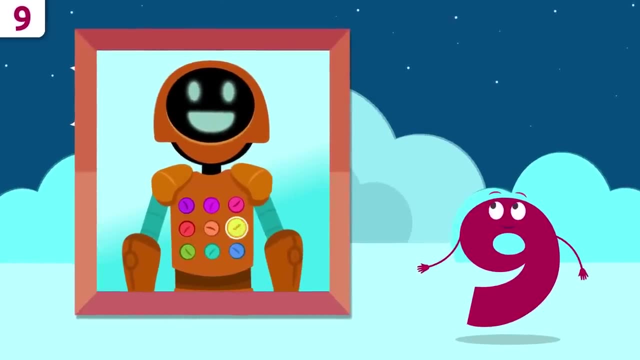 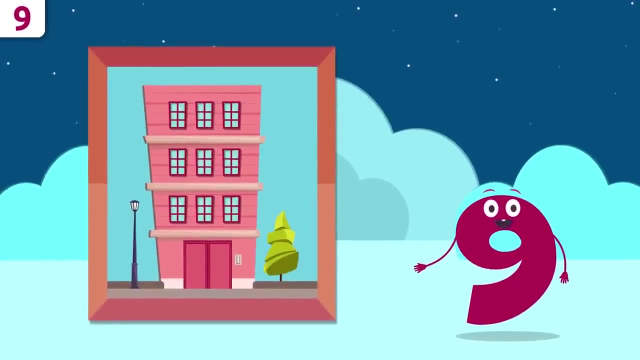 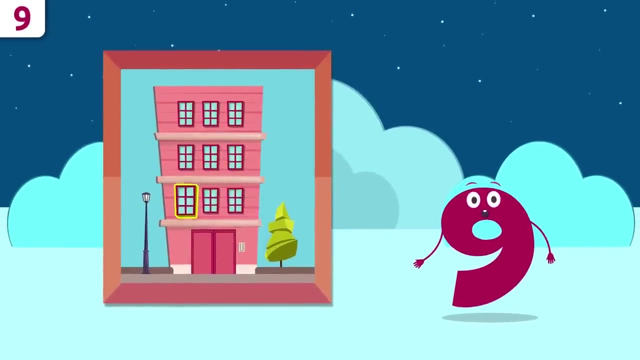 Hey look, It's Bot the Robot. Let me see how many buttons you have: One, two, three, Three, four, five, six, seven, eight and nine. How about this building? How many windows are there? One, two, three, four, five, six, seven, eight and nine. 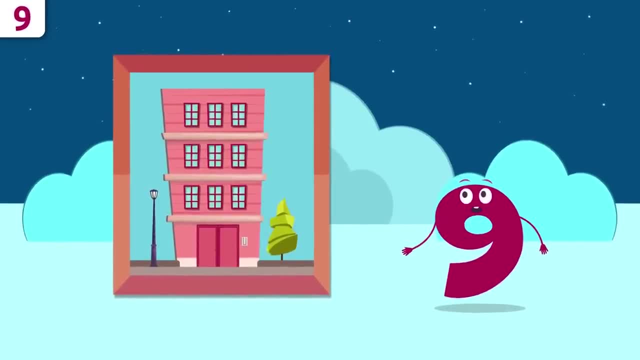 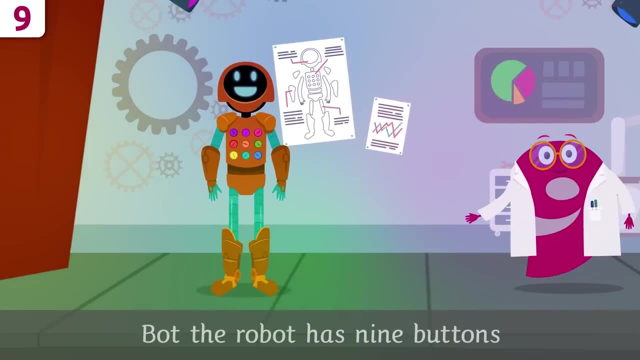 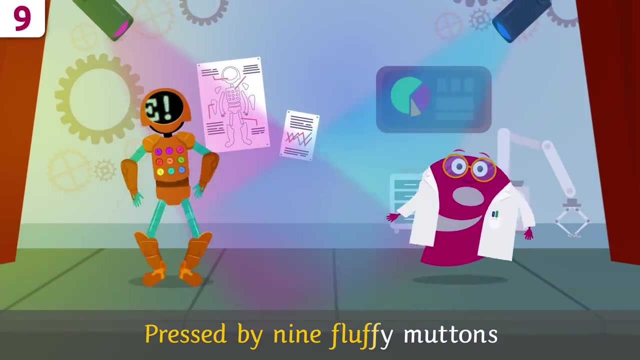 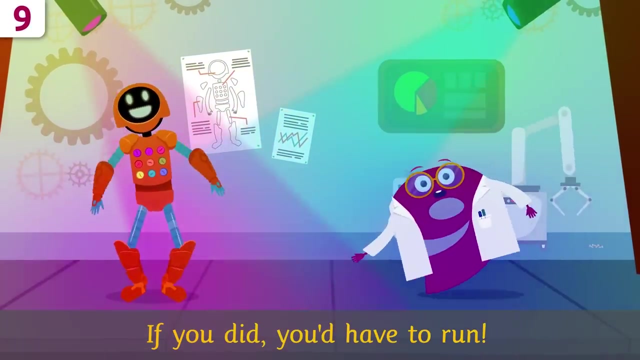 This building has nine windows. Great job, friends. Time to sing Bot. do you want to sing along Bot? the robot has nine buttons. Press behind nine fluffy buttons. Never, ever, hit the green one. If you did, you have to run. 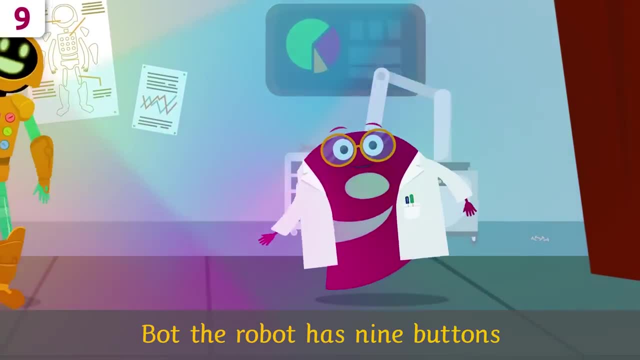 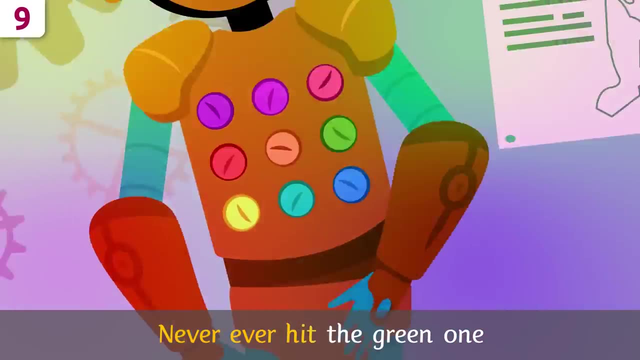 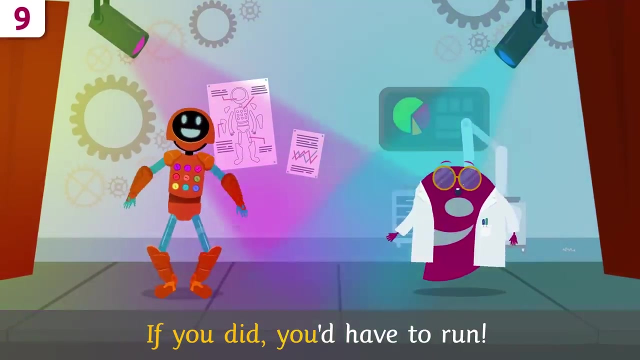 Bot. the robot has nine buttons. Press behind nine fluffy buttons. Never, ever, hit the green one. If you did, you have to run Green one. if you did, you'd have to run. Never, ever hit the green one. if you did, you'd have to run. 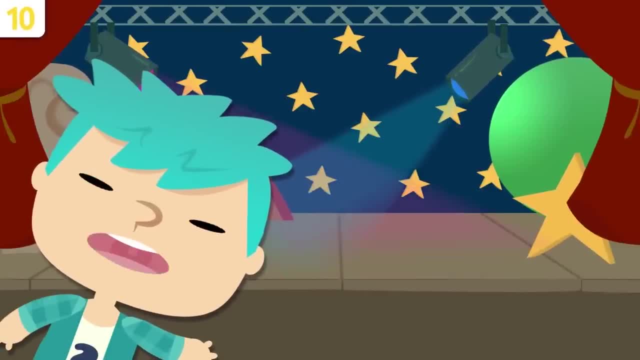 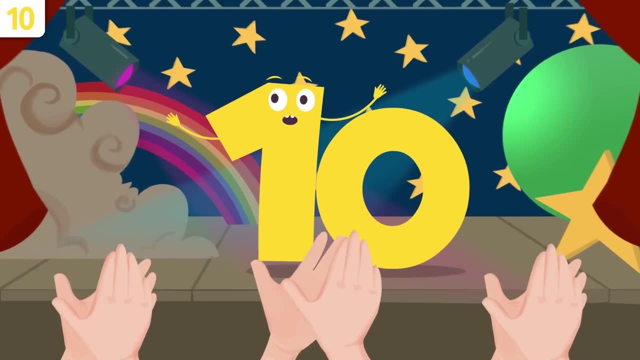 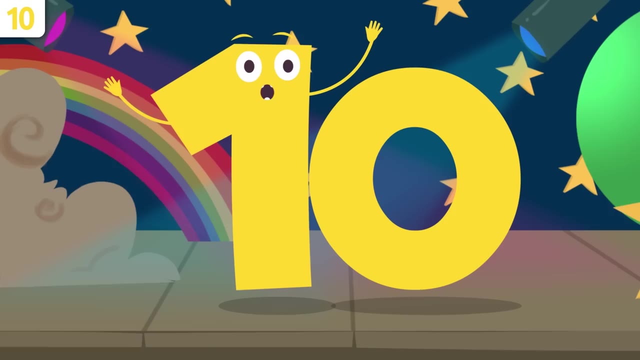 Here we are again, friends of numbers, introducing number 10.. That's right, I'm number 10.. And today I'll be telling you a few things about me. Remember, we'll be singing a song at the end of the video. you can't miss it. 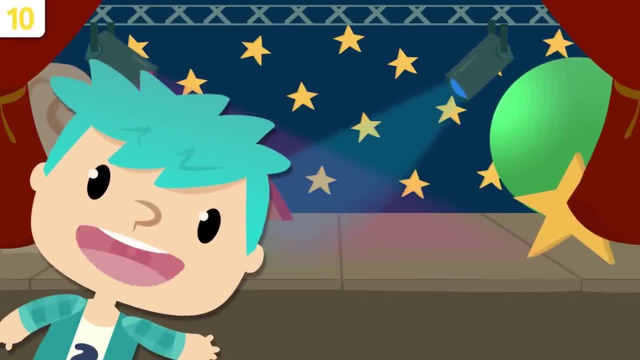 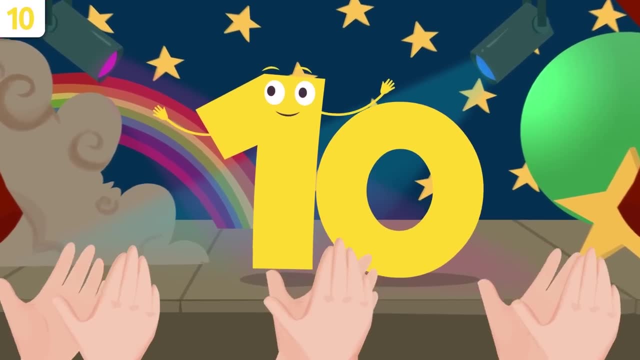 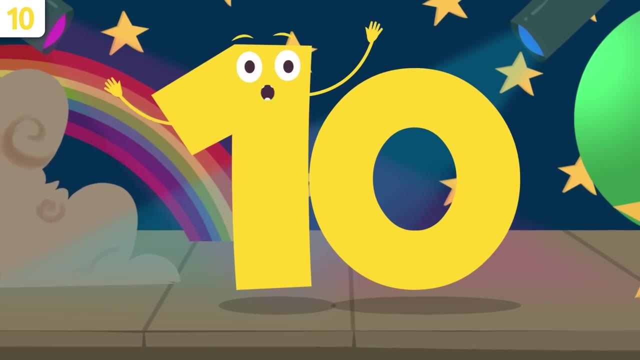 Here we are again, friends of numbers, Introducing number ten. That's right, I'm number ten, And today I'll be telling you a few things about me. Remember, we'll be singing a song at the end of the video. You can't miss it. 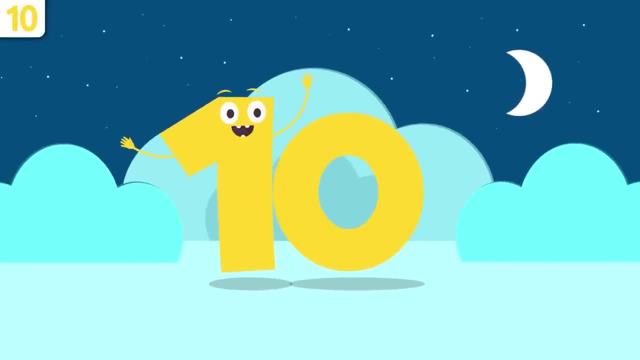 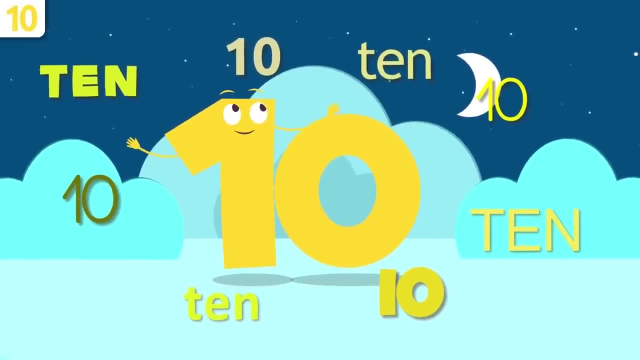 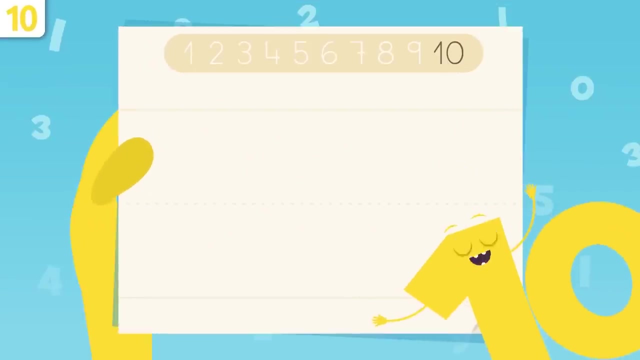 The first thing we'll do is say my name, Repeat after me Ten, Ten, Louder Ten, Yeah. Now I'm going to show you how to write number ten. Number ten is made up of two numbers: One and zero. Let's begin with number one. 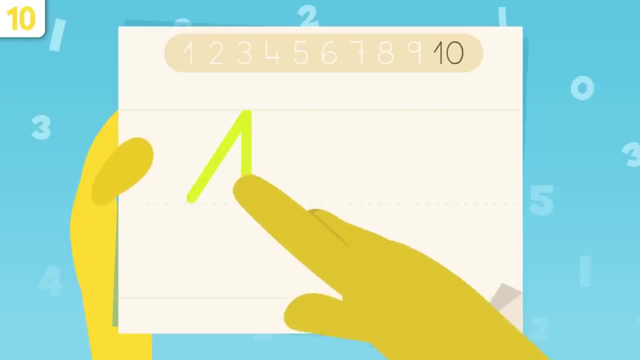 We're going to start right here and go all the way up. Then we'll trace a vertical line. That's number one. Let's try tracing zero. We're going to start right here and draw a curve, Then we'll close the curve, tracing it all the way up. 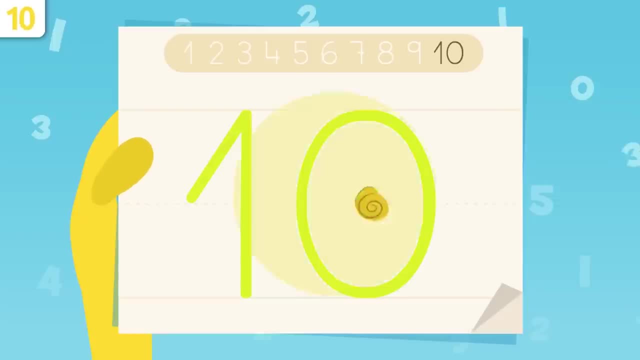 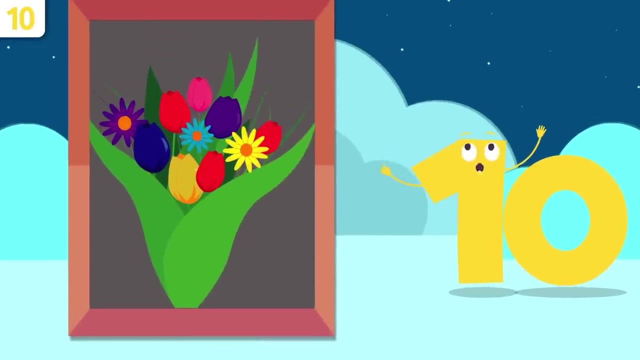 That's it. This is number ten. Oh look, I look like a snail. Try it at home using some paper and a pencil. It's easy peasy. How about looking at some examples? Whoa, look Flowers, So pretty. 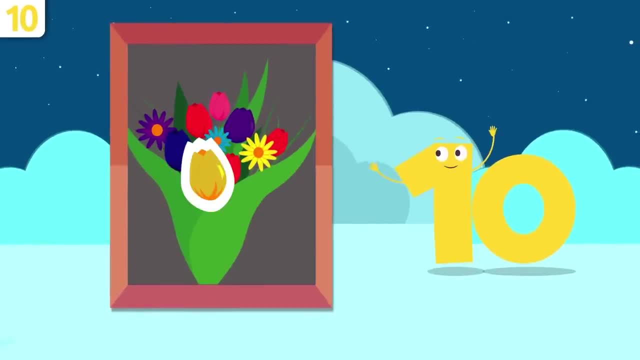 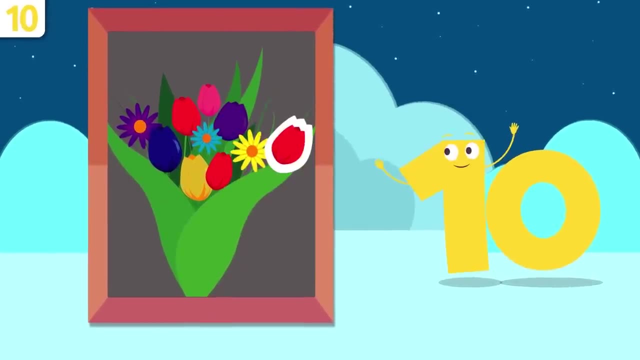 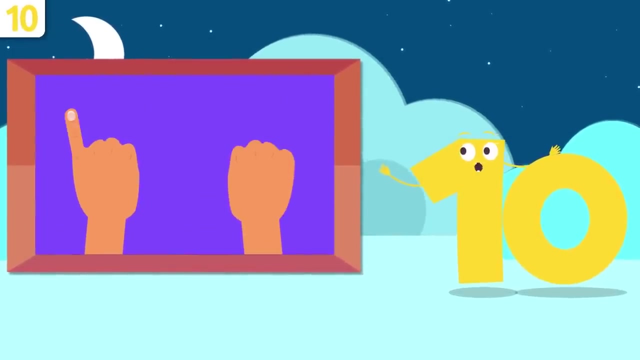 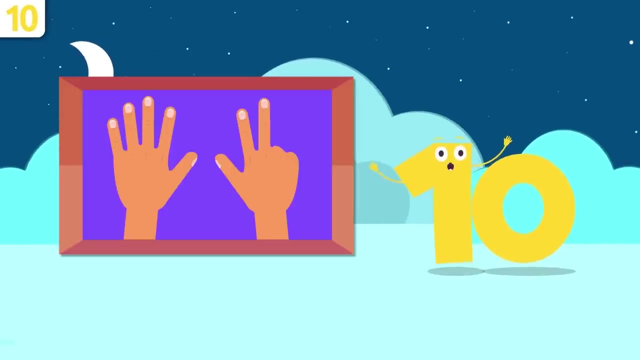 How many are there? One, Two, Three, Four, Five, Six, Seven, Eight, Nine And ten? There are ten flowers. How many fingers are there on both hands? Let's count: One, Two, Three, Four, Five, Six, Seven, Eight, Nine And ten. There are ten fingers on both hands. 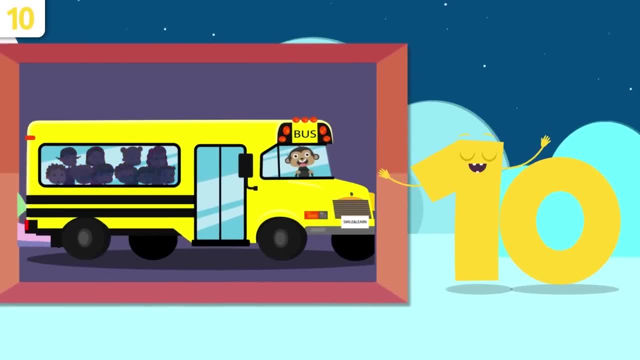 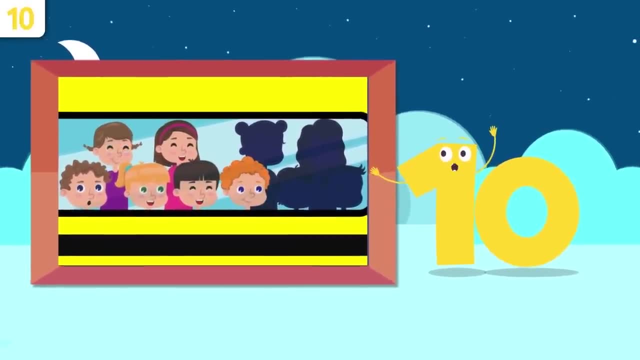 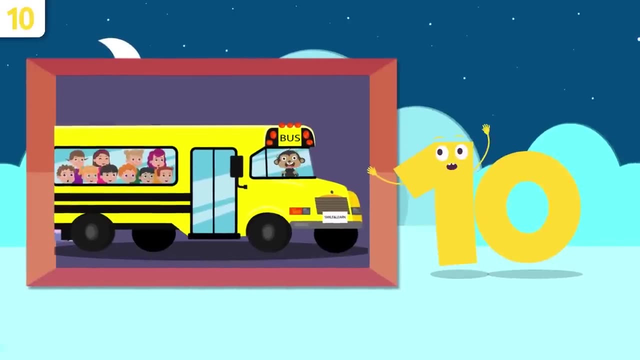 And how many children are there on this school bus? Let's see One, Two, Three, Four, Five, Six, Seven, Eight, Nine, Ten. There are ten children on the school bus. Hey, do you want to sing later? And how many boxes do we have here? 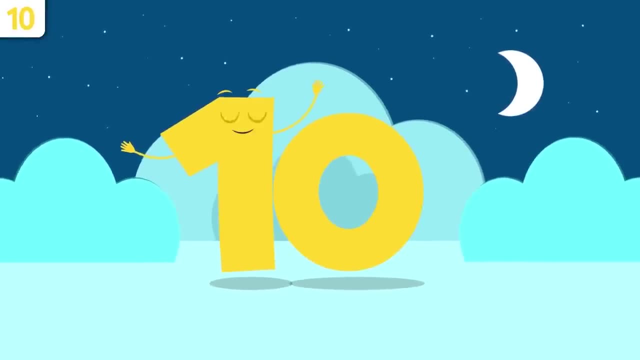 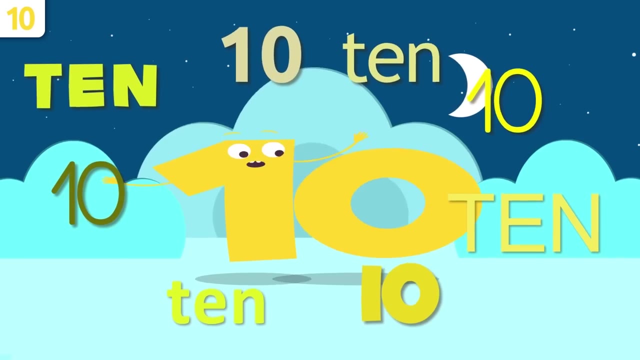 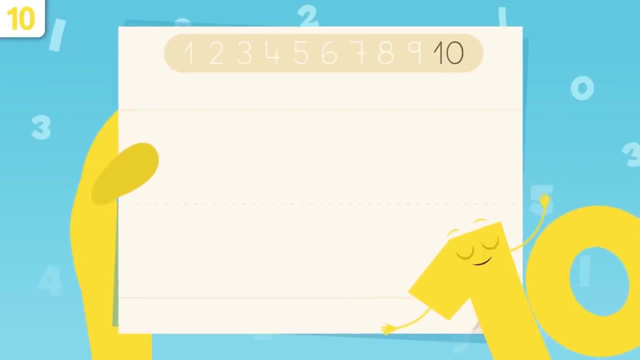 The first thing we'll do is say my name, Repeat after me: 10,, 10,, louder, 10.. Now I'm going to show you how to write number 10.. Number 10 is made up of two numbers: 1 and 0.. 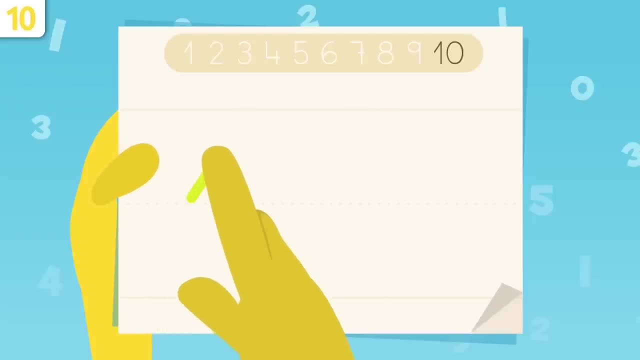 Let's begin. Let's begin with number 1.. We're going to start right here and go all the way up. Then we'll trace a vertical line. That's number 1.. Let's try tracing 0.. We're going to start right here and draw a curve. 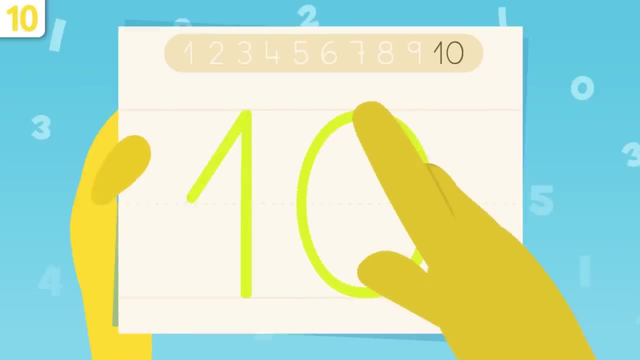 Then we'll close the curve, tracing it all the way up. That's it. This is number 10.. Oh look, I look like a snail. Try it at home using some paper and a pencil. It's easy peasy. 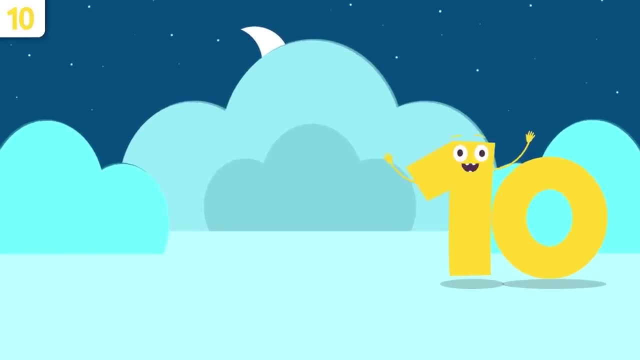 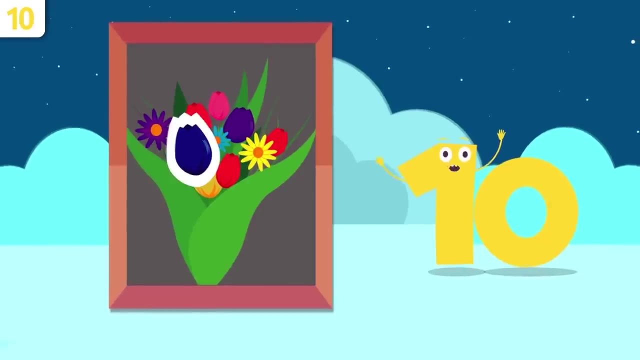 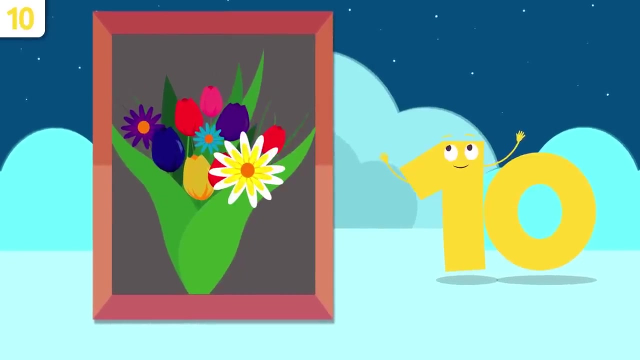 How about looking at some examples? Whoa, look flowers So pretty. How many are there? 1,, 2,, 3,, 4,, 5,, 6,, 7,, 8,, 9, and 10.. 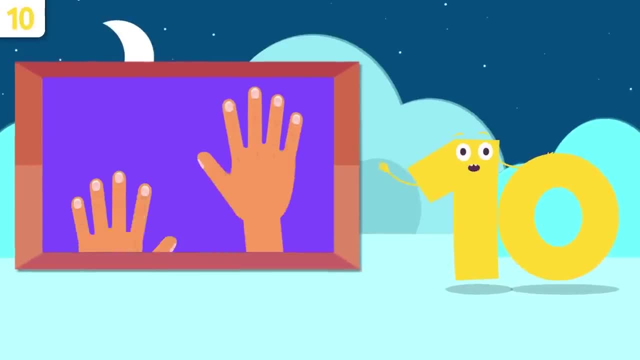 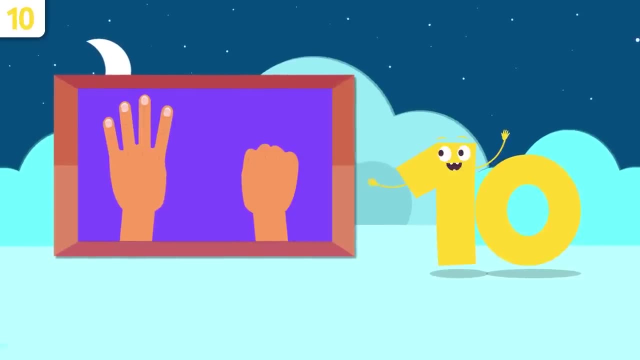 There are 10 flowers. How many fingers are there on both hands? Let's count 1,, 2,, 3,, 4,, 5,, 6.. 7,, 8,, 9, and 10.. There are 10 fingers on both hands. 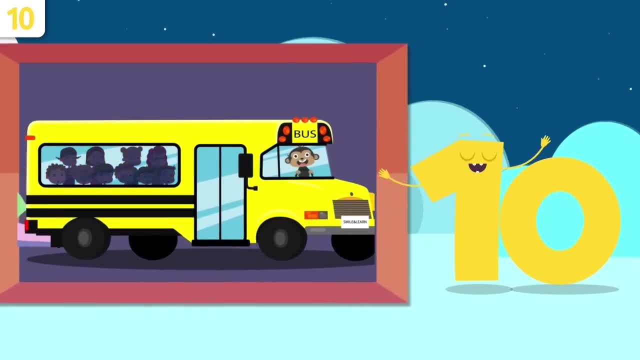 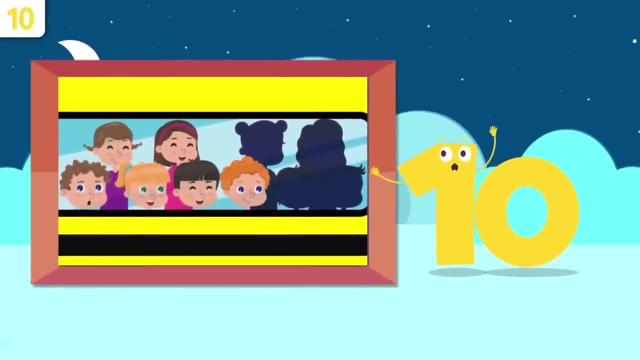 And how many children are there on this school bus. Let's see 1,, 2,, 3,, 4,, 5,, 6,, 7,, 8,, 9, and 10.. There are 10 children on the school bus. 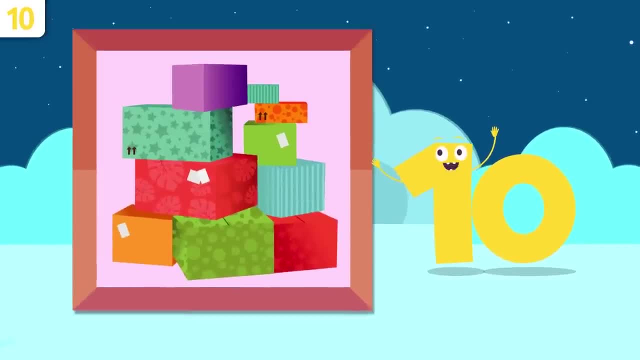 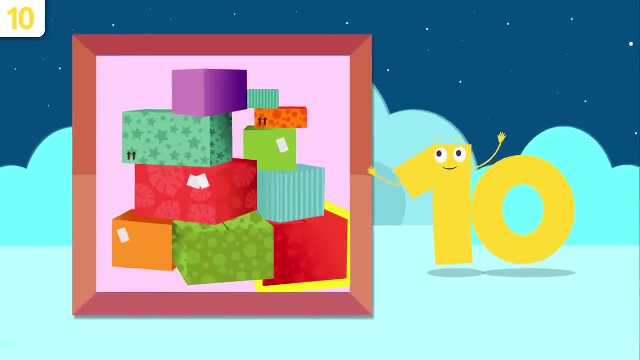 Hey, do you want to sing later? And how many boxes do we have here? 1., 2,, 3,, 4,, 5,, 6,, 7,, 8,, 9, and 10.. There are 10 boxes. 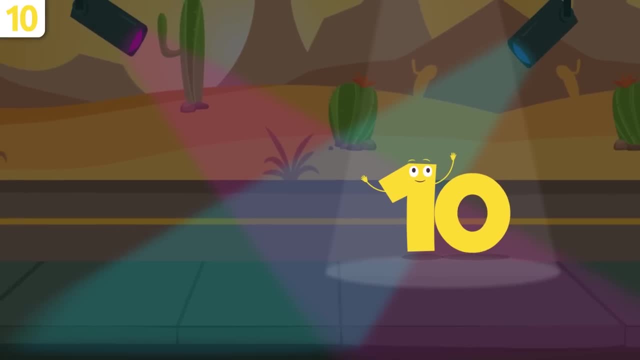 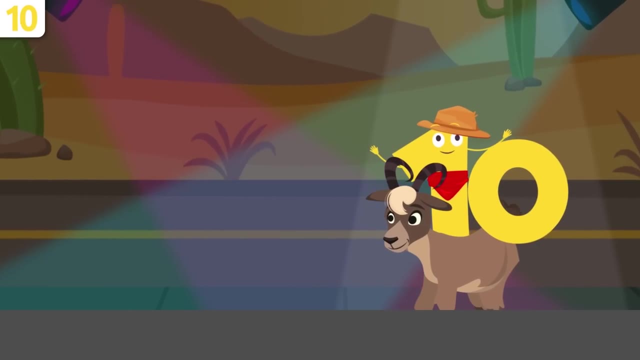 Awesome, Sing along everyone: 1,, 2,, 3,, 4,, 5,, 6,, 7,, 8,, 9, and 10.. And kids go on a field trip with a wild monkey. So hip, nobody can leave their eyes.